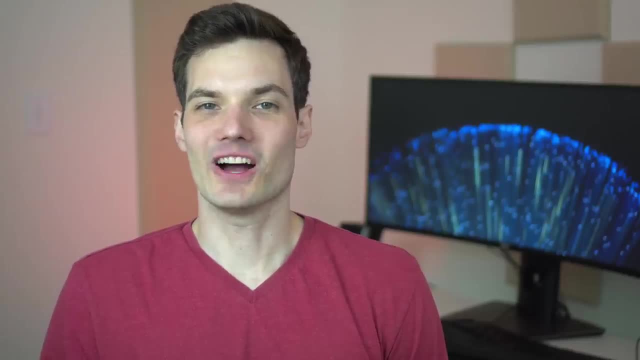 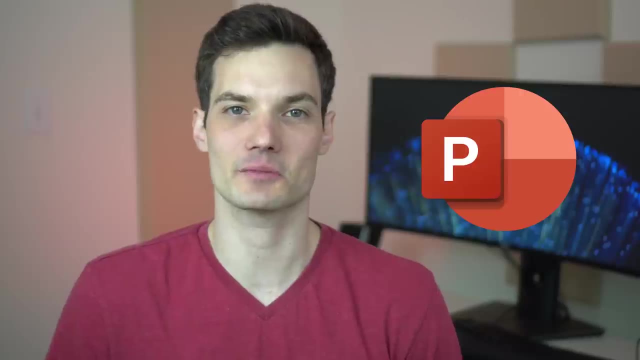 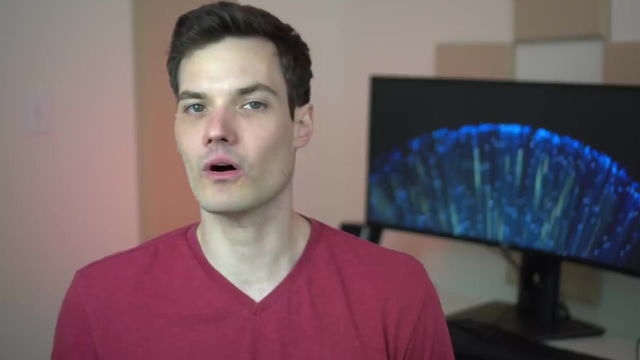 Hey everyone, Kevin, here Today I want to show you the fundamentals of animation in Microsoft PowerPoint. We're going to start off with the basics of how you create just a very simple animation. We'll also run through all of the different animation tools that you have. 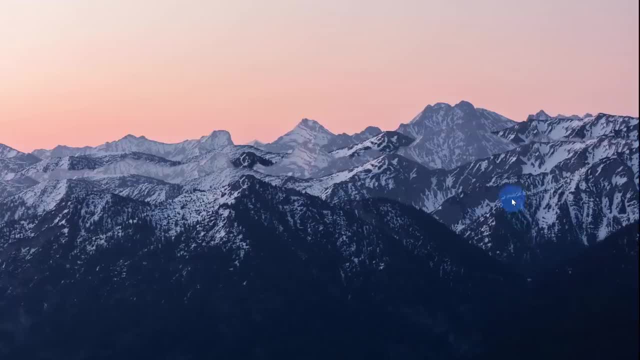 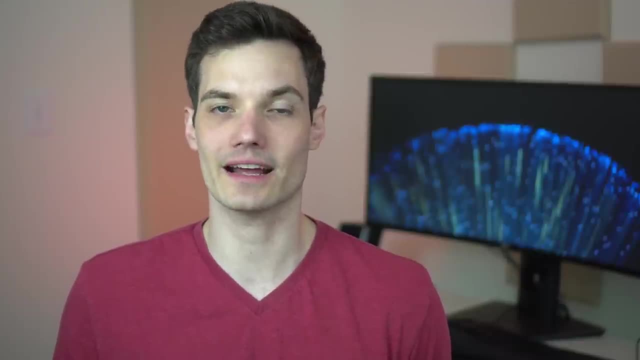 available to you. Once we look at the basics, then we'll go a little bit more advanced and we'll create a more complex animation that involves different layers. Once we run through that, I also want to show you how you can create a morph and also an advanced morph transition. 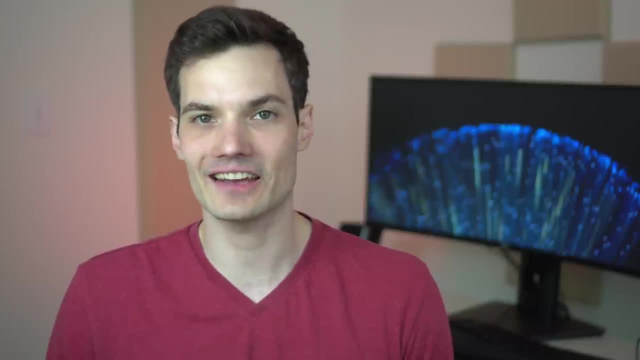 which is also a form of an animation. Then, at the very end, we're also going to look at how you can animate 3D objects. By the end of this video, you should know all of the essentials of how to animate in PowerPoint, All right? well, let's jump on the PC and let's start animating. Here I am. 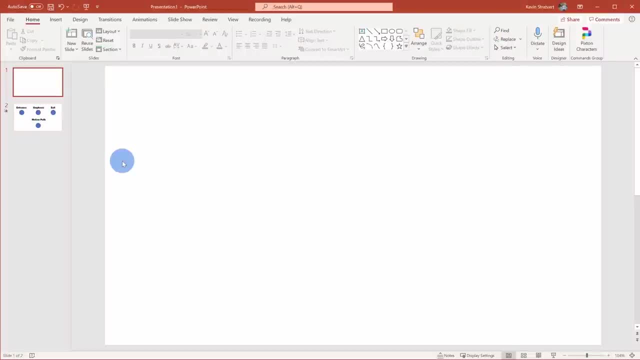 now on my PC, and I already have my PC. I'm going to go ahead and start animating. I'm going to Microsoft PowerPoint open. If you want to follow along with this tutorial today, I'll go at a pretty good pace so you can follow along as well. First off, open up PowerPoint and jump into a 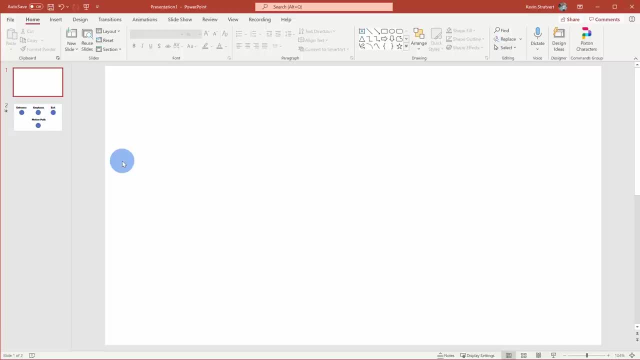 blank new presentation. We don't need anything in place. We'll be able to just start with blank and we'll create everything that we need as we go through this step by step. Once you land in your new presentation, right now it's just blank and we want to start animating. To animate, we need some. 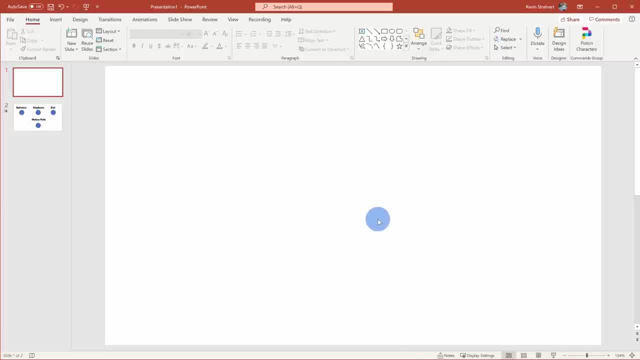 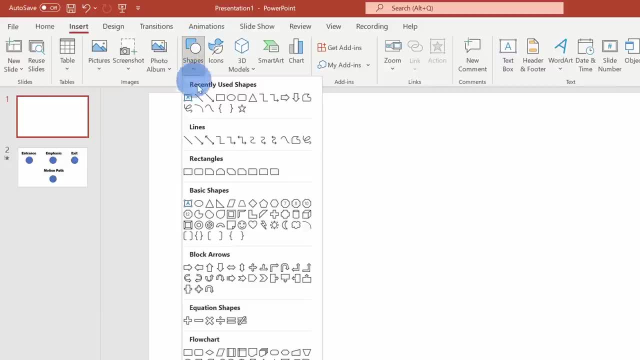 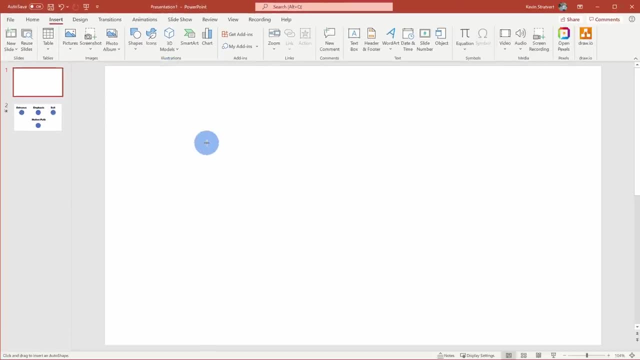 start off really basic today And let's just click on shapes and I'll use an oval right here and I'll insert this on my slide. You can use any type of shape, but I'm just going to start with this one. I'll click on this and now I'm going to draw an oval on my slide Just as a quick little tip. if 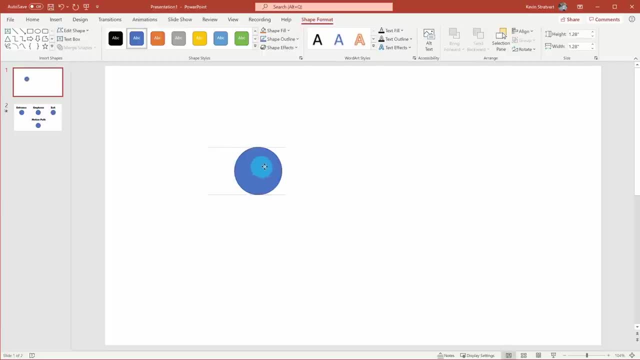 you want a perfect circle, you could press the shift key and this will give you a nice circle, And I'll just position that right here on my slide. So we have our first shape and now we want to start animating. So I'm going to go ahead and start animating. So I'm going to go ahead and 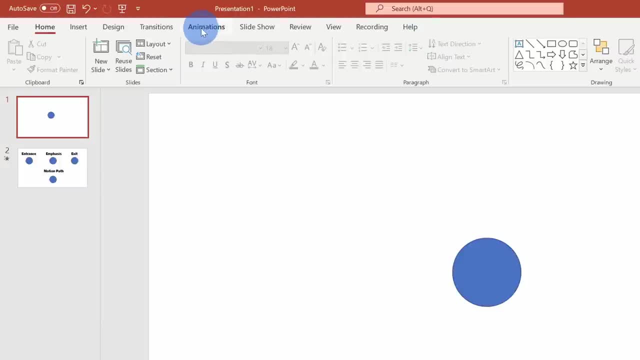 start animating. So, to animate, let's go to the top ribbon and there's an option here called animations. Let's click on this. This opens up the animation ribbon and you'll see here that there are all these different tools available to animate this scene or this object. Now, right now. 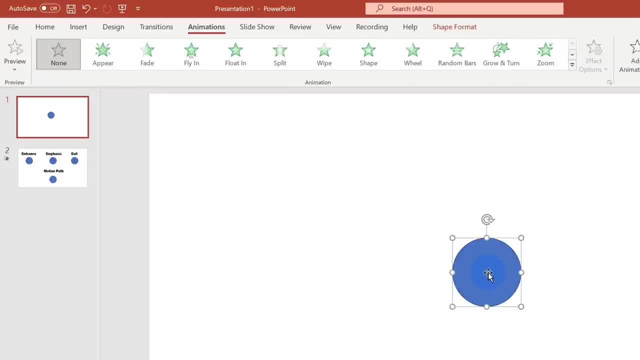 everything is grayed out. To highlight this, let's go down and click on the shape that you just inserted. Once you click on it, you'll see all of these different animation options light up. First, let's start over on the left-hand side, where you have this section called animation. 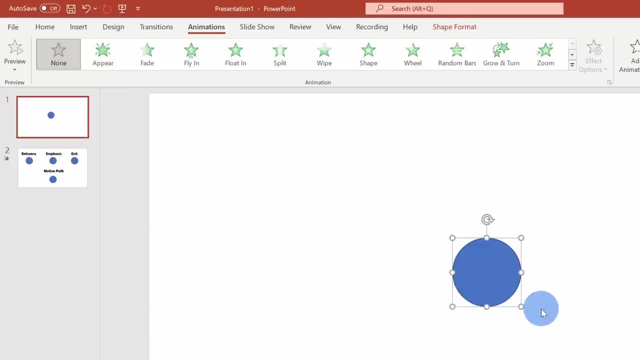 You'll see a few different types of animation that you can apply to this object. Right here you can scroll through all of the different options. but an easier way to get an overview of all of the different options or all the different animations that you have available to you, go down and click on this arrow on the bottom. 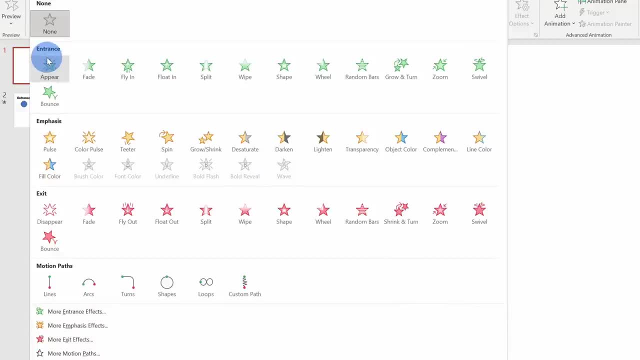 and this exposes the entire set. So right here we see a number of different categories of animations that we have available. Right now, we don't have any animation on our object, so it's currently set to none. You can always use this to remove any animations in the future. Right here: 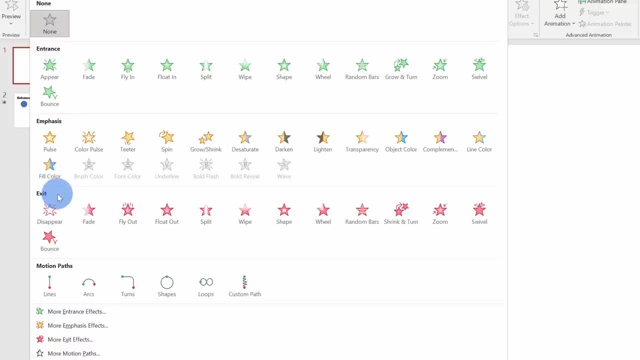 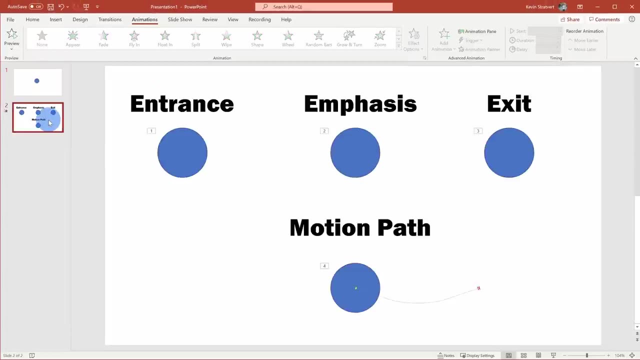 you have entrance animations, you have emphasis animations, exit and also motion paths. Now, the easiest way to understand what these are. I'm going to jump to another slide and I'll just show a quick example of what these are. I'm in presentation mode right now and let's start. 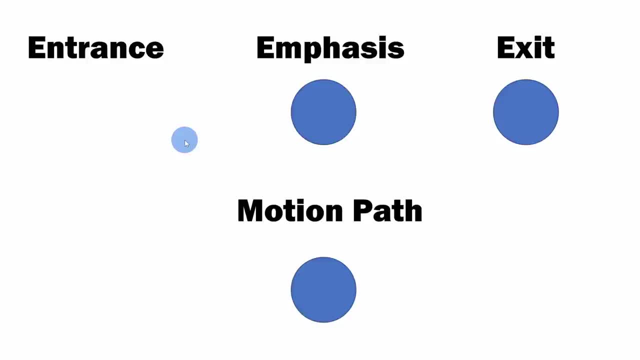 off with entrance. Entrance means that the shape is not yet visible, but when, let's say, I hit my mouse, it'll animate the shape in. You also have another category of animations, called emphasis, and here, when I click, you'll see that it just emphasizes the shape. The shape's already visible. 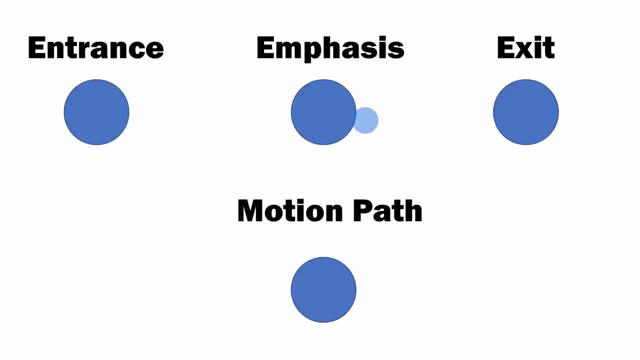 on the slide and it'll stay on the slide forever. So I'm going to click on this and I'm going to click on the slide. It simply emphasizes it. You have another category of animations called exit. So here you see the shape, and when I do the animation it'll exit out of the scene And then 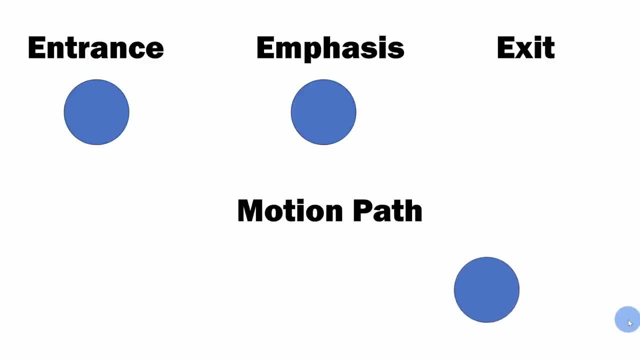 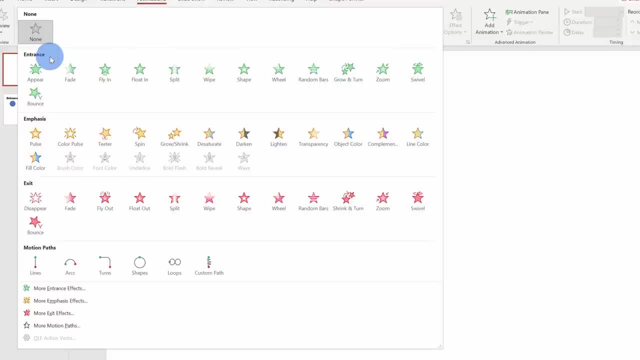 the last category is motion path. Well, here you can set up a path that the object will follow. Now that we've looked at what all of these different categories are, let's apply our first animation to this shape. To apply an animation, I can simply click on one of these and then that'll. 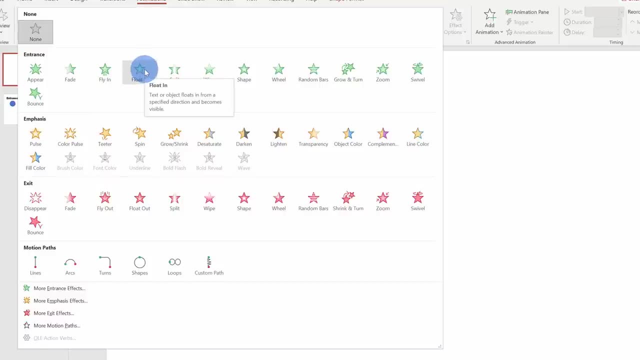 animate it. So here, for example, maybe I want it to float in- Let's click on the float in option. Right there you can see that the animation has been animated. So let's click on the float in option. 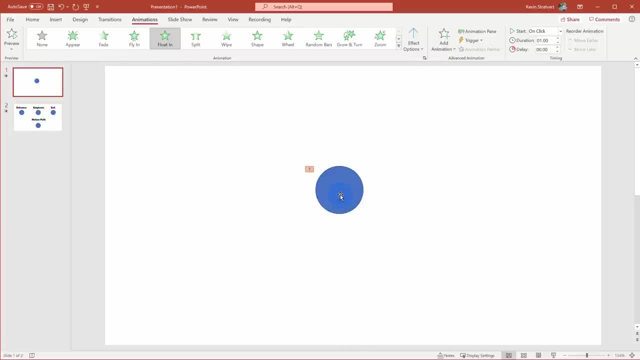 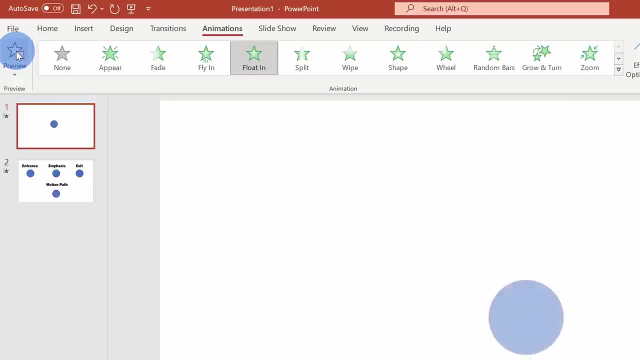 Right there you'll see a preview of the animation. If I want to preview the animation again, up on the top ribbon once again under animations over on the left-hand side, I have this button called preview. When I click on this once again I can preview what the animation looks. 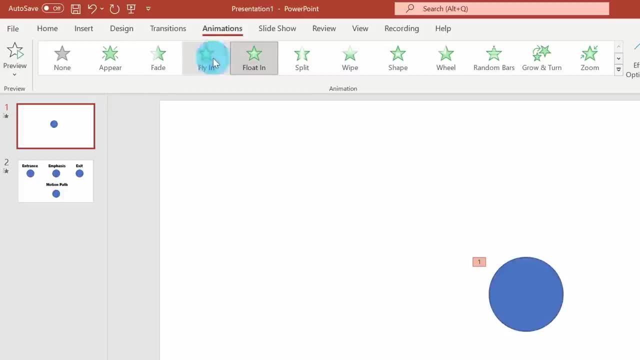 like And you notice too, once I applied an animation. so let's say I click on fly in Here, it'll preview the animation when I select it up here Over on the left-hand side. if I click on this dropdown I can turn on or off auto preview. I like leaving it on That way. 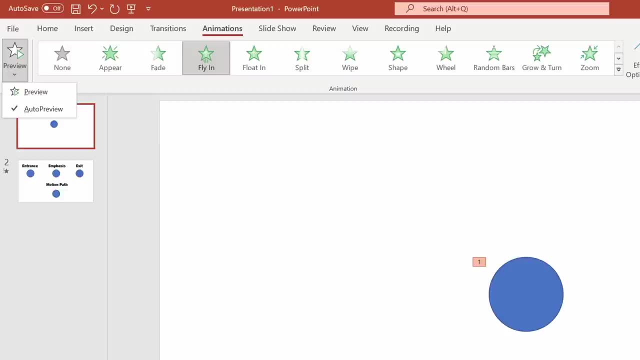 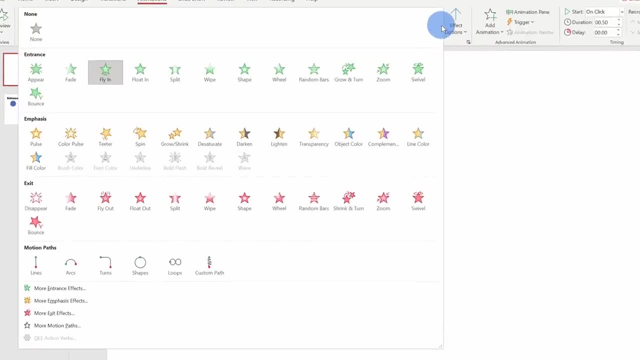 when you select an animation, you can quickly see what it looks like on your slide. We've now applied our first animation to a shape and we know how to preview it. And if I go right back up here and I look at all the animations, 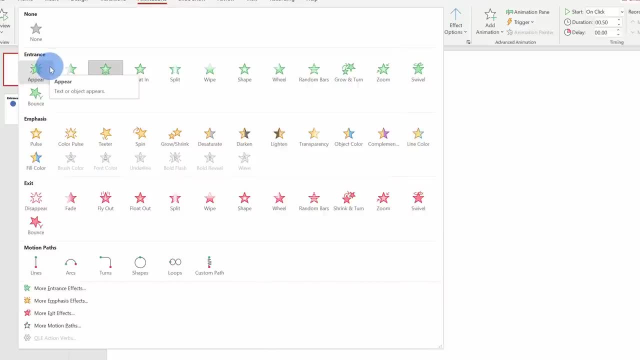 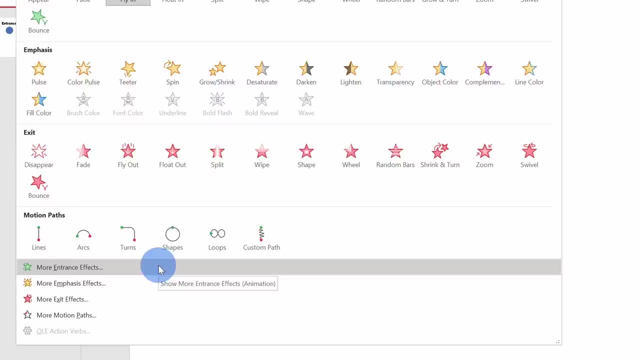 it looks like you have a bunch of different options, But you know, once you start playing with it, you might feel that you don't have enough right here. If we look at the very bottom, here you have access to even more effects, So you could get even more entrance, emphasis, exit. 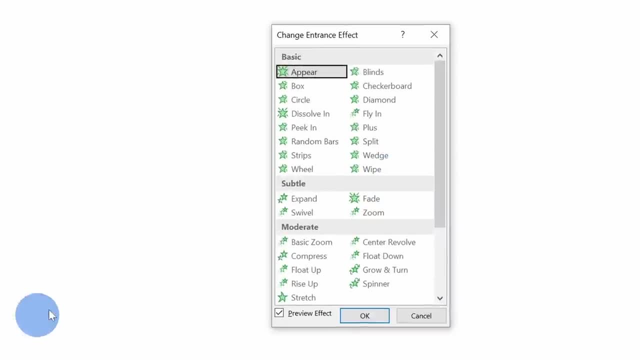 or motion path effects. So here I'll click on more entrance effects, and this opens up a prompt where you can see if you want to preview the animation. you can preview the animation and you can see a very broad collection of different effects. So right here, maybe I want. 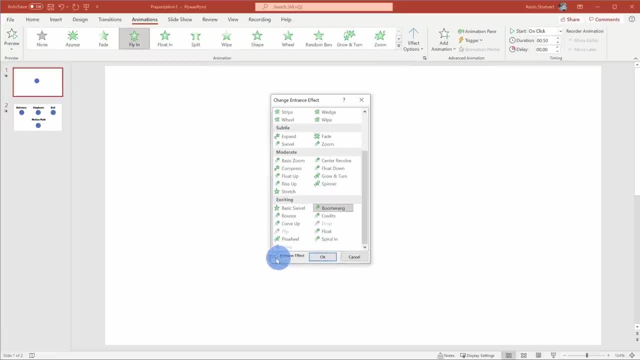 to go with boomerang. I'll select this one and then click on okay. Once again, it's set to preview the effect once I select it. So right here, you can see it now and let's preview this animation. 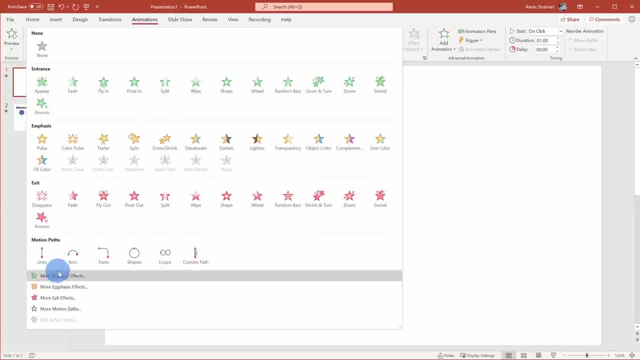 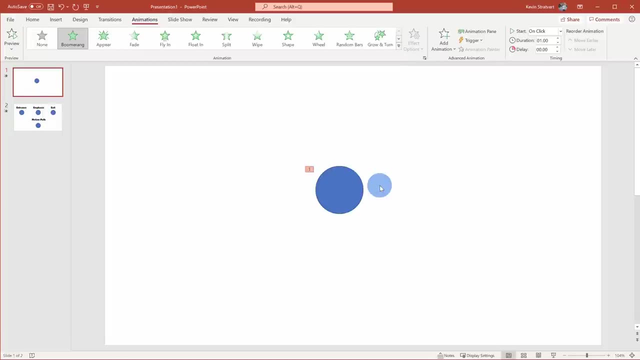 So this is one of the animations that's not part of the default set, but you can access it down here. So it's easy to miss this, but there are a lot more animations that you can choose from, So I now set this boomerang effect If I go back up to my animations, if I click on any one of these. 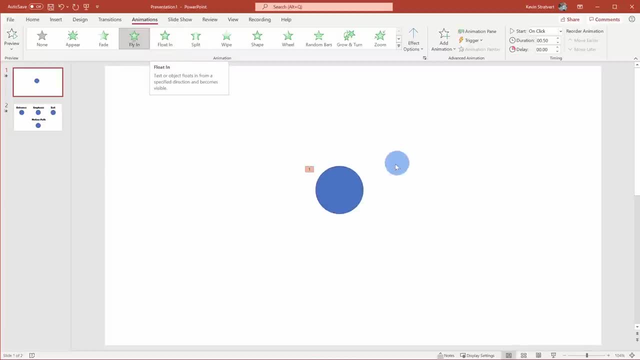 so let's say that I go with the animation. I can see that I have a lot of animations that I can go with fly in. When I click on this, this overwrites the animation that I already had selected. So here, if I click on zoom, it'll overwrite the fly in. Here, if I click on fly in. 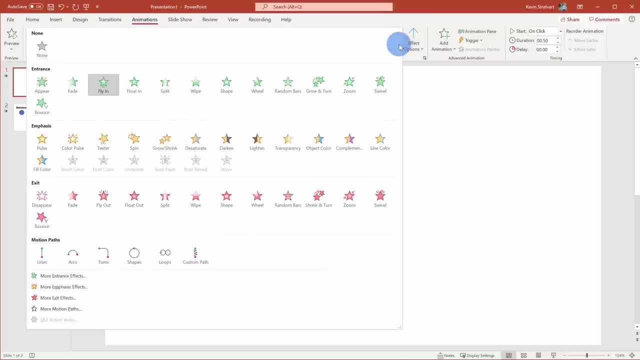 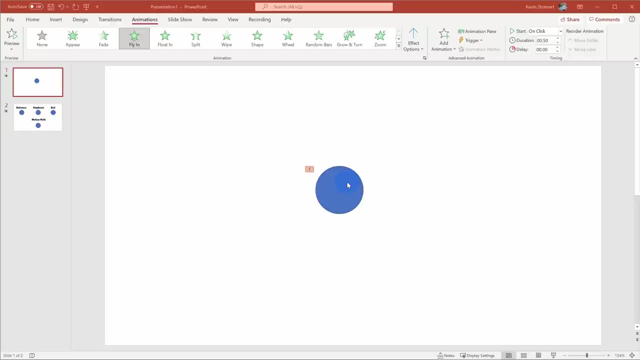 that'll overwrite the zoom. So anytime you click on an animation over here, it'll overwrite any preexisting animation that you have set to an object. I've now set the fly in animation to this shape and if we look up on top on the ribbon, once again right to the right of all of my 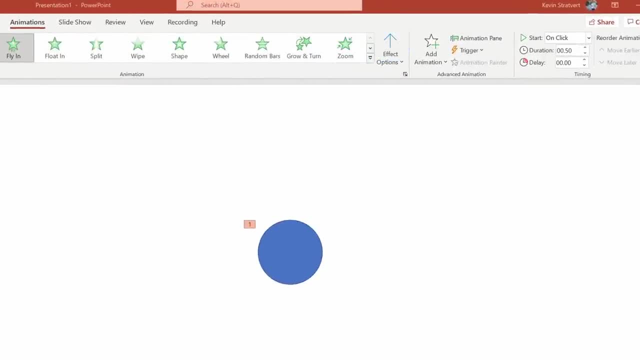 different animations. there's something called effect options. If I go back to my animation, I can see that I've set the object to what I want to call the object and I can also set the. Now you'll notice, when I play this animation it comes in from the bottom or it flies in. 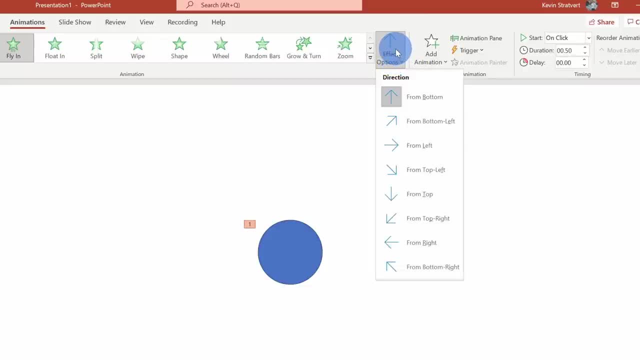 from the bottom. If I click over on effect options, I can alter the direction that this shape comes in from. So maybe I want it to come from the left. I could have it come in from there. I could have it come in from the right. 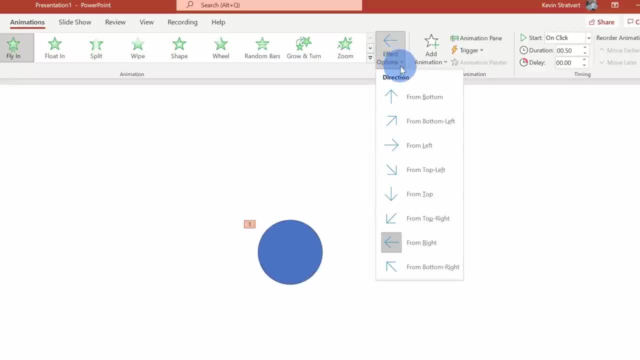 So it gives me some control over what this animation looks like. Later on in this tutorial, I'll show you even more ways you can gain even more control over what these animations are. If I click on these different shapes, you'll notice that some of them have different effect. 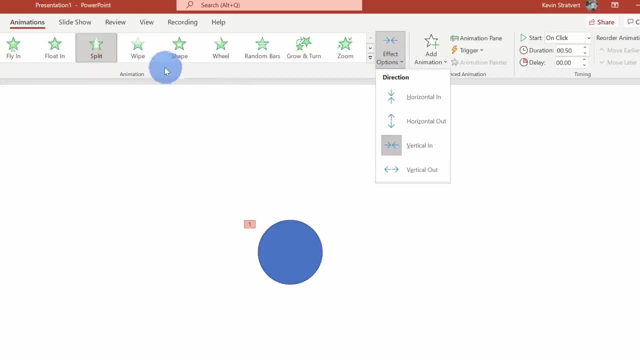 options. So here for split, you could have it split in or split out, And some of them won't have any effect options at all. But here you'll notice as I'm clicking through, most of them do, but some of them don't. 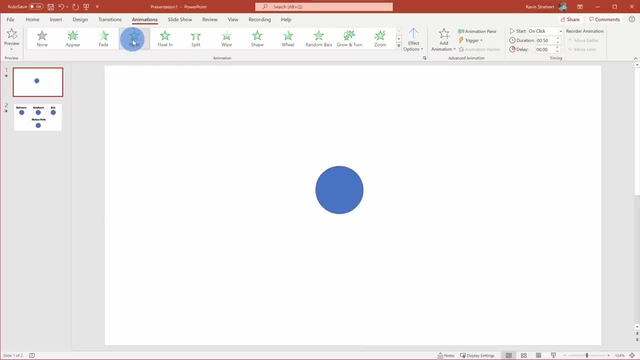 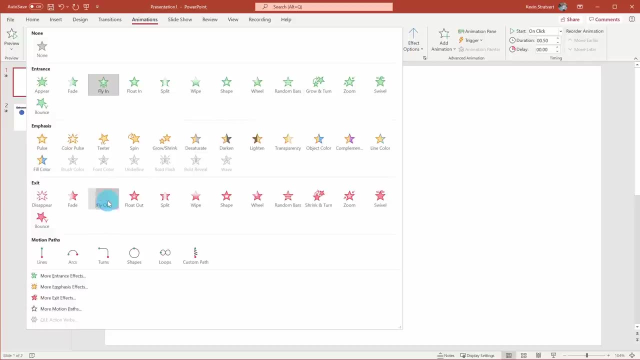 I'm going to go back now and select the fly in animation And let's say that I want the shape to fly in, but then I want it to also fly out. Now I could click on here and let's say: I go with fly out. 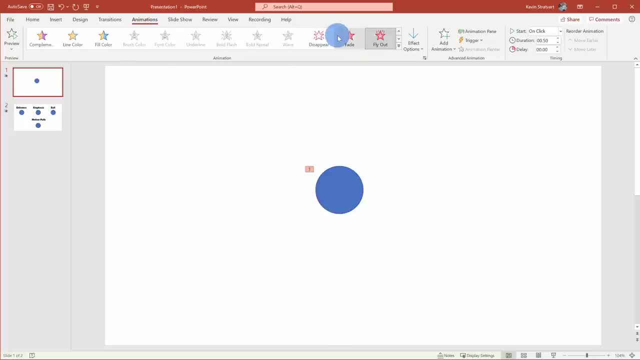 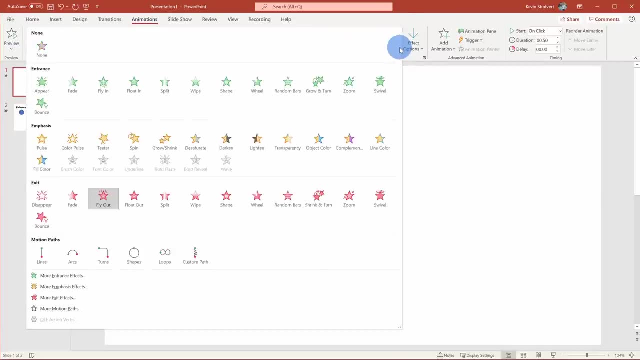 Now, just like I said before, when you select an animation in here it overwrites whatever animation you had in place. So here, if I preview it, it just flies out now and it no longer flies in. Let me go back and I'll select the fly in entrance animation and I'll set that. 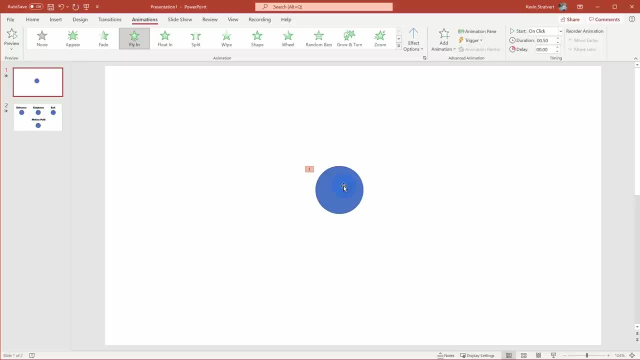 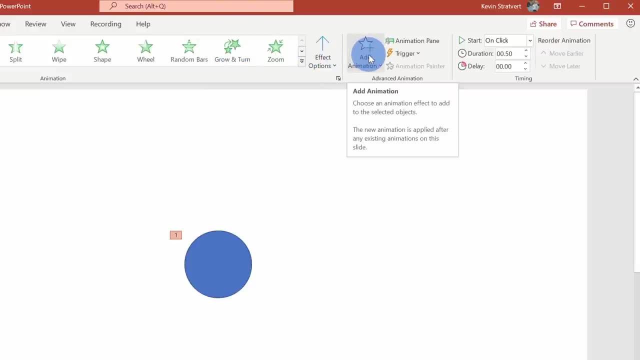 I like the fly in, but now I want to add an additional animation to this. So right up again on the ribbon if we work our way over to the right. another option here is called add animation. When I click on this, this once again shows me all of the different animations that are. 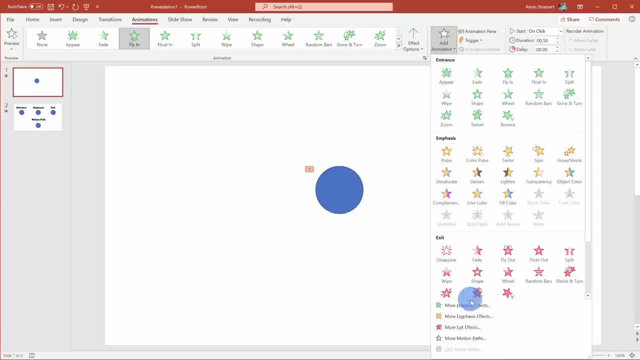 available to me. So here I see all those same categories again, And once again I can access the overflow over here in these different options down here. Now I already have the fly in animation, but I also want it to fly out, So I'll select fly out right down here. 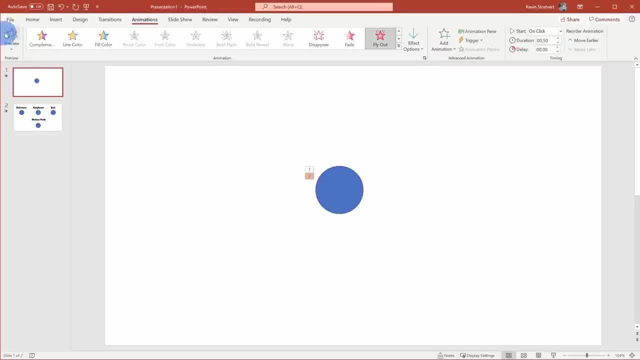 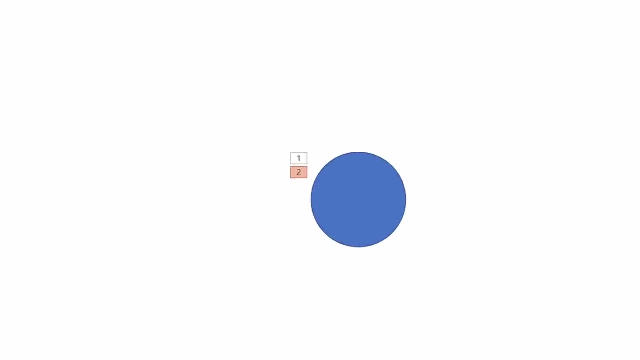 I've now added an additional animation Here. if I go over to the top left hand corner and click on preview here, you see it fly in and then it flies out, So I've now added multiple animations. Also, if we look over at the object that I animated, you'll see these two numbers here. 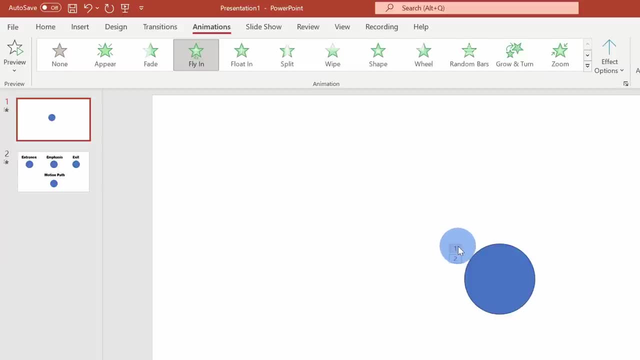 You have a one and a two. If I click on the number one One over here, you'll notice up here on the ribbon that it shifted the animation and it shows that I have a fly in selected. If I click on number two here, it shows that the second animation is the fly out. 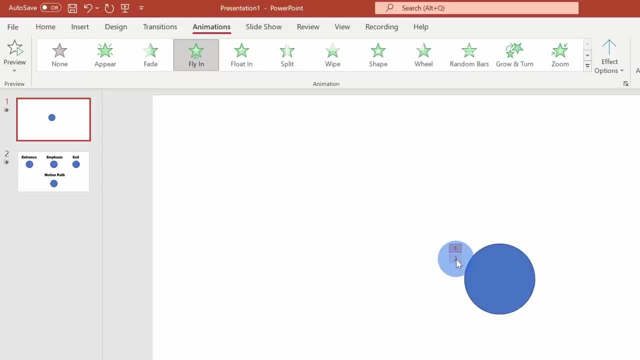 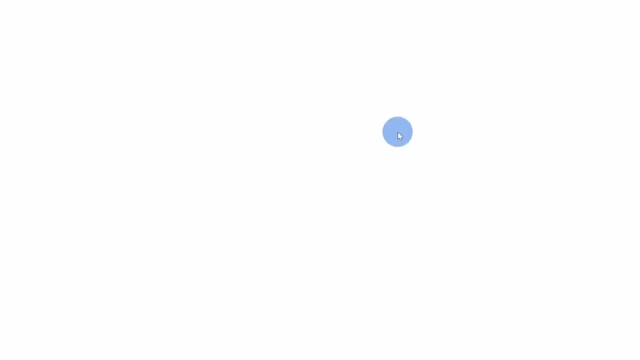 So this is a quick way just to check what animations you have applied to an object. Now that I have two different animations applied to this object, let's jump into presentation mode to see how this works. Right now I'm in presentation mode and the object or the oval isn't yet visible, because 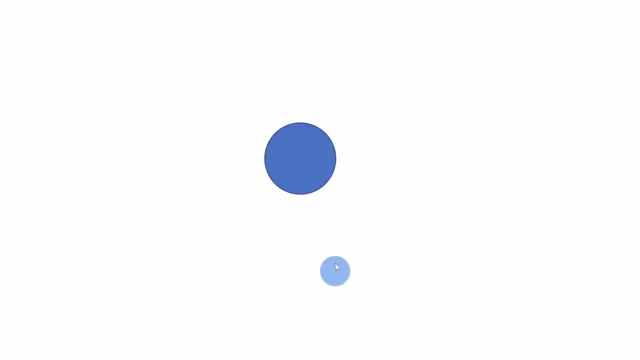 it hasn't entered. I could simply click on the slide. That'll kick off the entrance animation And then, when I click again anywhere on this slide, it'll animate out or it'll fly out. So that's exactly how it should behave. 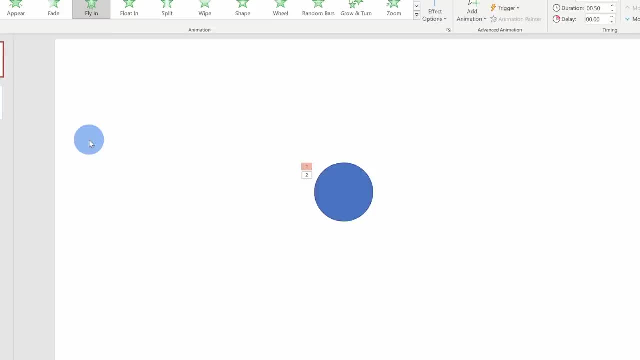 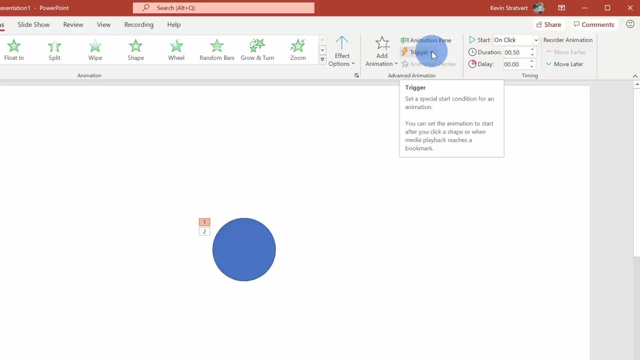 But let's say I want a different trigger for this object. So right up here, right over to the right of add animation, we have this option called trigger, So I could set a condition for when I want this object to animate. So let's click on this and maybe I'll do it for the exit or the fly out animation. 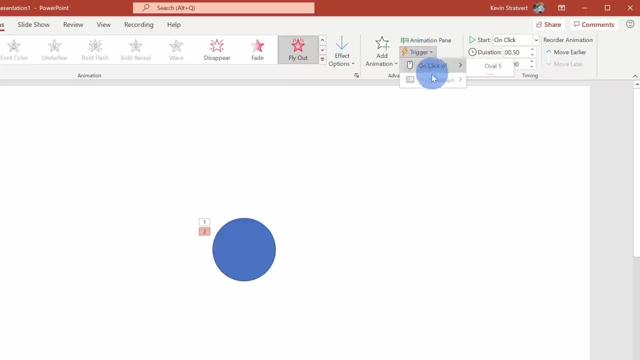 So here I'll click on trigger. and I see that there are two different options: There's on click of and also on bookmark. So right here I can set the trigger to on the click of the oval. So here I'll click on the oval. 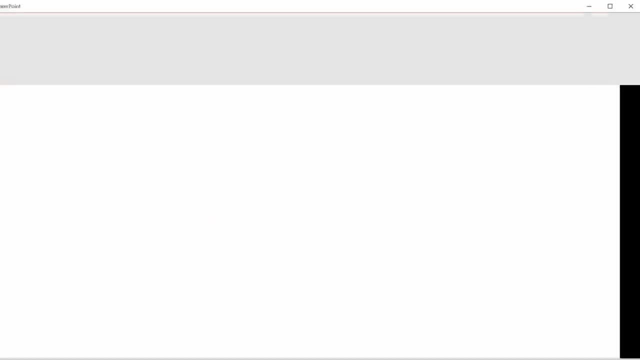 So for it to fly out I have to specifically click on the oval. Here I'll jump in presentation mode again and here I can animate it in. but if I just click on the slide, it'll just simply jump to the next slide. 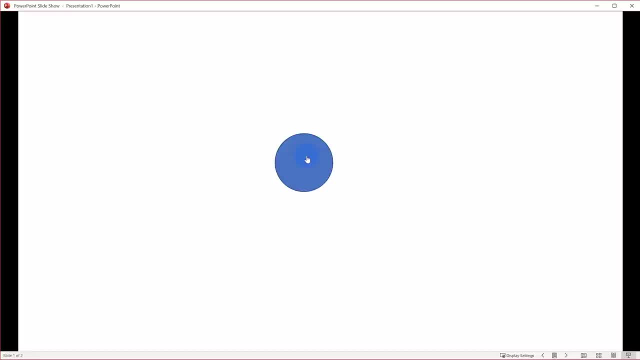 It won't actually animate it out because I have to click on the object. So I'll click on that and that'll now animate out. So, especially if you start building more complex animations, you might want someone to say, click on a button or click in a specific area of your screen to kick off or trigger the animations. 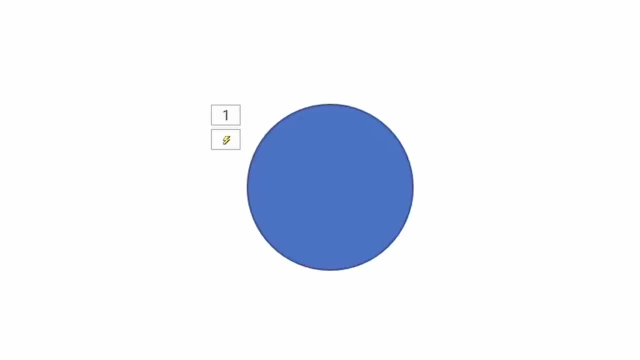 This is a helpful tool that you can use to accomplish that. Now that I've added a trigger over by the oval, once again, you'll see my different animations. I have one and then I have the second one. For the second one, you'll see this trigger icon indicating that I've assigned a trigger. 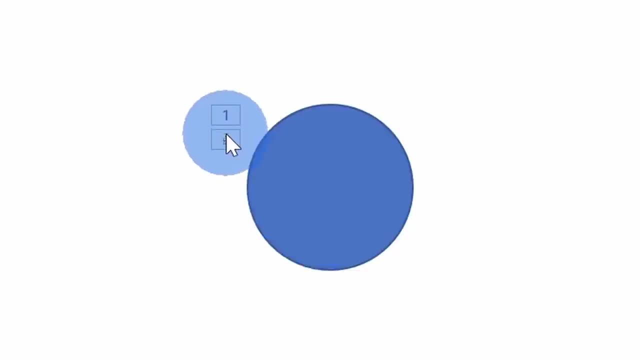 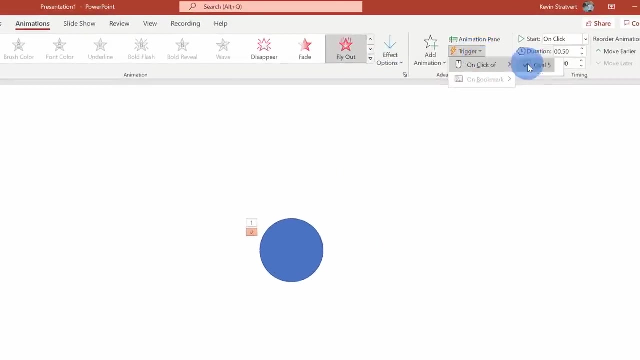 to this second animation. If I want to remove the trigger, I could simply click on step two right here. So I'll select that and up here in the ribbon I could just go right back to trigger. You click on on click of and then I could uncheck oval five. 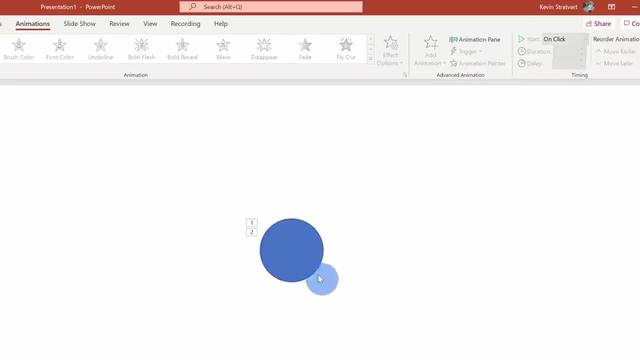 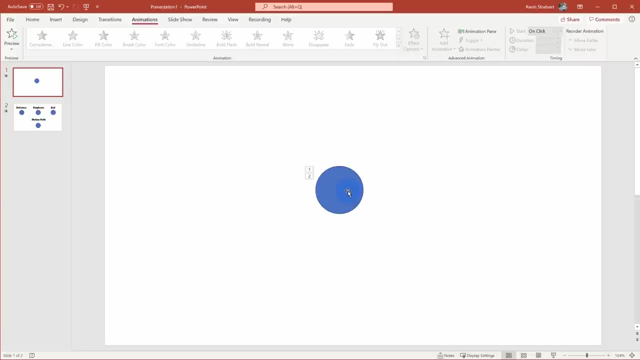 So right now it's back to the original state, where I can click anywhere on the slide to kick off this animation. Now that we have some basic animations working, we've also added multiple animations. What if you want the animation to apply to another shape? 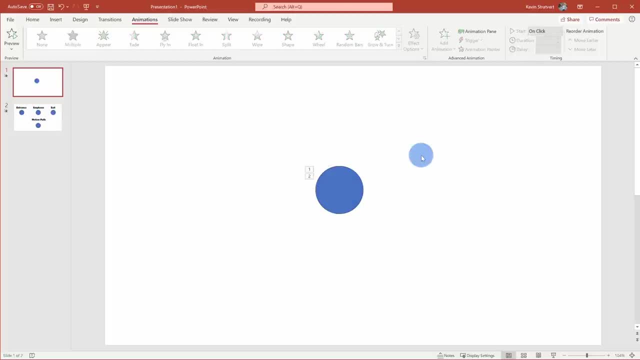 Well, here, for example, I could click on this object and I'll press control C to copy and control V to paste. And so here now I have another oval, and here you'll notice that it carried over the same animations. So first I have the fly in, the fly out. 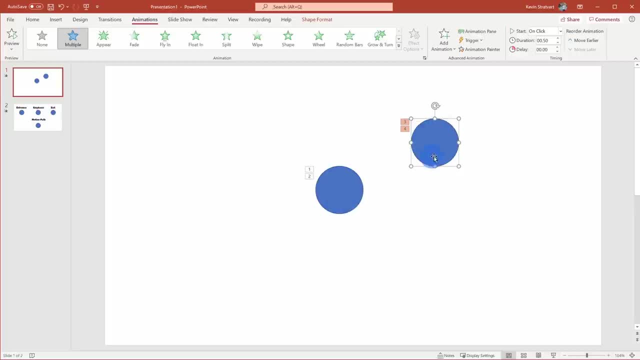 On the first oval And then, once that animation is done, it'll jump to the second oval where it'll both fly in and fly out. So that's one way you can copy the animations: You simply copy the shape and all of those associated animations will carry with it. 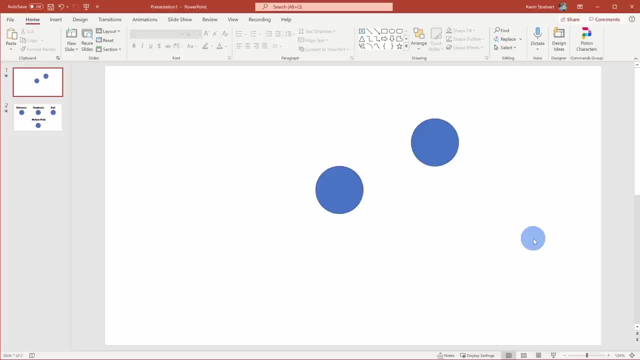 Now let's say you want to add other shapes to your slide and you also want those to carry the same animation. but maybe you don't want to copy and paste Right up here. I'll go right back onto the top, click on insert and then I'll go over. 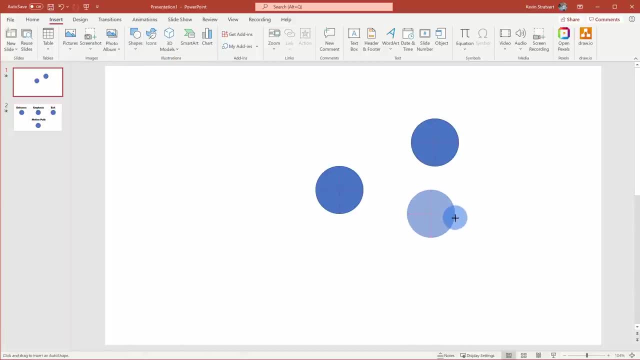 to shapes And once again I'll insert another oval. I'll insert an oval right here and let me copy and paste it, and I'll just paste it two more times. So here I have three new ovals. Now, right now I don't have any animations on these three ovals. 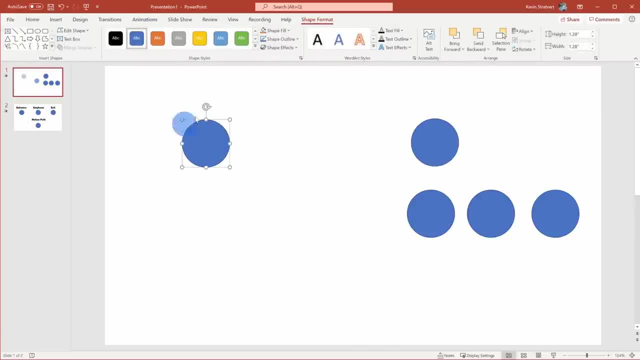 I'll go back to the animation ribbon, and here you see that only this oval- this was our original one- has animations, and the one I copied and pasted also has animations assigned to it. But I want these same animations from the first one and the second one. I want them. 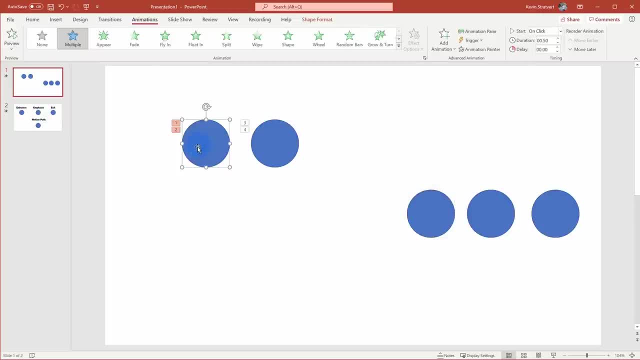 to also apply to these. How can I easily take these animations and apply it to this other shape? This is where the animation painter can help us. When I have this object selected, you'll see that I have these two animations assigned to it. 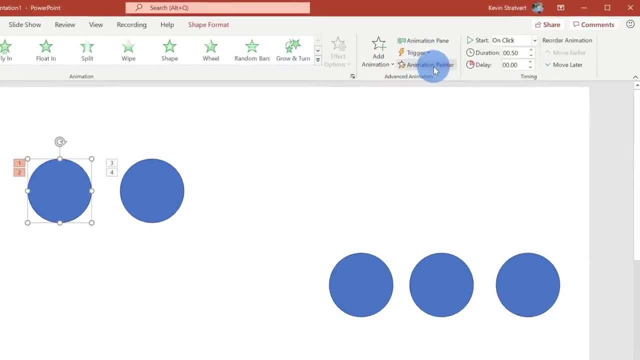 Right up here on the ribbon I have all these different options and there is one called animation painter. What this will do is it takes all of my different animations that I've assigned to this shape and I can very quickly pull it over and then apply it to another shape. 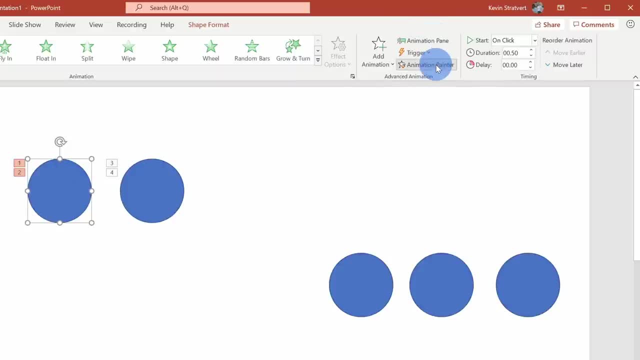 So here, with this shape selected, I'll go up, let's click on animation painter and you'll see that I have this paintbrush right next to my mouse. That indicates that the animation painter is currently active. I'll bring it down and let's click on this shape. 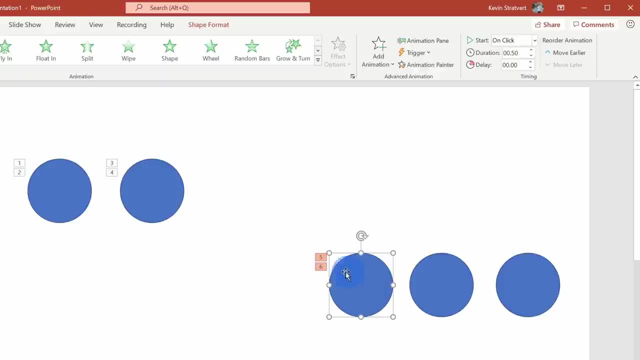 Right now you've got a preview of the animation. It flew in and then it flew out. You also see the 5 and the 6.. So it's now the fifth and also the sixth animation on this slide. So that looks pretty good right now. 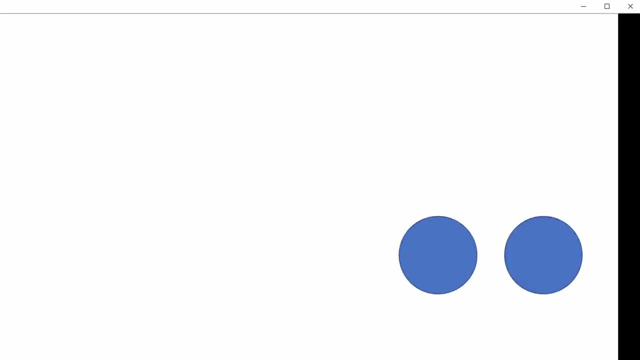 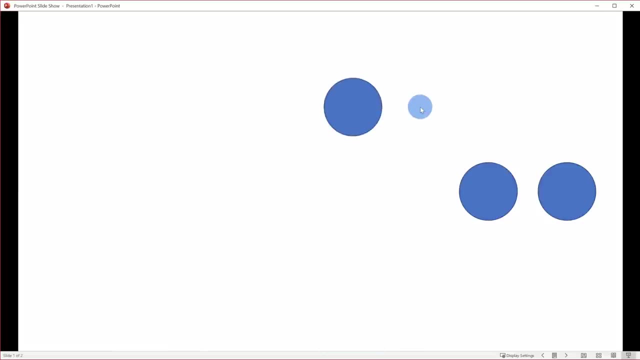 Basically, I took the animations from this first one and I applied it to the second one Here. if I throw it into presentation mode, we see the first one flies in, flies out, this one flies in, flies out, and then the third one flies in and flies out. 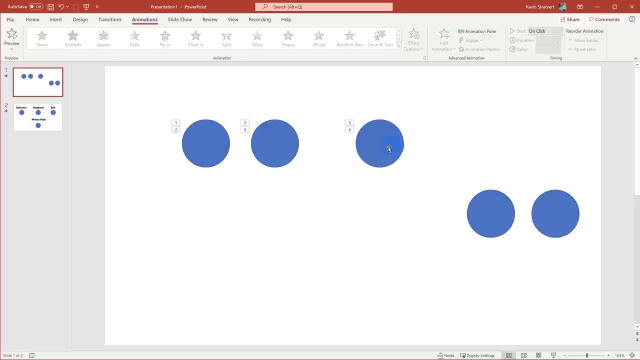 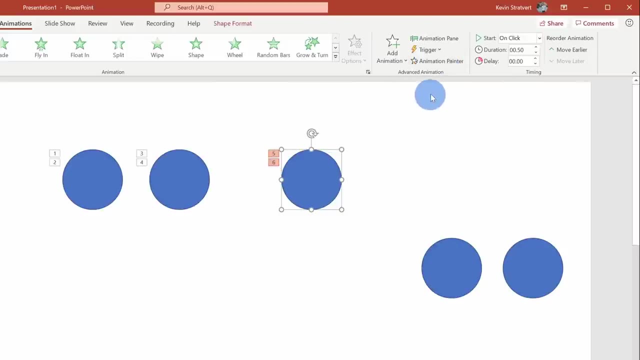 It's taken the animation exactly as it was on the first one and it's applied it to this one. Now I do have two more ovals and I could go through with the animation painter. I could click here, click on the next shape, click on the animation painter again. 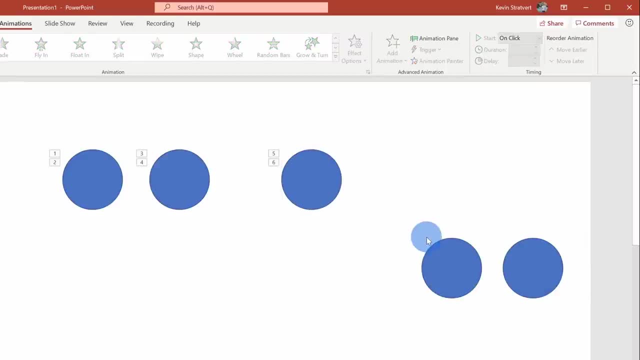 and then click on the next shape. But let's say I have a whole bunch of different objects that I want to apply the animation to. There's got to be an easier way. I can click on this shape and this has the animations, And instead of just pressing once on the animation painter, I'll double click on it. 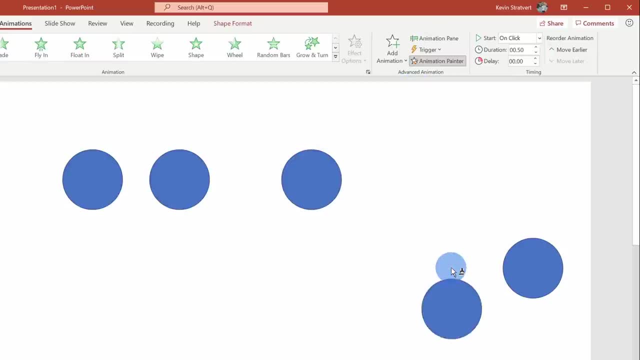 Now that I've double clicked on it once again, you see the paintbrush icon and I could click on this shape and you'll see that the paintbrush is still there. So I can now go over, click on another shape And once again, that's applied the same animation to this new shape. 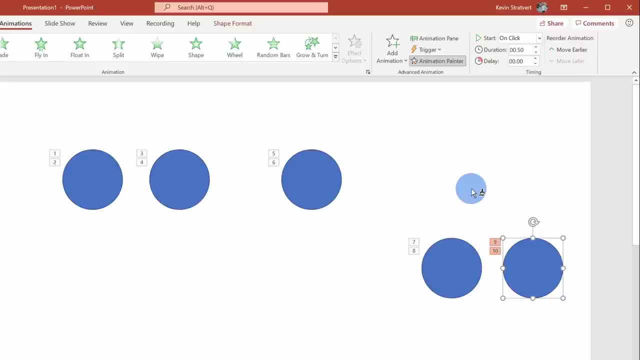 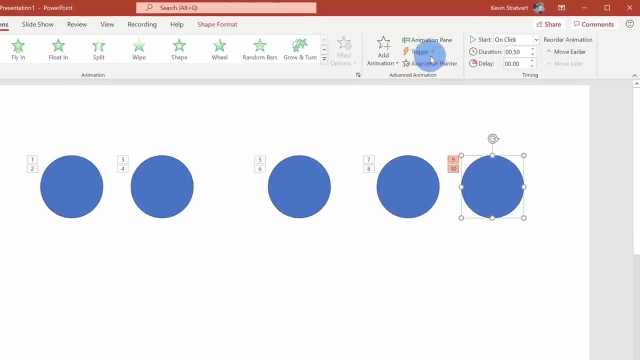 Once I'm done applying the animation, I'll simply click on the escape key. Now, once again, when we looked at the trigger, we saw how you could click on the shape to trigger it, But here, for example, I could select this shape. 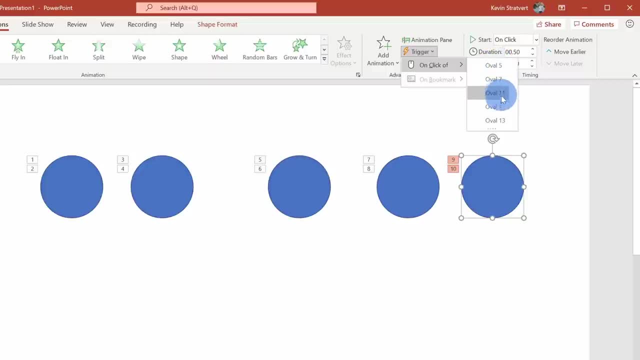 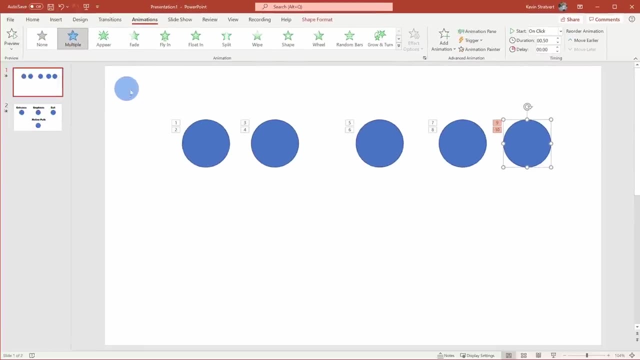 And if I go back over to trigger here, you could see a click on any one of these shapes can trigger the animation on this one. So once again, like I said earlier, you can have say, a button or some other control on your slide. 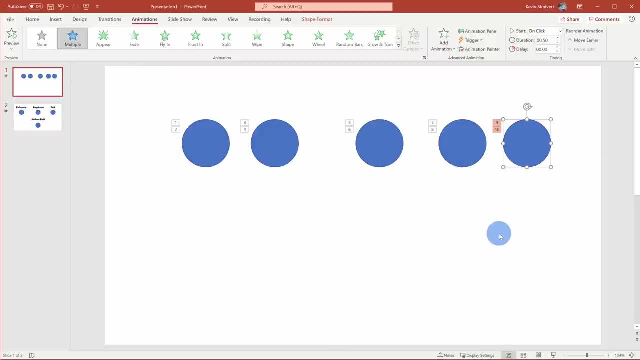 that'll kick off an animation somewhere else on your slide. So it's pretty powerful stuff. We've gone through a lot of the basics now And, just to simplify, I'm going to remove some of these shapes. just to make it easier, I'll select these three shapes that I added and I'll delete them. 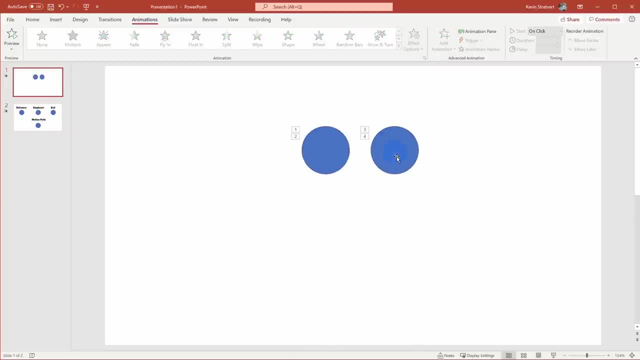 So right now we just have two of these ovals left And right now we have them animated. Now, especially as you start getting a lot of animations here- you see, I have one through four different animations- It could start getting a little disoriented. 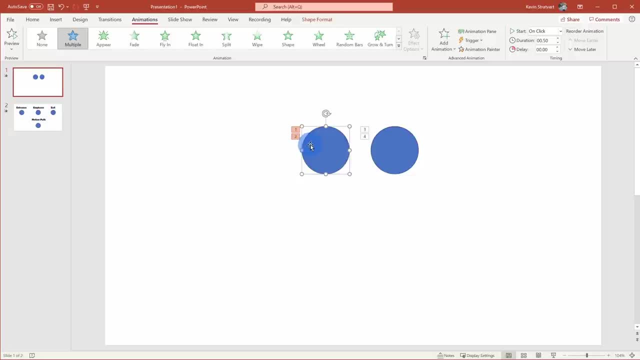 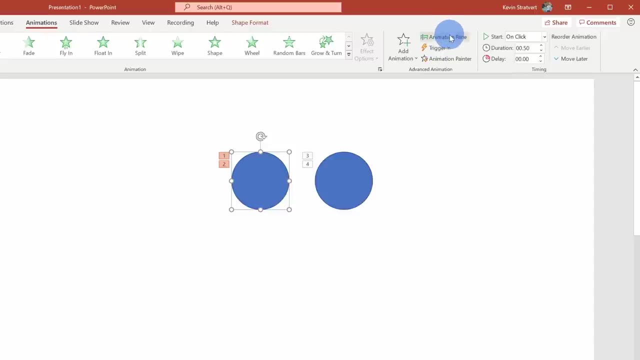 Let's say, maybe I want this one to animate before this oval. The easiest way to adjust the order of animations is right up here under advanced animation, There is an option called animation pane. When I click on this, this opens up a pane over on the right hand side. 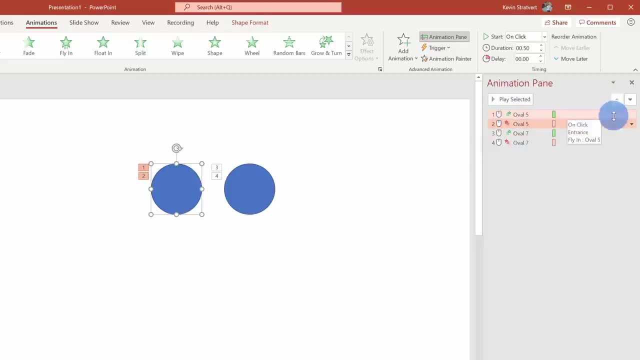 And here, if I select the first oval, it'll highlight all the animations associated with this oval. Here, for example, too, I could click on the second oval, And here you'll see that it highlights all of those associated animations. Now let's say that I wanted this one. 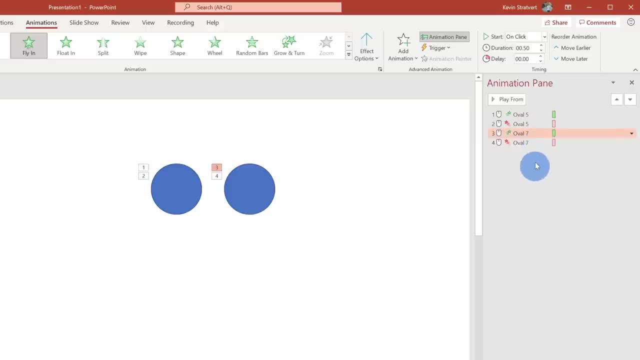 Let's say that I wanted this one to animate before this oval. Well, here I could select oval seven, and I'll select all the different options here, And then I can click on this up arrow and this will move it up in the order. 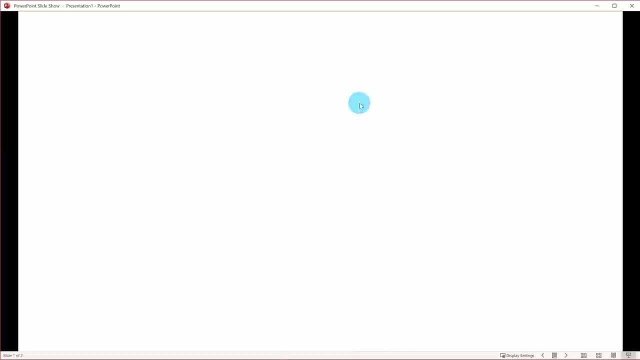 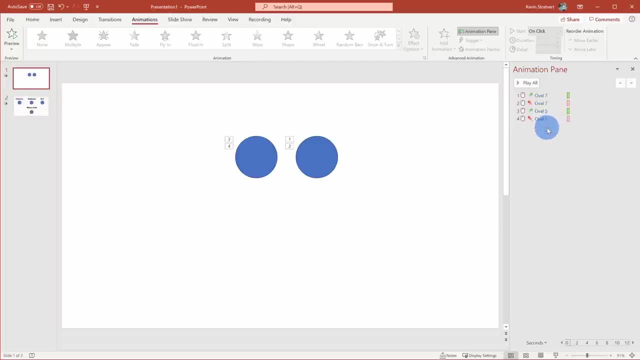 So here now, if I throw it into presentation mode here, you'll see this: one comes in, flies out, and then the other one flies in and flies out. That allows me to shift the order. So, especially when you start getting a lot of animations, if you want to move things around or have things animate in a different order, 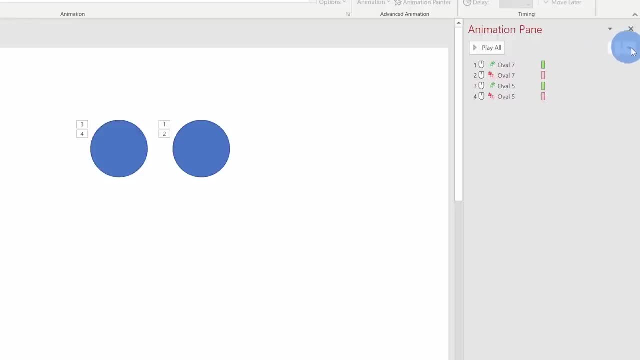 the animation pane can help you with that. Along with using the arrows to move the panes, the position of an animation- you can also select the item right here in the animation pane and then you can move it to the position where you want it. 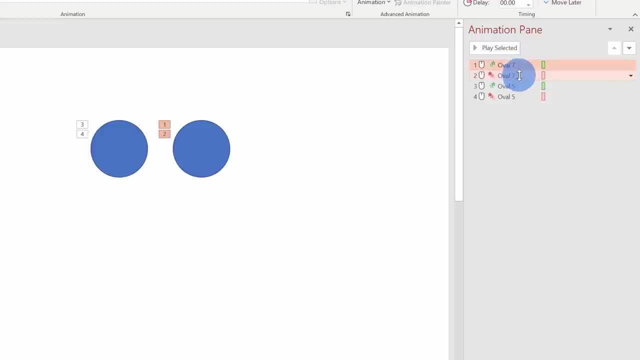 So here I've selected the entrance animation and I can also press the shift key to select the exit animation. Here I can select this entire group and I'll pull it down to the bottom. So here you'll see, as I pull it, I could choose the exact position where I want to place it. 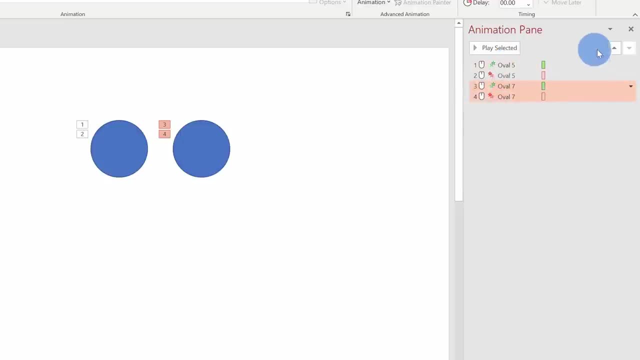 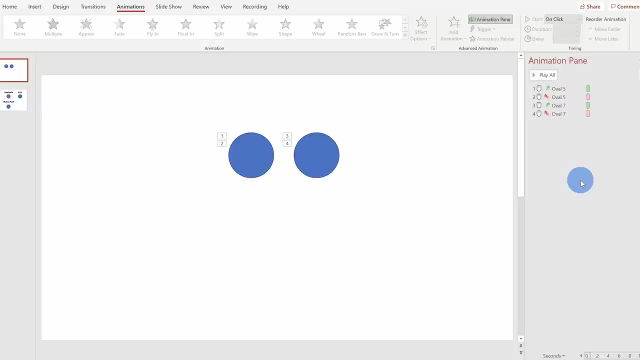 I'll simply leave that animation at the end. So once again, you could simply drag and drop, or you could use the arrows over here. Now, so far, with all of our animations, it requires you to click before the animation takes effect. 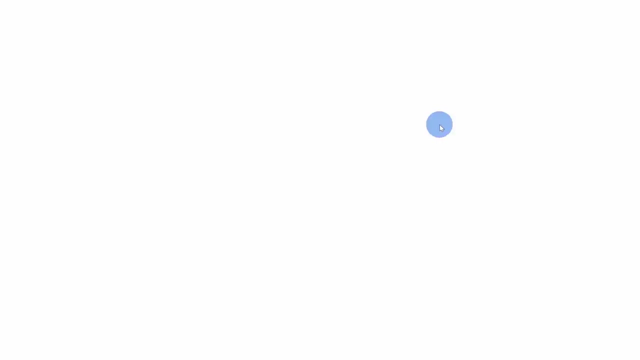 So here, for example, I'll jump into presentation mode again- For this shape to fly in or that fly in animation to occur, I have to click my mouse button and then you'll see the animation takes place, And then I have to click again for the next animation to take place. 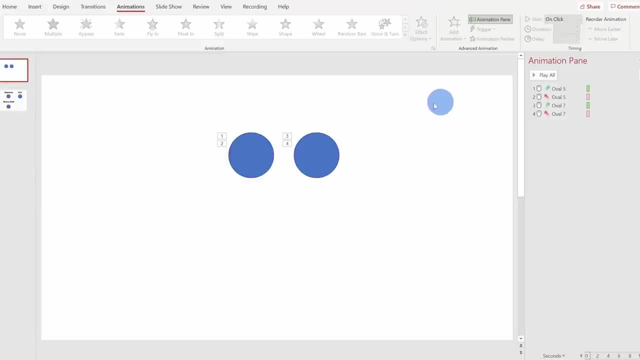 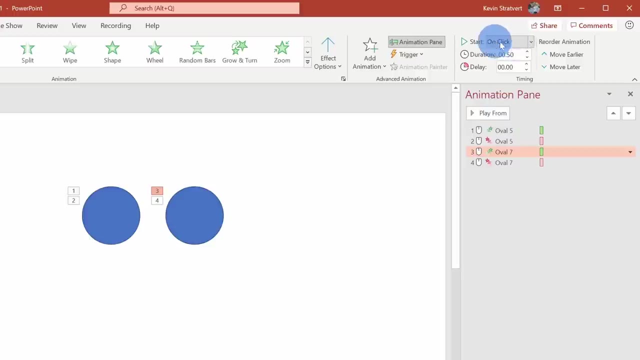 I can change that, so it's not just based on click. So here, if I come over to my second shape right now, here I'll select the intro animation And right up here I see that it's currently set to on click. If I also look down below at the animation pane, 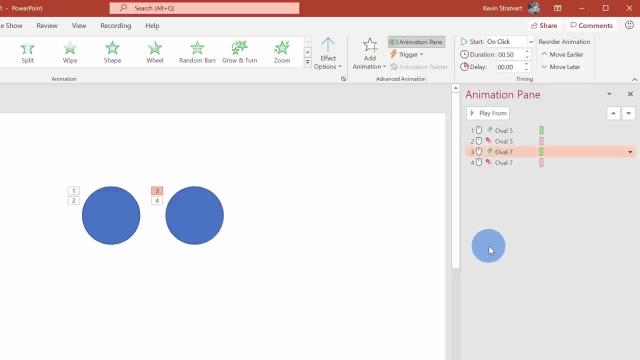 I see a mouse icon indicating that it's currently triggered by my mouse click. Now, let's say that I wanted to maybe animate with the previous option, Or maybe I wanted to animate after the previous option. I can set that. So here I have the fly-in animation for this oval. 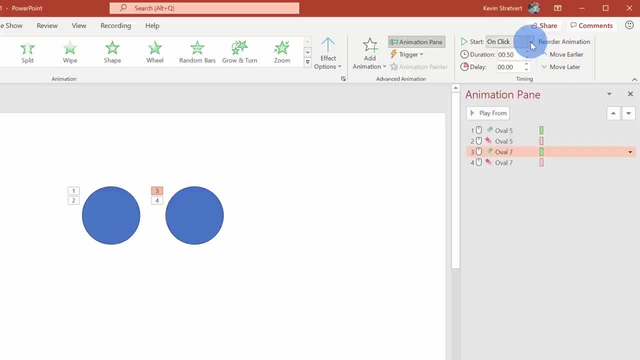 So this is my third animation. If I go up to the top instead of going on, click I could select this and I can have it go with the previous one. So if I select this, when oval 5 flies out, oval 7 will automatically fly in at the same time. 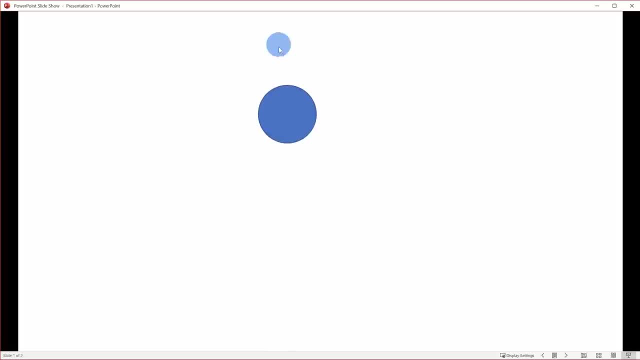 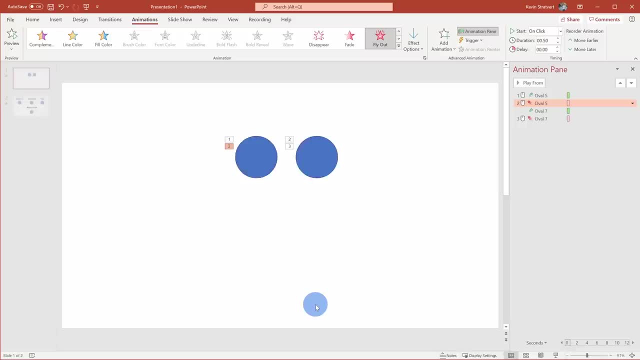 So let's jump into presentation mode and let's see how this works Here. I'll click to bring it in and now, when I click for it to fly out, you'll see that the next shape flies in at the same time as the other one flying out. 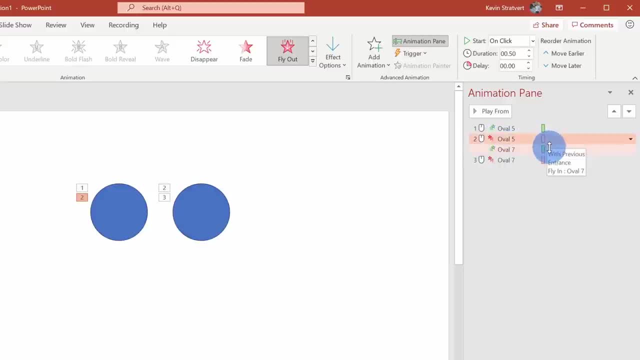 Over on the right hand side you'll see that these currently are occurring at the same time. So I have the mouse click and then you can see here on the timeline that this action or this animation occurs right at the same time as the next animation. 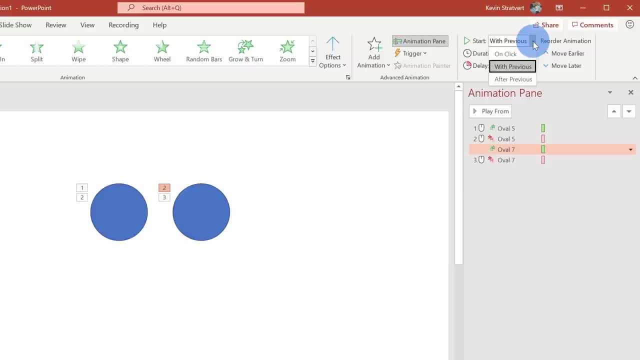 Here I'll select oval 7 and once again, let's go up to this dropdown list and instead of going with previous, let's try after previous. When I select after previous, you'll see this clock appear right here. This means that there's going to be a slight delay or it's going to occur after the animation. 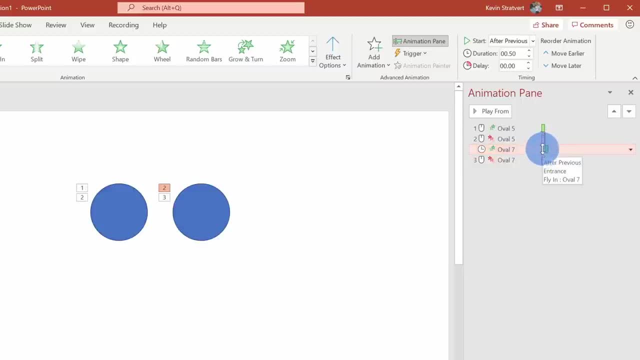 right up here You'll also see on the timeline you can see a visual of when the animation is occurring. So here you'll see that the fly out animation will happen, And as soon as that's done, then the fly in animation will start. 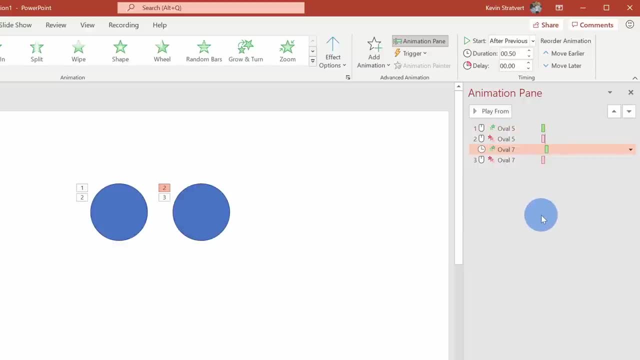 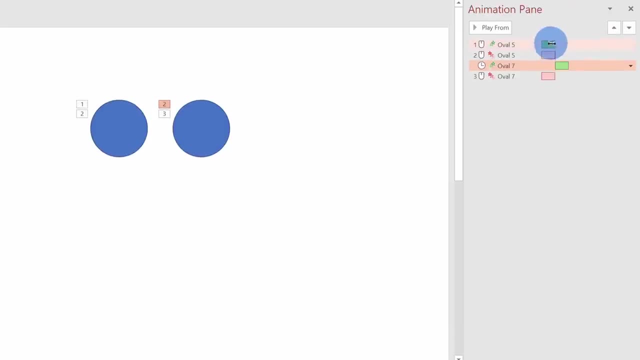 Also, you'll see that these little icons on the timeline. they're kind of small and hard to see. Right down here I can click on seconds and I can zoom in So that way we can make it a little bit bigger and easier to see when these different animations. 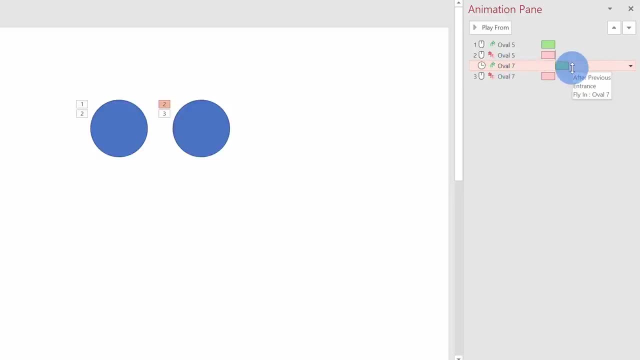 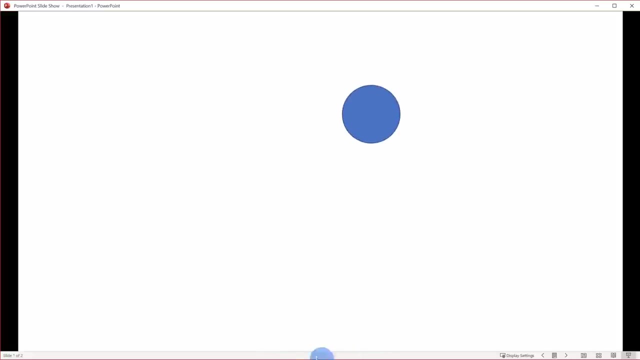 are occurring. Now that I have oval 7, starting after the previous one, once again, let's jump into presentation mode Here. I'll click in and that flies in, and now we'll see it fly out, And then, as soon as it finishes flying out, the next one will fly in. 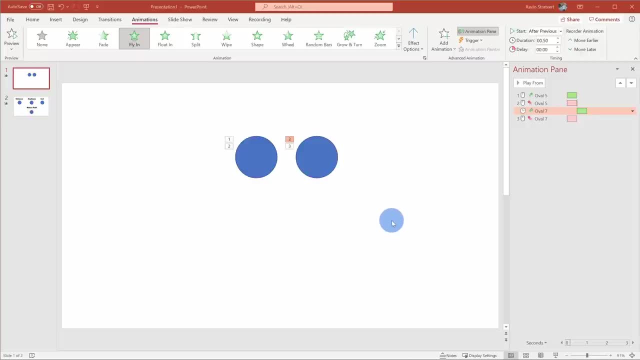 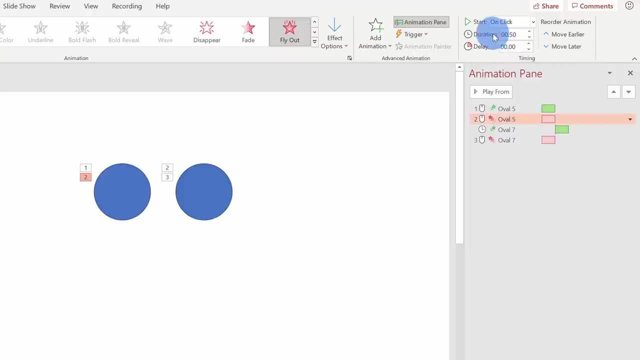 So I want to look at a few additional options you have for animations. So right up here on the top, let's say on the fly out of oval 5, when it's flying out, Right up here under timing, we can set the duration of the fly out. 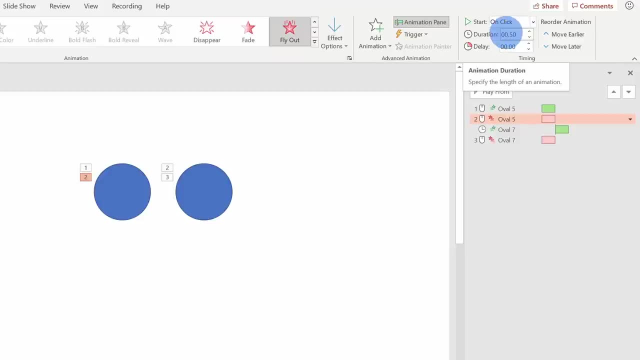 And then right now it's set to 0.5 seconds, So it's a fairly quick fly out. Now I could adjust this. Let's say I want it to take maybe, let's say, two seconds, just to make it really obvious. 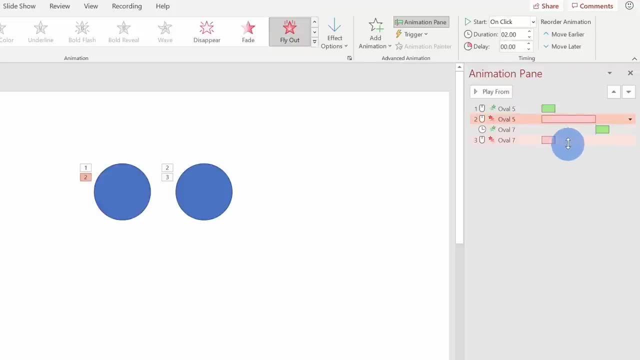 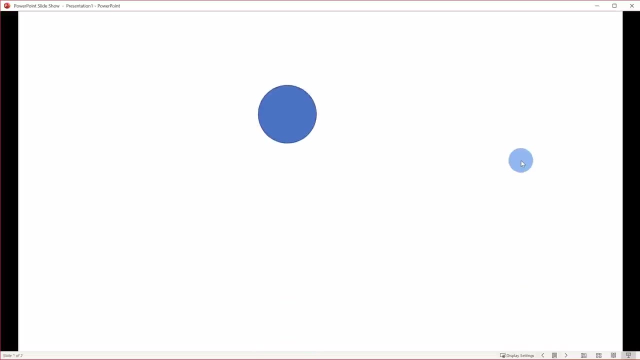 that it's a little slower. When I enter 2 on here, you'll notice right here in the timeline it greatly expands how much time it's taking. So here, if I jump into presentation mode, I have it fly in and now you'll see the fly. 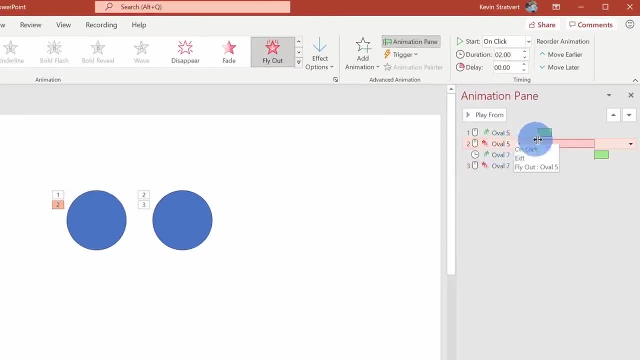 out is a lot slower, So I have full control over how long it takes for that object to come in or go out. Now, along with setting the duration, I can also set a delay. So this is the delay from when I have the animation start to when it actually starts. 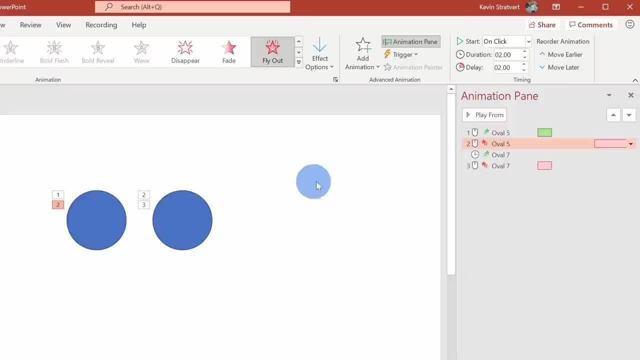 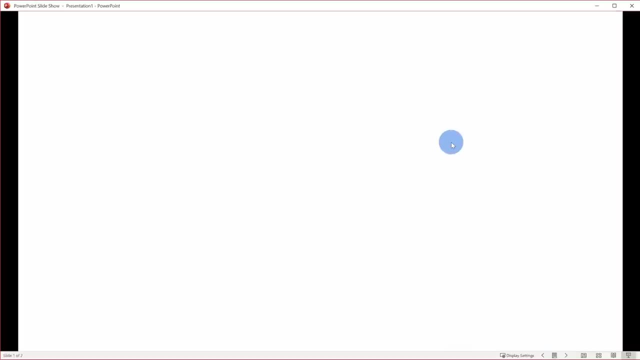 animating. So here maybe I'll set this to: let's go with two seconds for delay. Here you'll see it pushed it back. So I have this first animation and then there's a delay before the second one starts. So once again I'll jump into presentation mode. 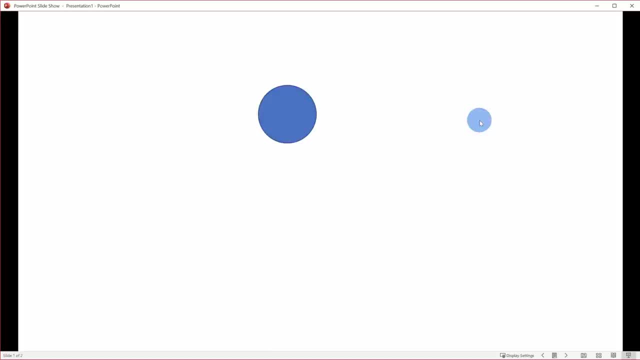 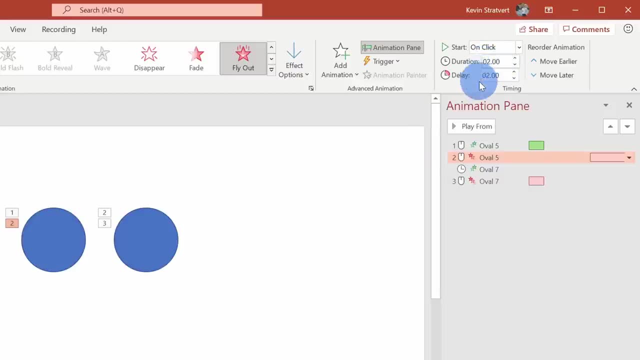 Here we have it. fly in Now. I'll click on my mouse and you'll see that it hesitates before then animates out. So those are two additional tools that I have to animate different objects. Now, as I've been doing this, you'll notice that it's been updating the timeline. 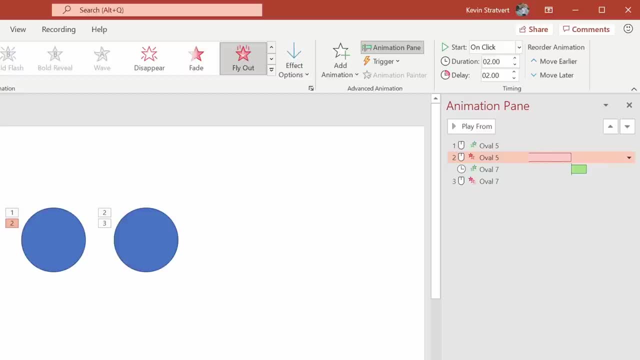 And so here it added a gap for the delay, And here, if I go over, you can see how long the duration of this animation is. I'm going to zoom out just a little bit so we can see all of the different animations. Now I could also click on the timeline and I can drag the object. 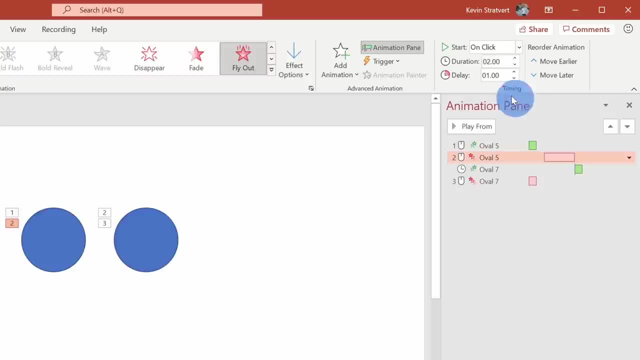 The item here. So here maybe I just want the delay to be one second. I could drag it to the one second position Here. you see, as I'm dragging it I get a little tool tip that tells me what the delay is. 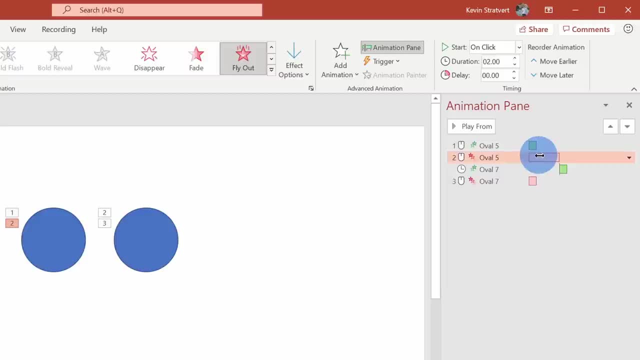 So here I see that right here would be 0.3 seconds, and here I could bring it back down to zero seconds. Also, not only can I adjust the delay by dragging and dropping this object on the timeline, I could also click on the ends over here to adjust the total duration. 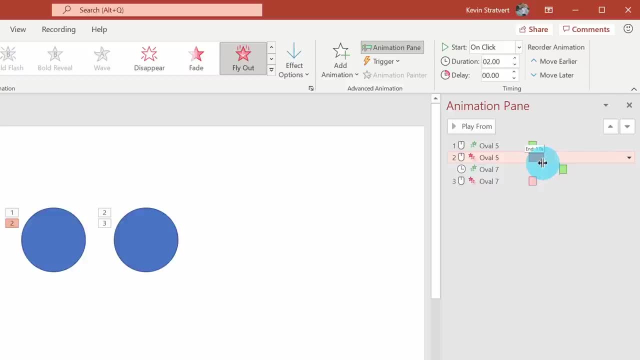 So here I'll click on the end and here I can bring it right back down to, let's say, one second for this animation. So this is another way that I can simply just use my mouse to change the duration and also the delay. Now that we've played around a little bit with the animation pane, I want to show you 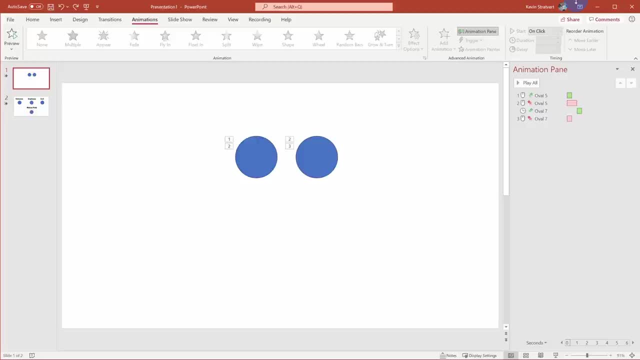 how we can add additional animations to a shape. So right over here, let's say that I want it to grow in between the fly in and the fly out. Now remember that if I go up here right now, I see that there are multiple animations assigned. 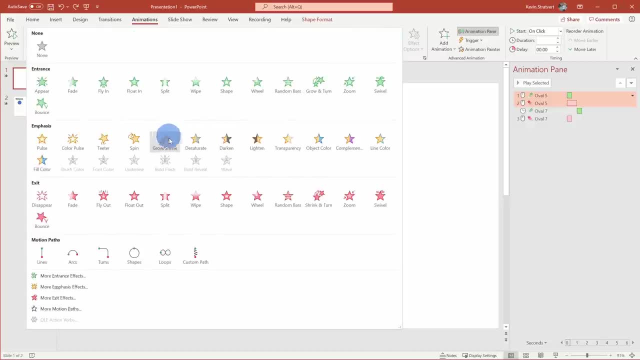 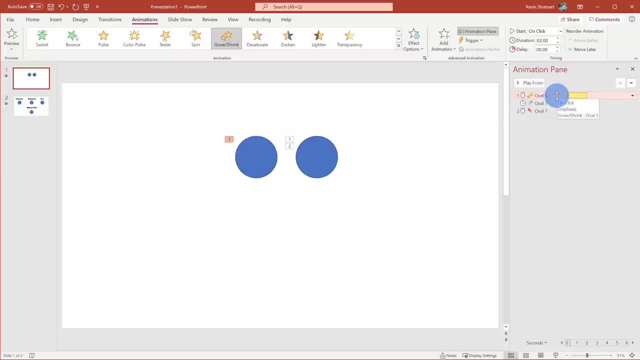 to this object. If I go over here and let's say, I select grow and shrink Here, I selected that And once again, when you just select from up here, it'll overwrite any animations that you already have in place. So remember, once you've already set animations, you don't want to use this section anymore. 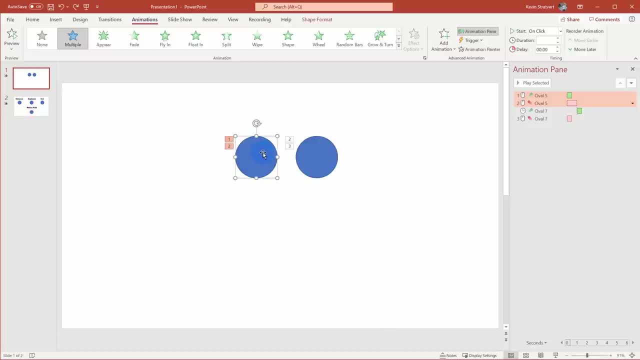 I'm going to undo that with control Z. instead let's select this shape And then once again let's go up to add animation, and over here I'll select grow and shrink. So here now, that added the grow and shrink animation to the animation pane. but here 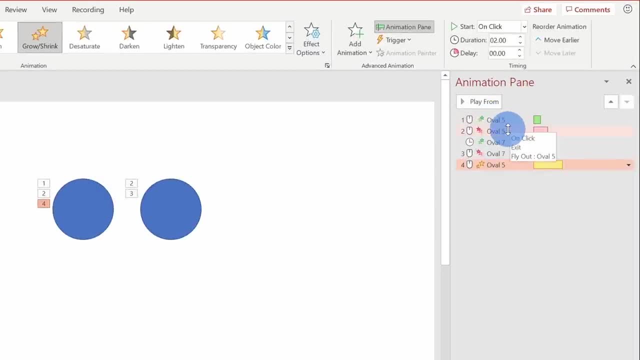 you notice, it's at the very bottom and I want it to fly in, Grow and shrink and then fly out. So here I'll select this new animation that I added and I'll simply pull it up in the list and I'll put it in between. 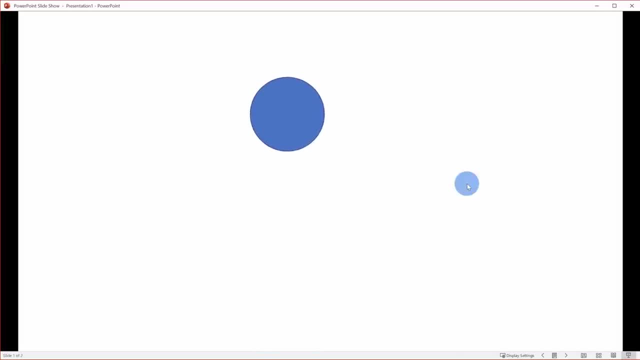 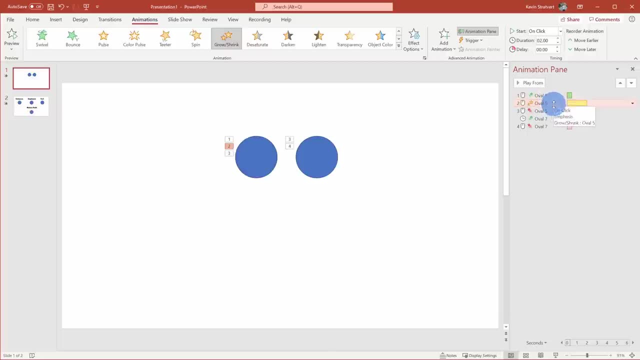 So right now, if I jump into presentation mode here, it flies in, it'll grow, and then I'll click it again and it flies out. So that's an easy way to add additional animations And this way you can grow out your animation sequence. 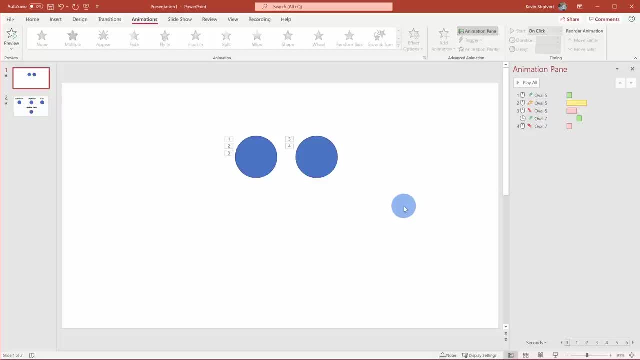 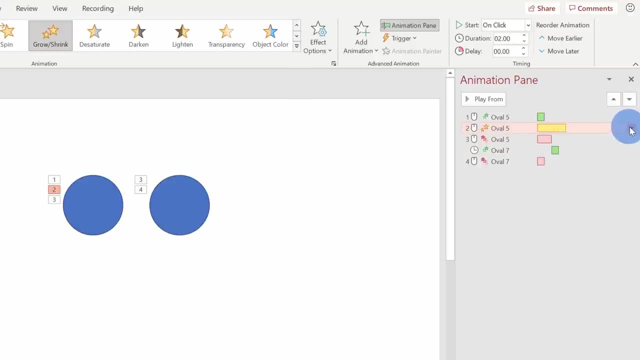 Within the animation pane we can also access a lot of different advanced options Here. when I go over into the animation pane and let's say I click on one of these items over on the right hand side, you'll see this little drop down icon. 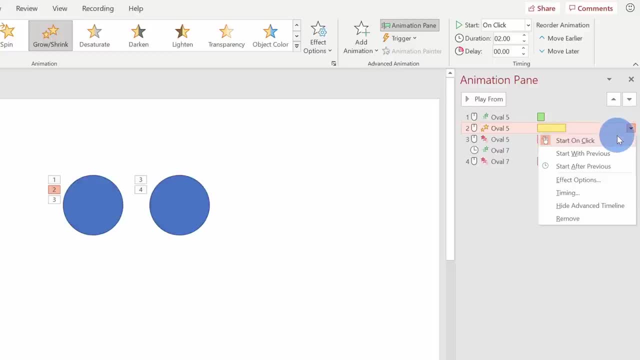 Let's click on that Right here. this exposes some additional options. For example, once again, just like we did above, you can set whether it starts on click with previous or after previous. So this is another way to access those same controls. 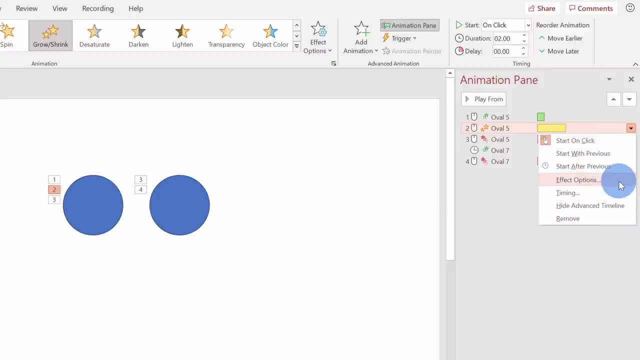 But down here now we have some additional options. You have effect options, you have timing. you could hide the advanced timeline so you won't see the timeline behind here, or you could simply remove the animation altogether. Now, the two that I want to talk about here are the two that I want to talk about in this. 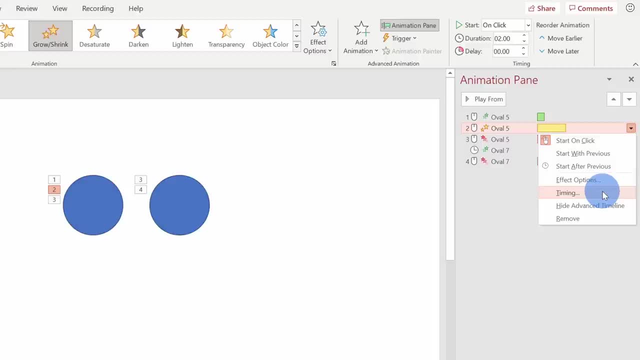 video, One that I want to look at. let's jump into effect options and also timing, and let's start with timing. When I click on timing over here on the left hand side, once again, you can see that it currently is set to start on click. 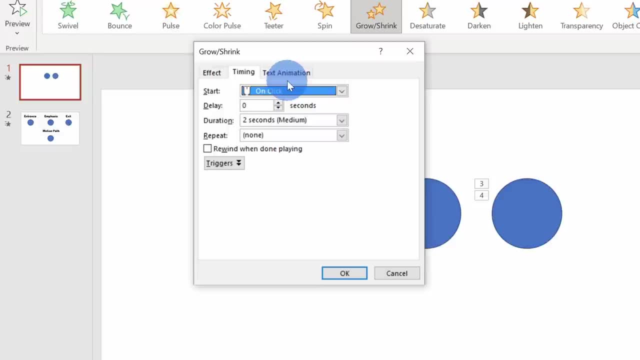 So, once again, this is another way to access. when this animation starts Right down here, I could also see the delay. We were able to set the delay up here as well, and here we could set the duration. But there is one additional new option that we can't access on the ribbon, and that's 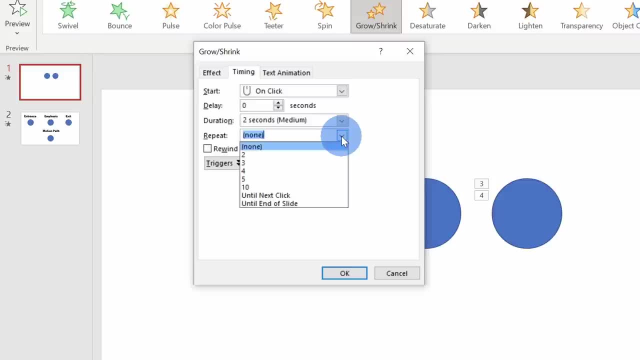 called repeat. So here I can choose to repeat my animation. So maybe I'll just say Until the next click. So it'll just keep animating again and again. There's also the option to rewind when done playing. So let's say you have a motion path and maybe it goes from one side to the other. 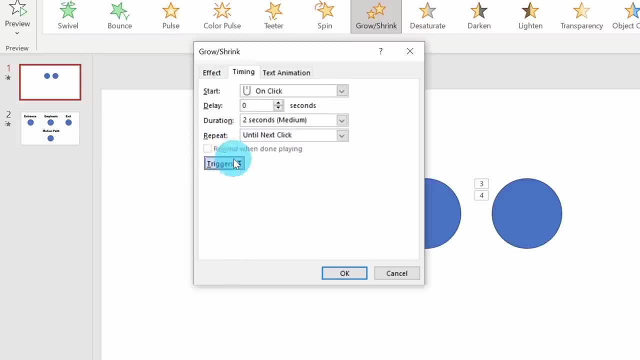 Once the animation is done, you can have it reset. So you also have that option And once again, we have different triggers that we can set. I'm going to leave this as is for now and let's simply go with the repeat option. 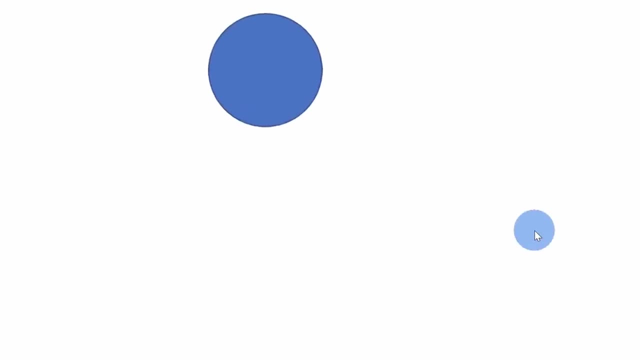 I'll click on OK, and let's now play the slide. So here it comes in, and now I kick off the grow animation And here you'll see that it just animates again and again. So this can be a neat way to bring different effects into your slide. 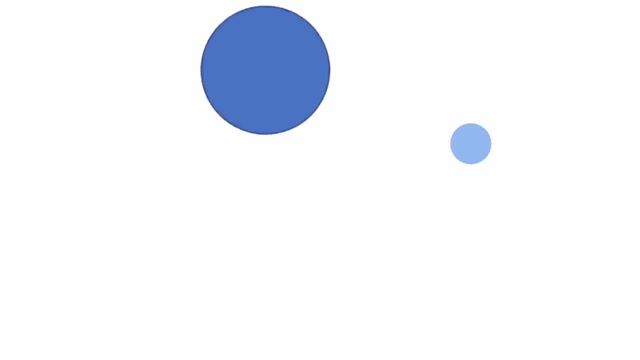 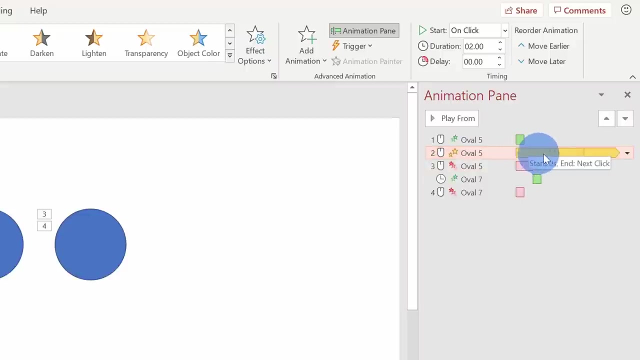 Let's say you want to have a pulsing light or something else. You can use this repeat effect to just keep it playing on your slide Over on the animation pane right here on the timeline, you'll see that it also updated the visual to reflect that it's now repeating. 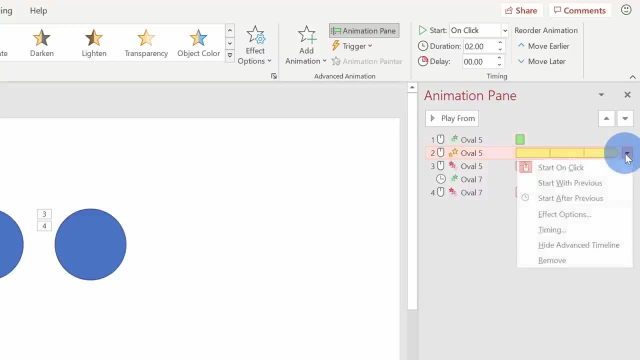 If I want to turn off the repeat animation, I can turn it off the same way. I'll click on the drop down, go back over to timing and here I'll turn it so it doesn't repeat at all. Then I'll click OK. 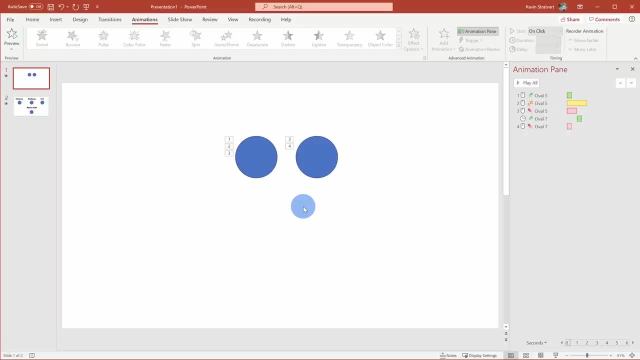 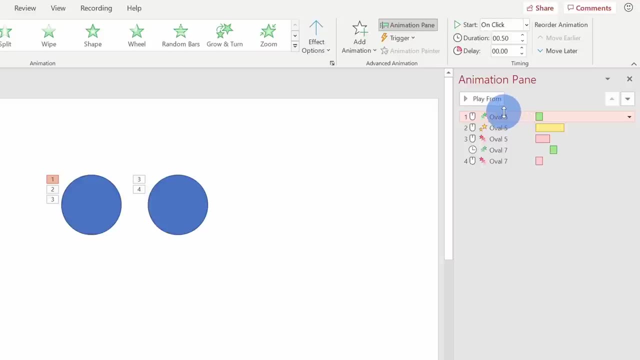 Next, I want to show you some of the advanced effects that we can access. So here again, I'll click on this first shape and I'll click on the fly in animation And over here. here too, I also have that drop down. 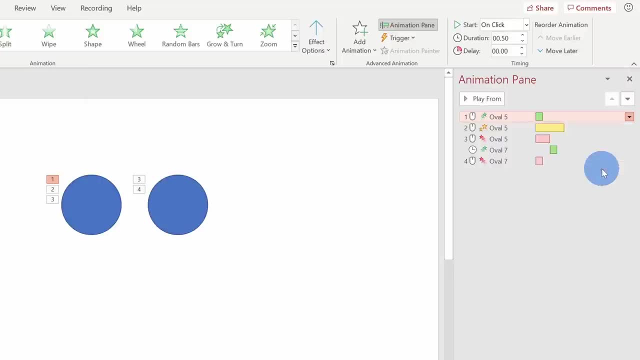 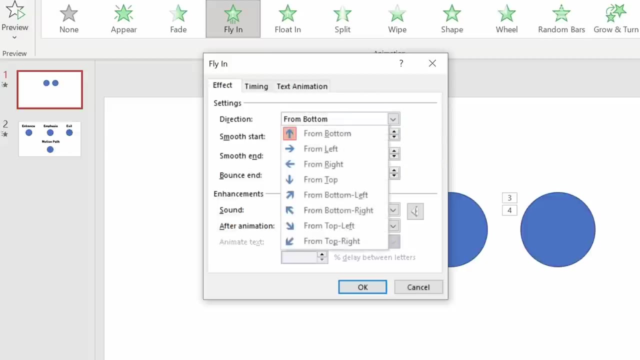 When I click in this, we see effect options. Let's click into this. This opens up a prompt with all of my effect options, And here too, I could also set the direction that it flies in from. So that was available here, and this is just another way to access those same controls. 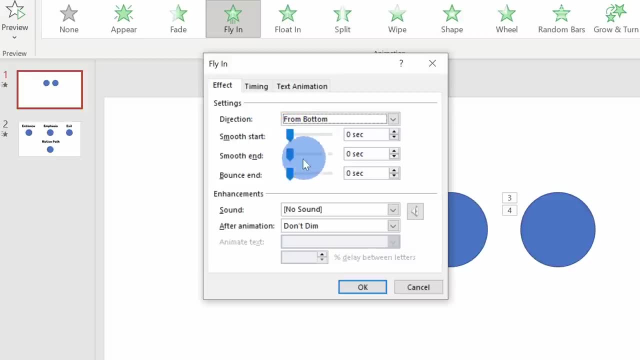 I can set whether there's a smooth start, a smooth end or a bounce end, and I could even set sounds to go along with this animation. And even after the animation, you can have it dim or you can even adjust the colors. 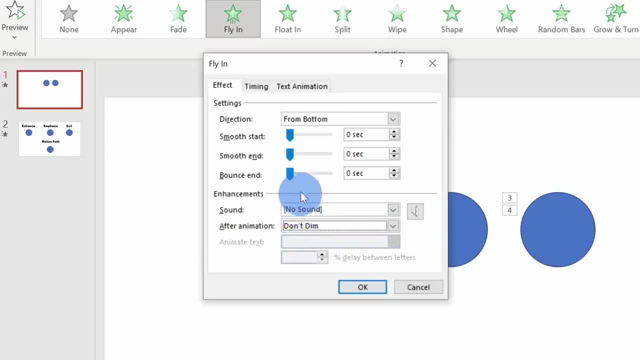 So there's quite a bit that you can do here. Now, why don't we test out one of these, and maybe I'll set a smooth end and I'll set it to 0.5 seconds, just so it really stands out? Also, maybe we'll play a sound to go along with this. 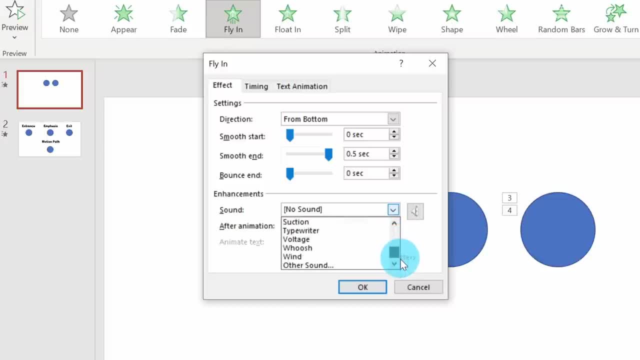 So I have a bunch of different options. In fact, if you want to set a custom sound, you can even select other options. So I'm going to go ahead and do that. I'm going to go ahead and do that. There's another sound down here and you can select a sound from your computer. 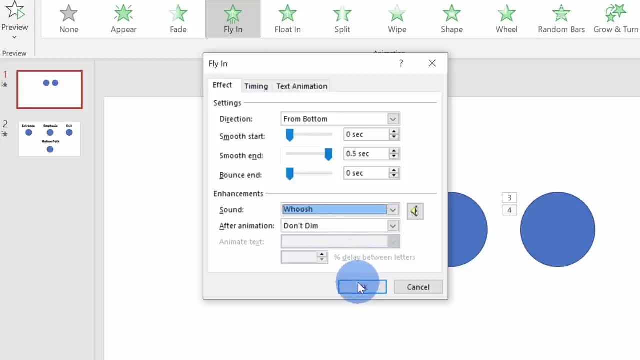 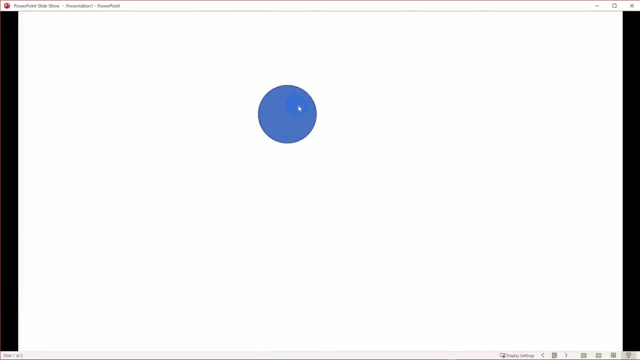 Now let's go with this whoosh as the oval flies into the screen. Next, let's click on OK. Next let's jump into presentation mode to see how this looks. So here now you see that it slowly eases in, and you also heard a sound go along with it. 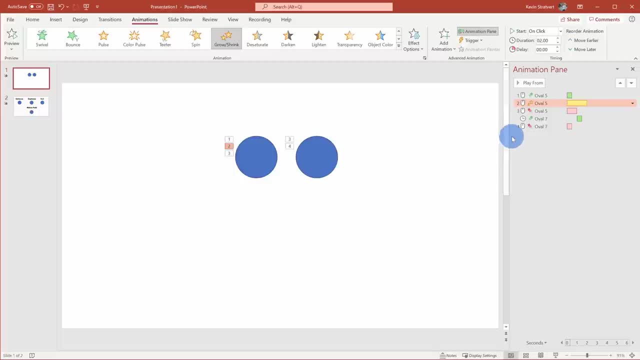 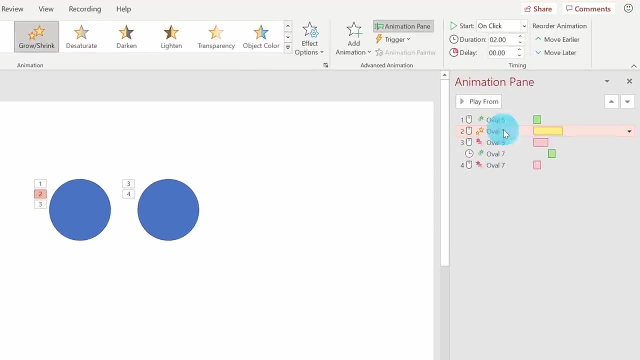 As you start building out your animations, you might decide that well, maybe you don't like one of these animations, So here I have it, fly in, I have it grow, and then I have it fly out. But let's say I don't want it to grow in between. 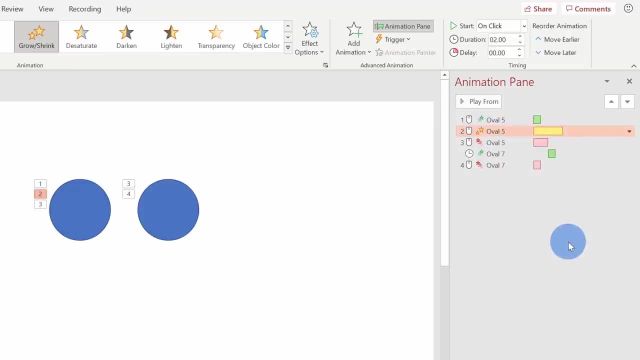 So I can select that animation on my animation pane and then I could hit the delete key and that'll remove that animation. Once I start adding a whole bunch of different animations, you might have a very complex set of animations on your slide And maybe you want to preview your animations. but you don't want to always have to preview. 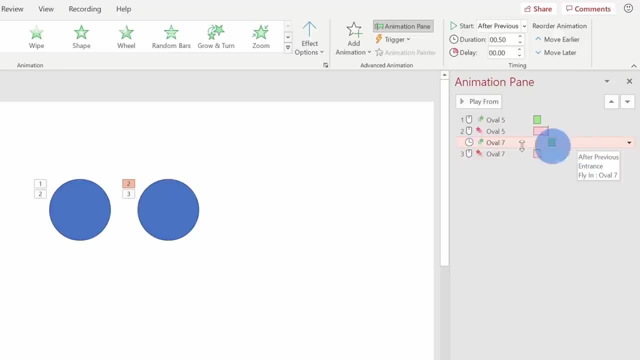 from the beginning. Right here I can select an item in my animation pane and then I see this button that says play from. So here, if I click on this, it'll simply fly in and fly out for oval 7 and it won't show. 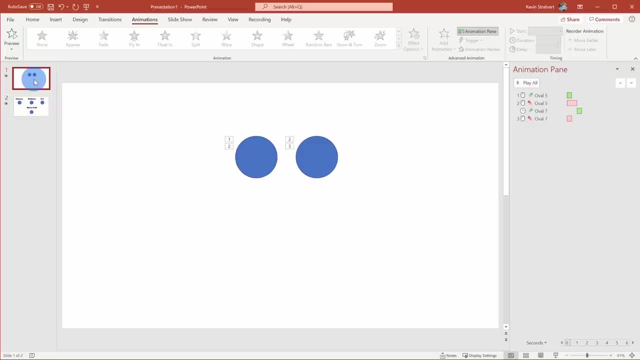 me the animation for oval 1.. So far we've been looking at all of the fundamentals of how you can animate objects, But what about text? and are there any differences? Let's add another slide in your presentation and let's go up to insert, and then let's insert. 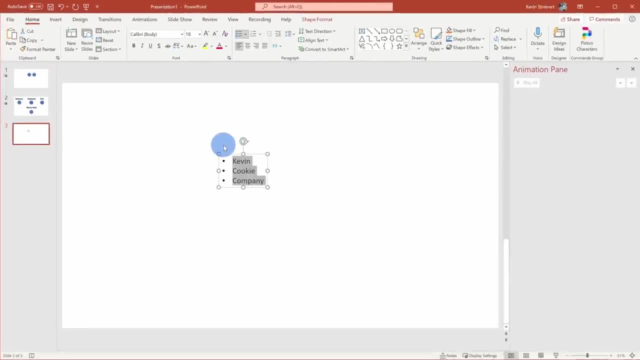 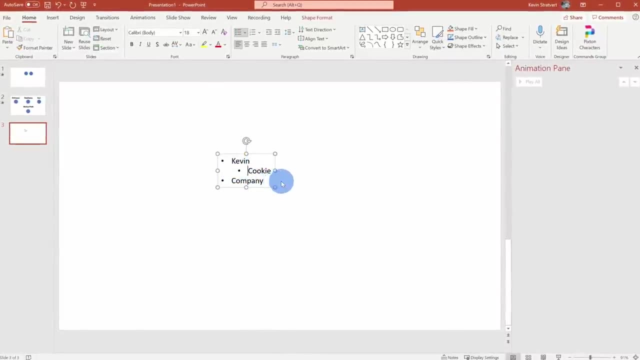 some text. I'll click on text box right here. I've inserted some text on my slide and this is a bulleted list And let's say, maybe I'll move cookie and I'll make that a second level bullet. So right now I have some text on the slide and I'll expand the size a little bit as well. 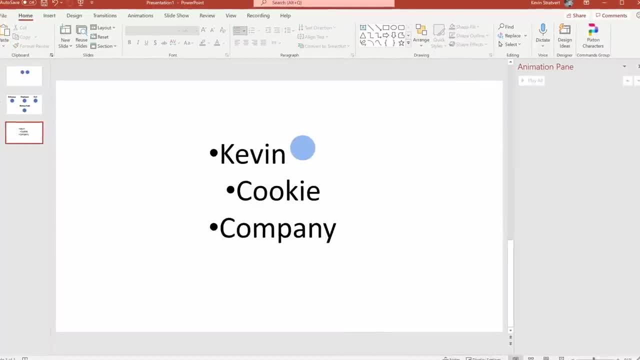 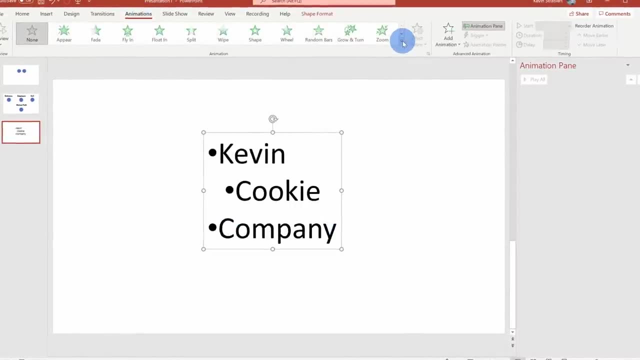 just so it's a little bit easier to see. Now I can also apply animations to text Here. I'll select this object or the text object and I'll go to animations on top. When I click over here on animations within the emphasis category, you'll see that some 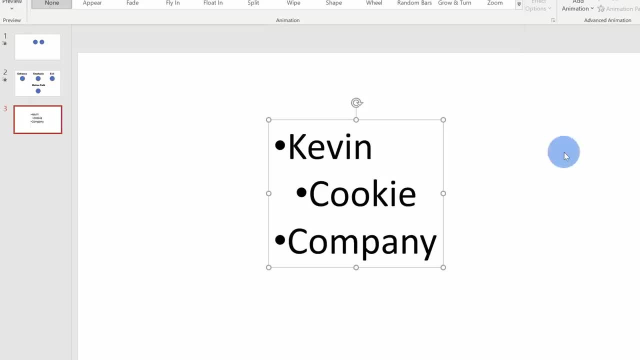 of these animations have a letter in it. These are text only animations. If I go back to the first slide and I click on animations here, you'll see that they're all grayed out because this is an object. it's not text. 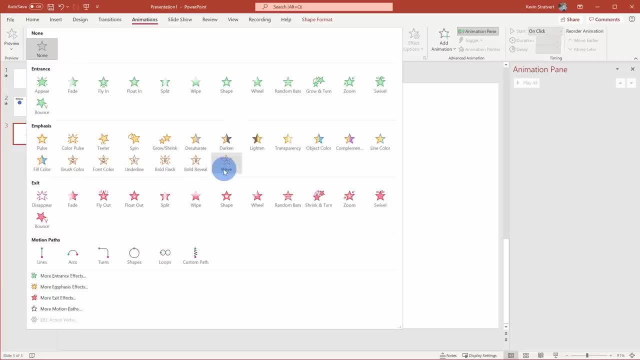 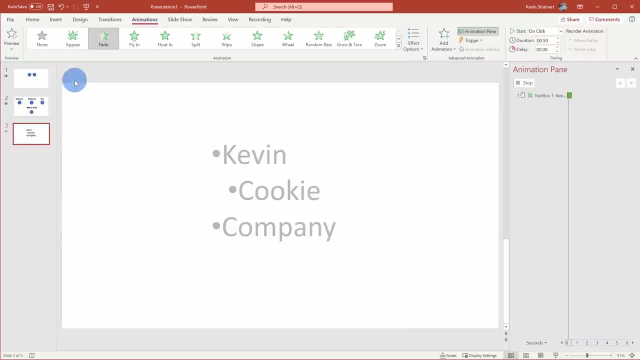 So I can apply specific animations just to text. So here I could do a wave, a bold reveal, And there are different animations I can apply. Now let's say I want my text to, let's say, fade in. Here I'll click on the fade animation and here you see that it all fades in together. 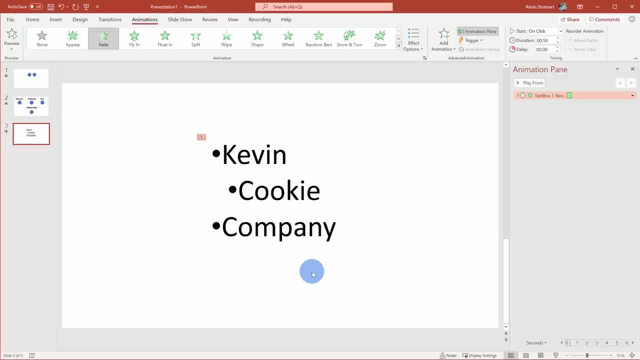 Now, frequently, when you're, say, presenting a PowerPoint presentation, you might have a whole bunch of bullet points and you want them to animate in separately. Or maybe you want your top level bullet to come in and then you want your second level bullet to come in. 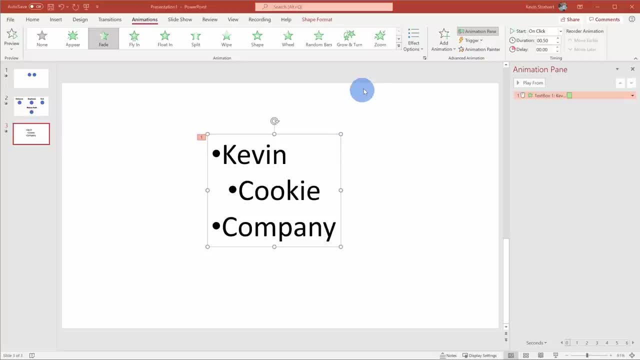 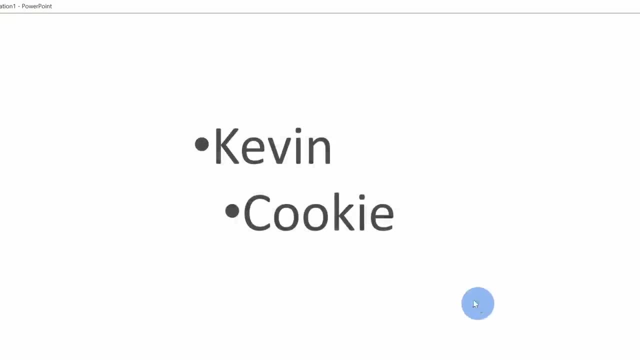 We can adjust that. To adjust this I can go up to the top ribbon and here under effect options I can change it's in by paragraph. So here I'll throw it into presentation mode and we see the first paragraph comes in with its sub bullets and then the last one comes in. 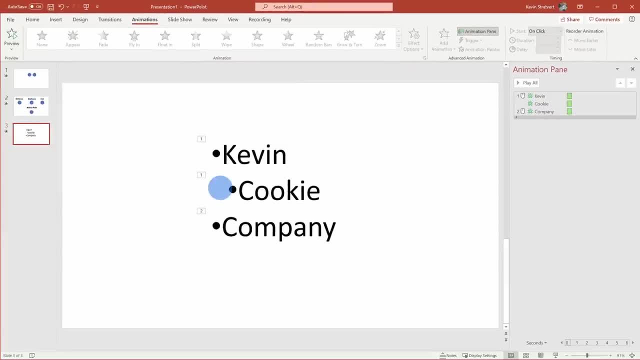 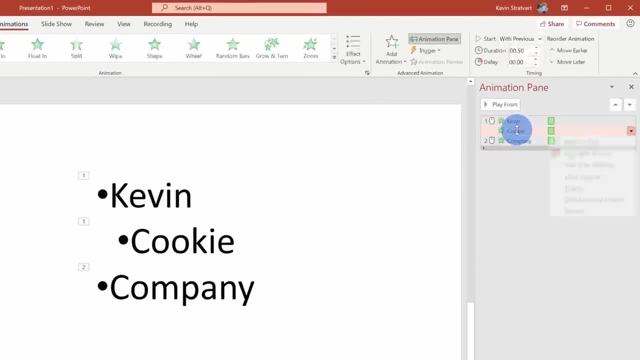 So that's exactly how I want it to look, But let's say that maybe I want cookie to come in on its own as well. Now, once again, we can go to the animation pane, and here you see that it's coming in with the previous. 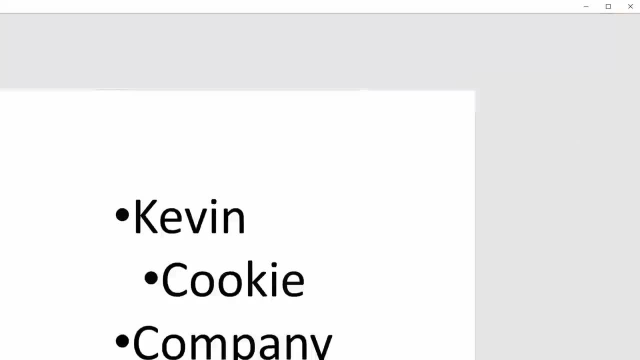 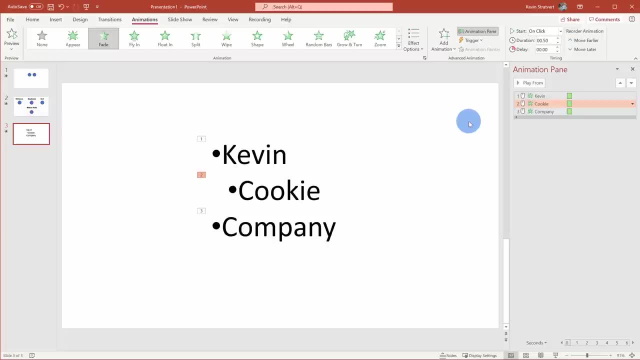 Now I could right click on this and I could have it come in on click. So now in presentation mode the first bullet comes in, then the second and then the third. So each one now comes in separately. Now it's a little bit of a pain. 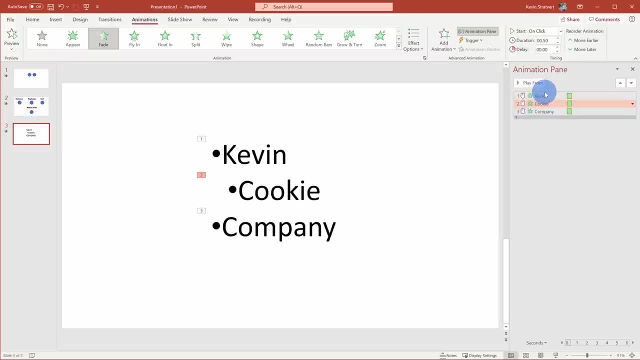 Add the animation and let's say you want all sub bullets coming in on their own. It's a pain to come into the animation pane and then bring each one in on click. You can also change it in bulk Right up here by effect options. there's this icon right here which will show additional. 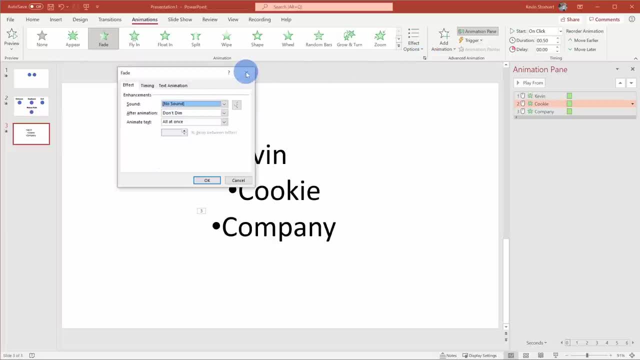 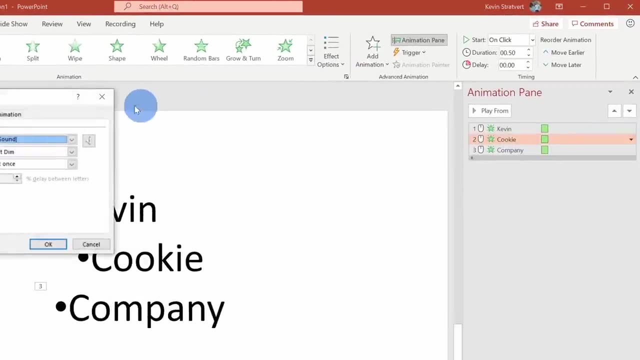 effect options. When I click on this, this opens that same prompt that we saw before. So PowerPoint offers a bunch of different ways to access this. You can come over here and here you could click into effect options, or right here on the ribbon. 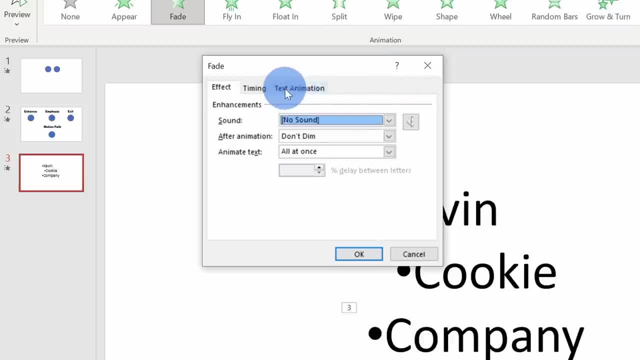 You can also access your effect options Within the effect options over on text animation. right here we can see how this animation is working and right now it's set to animate by the first level paragraphs. So first level is basically the first bullet point. 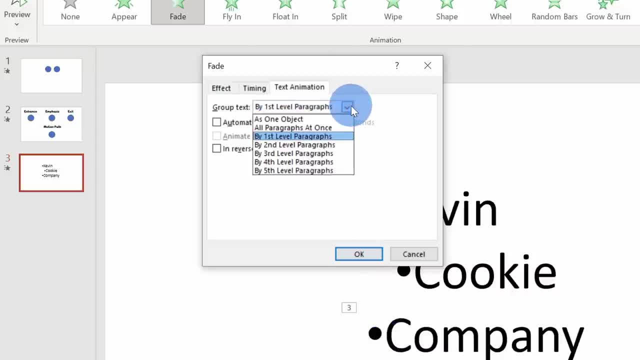 If I wanted to in bulk animate all of the different sub paragraphs as well, here I could go to second level, third level, all the way down to the fifth level. So here, if I choose by second level animation, I'll select that and then click on OK. 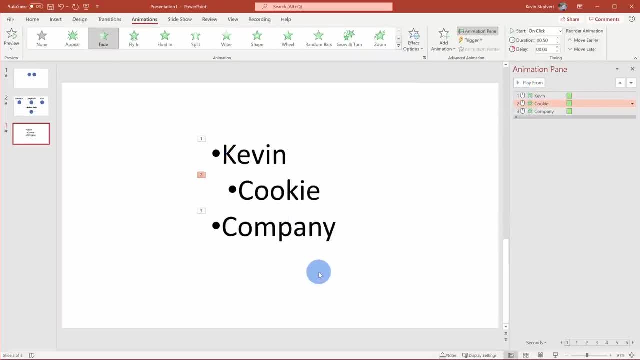 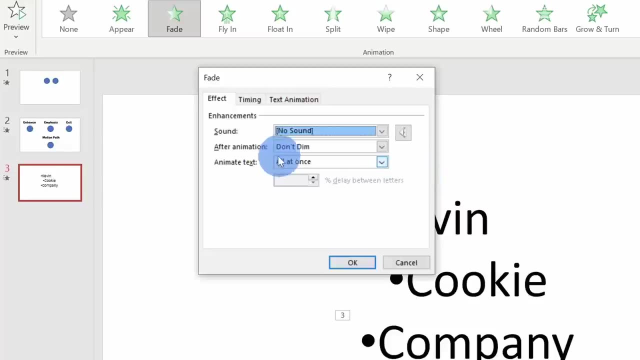 And here It's automatically done on click for all the different options With text as well. there are some other options. If we go up here and we look at all of the different effect options, you have other things like animating your text. 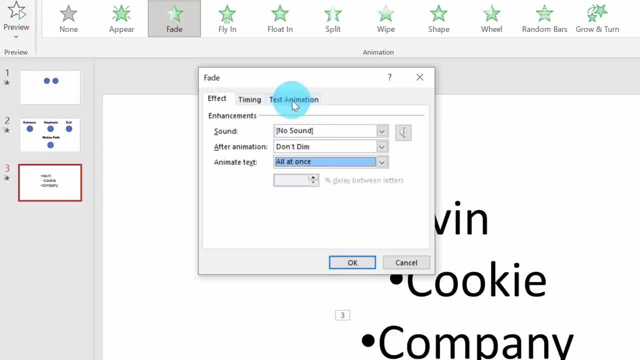 Is it animated all at once? Is it by word? Is it by letter? Also over here in text animation, you can have your sub bullets come in after a certain amount of time, or you could even have them run in reverse order. So you have a ton of power when it comes to animating different objects. 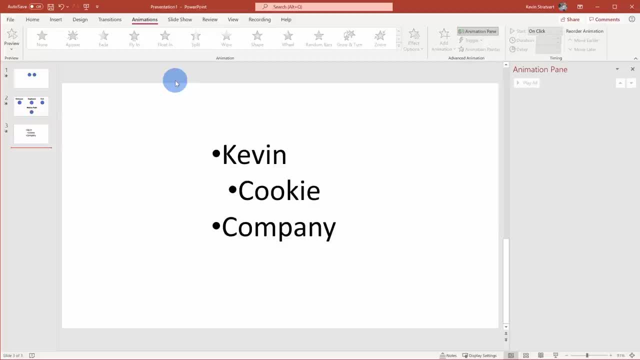 So far, I'm looking at all of the different fundamental tools that you have available to you to pull together some pretty incredible animations. And next I want to bring this all together and let's pull together our very own cool animation Over on the side. let's click in and add another slide. 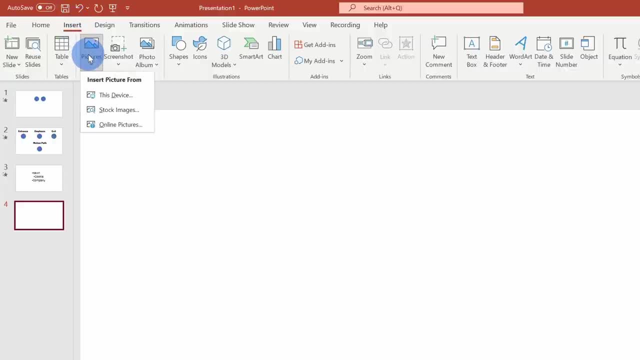 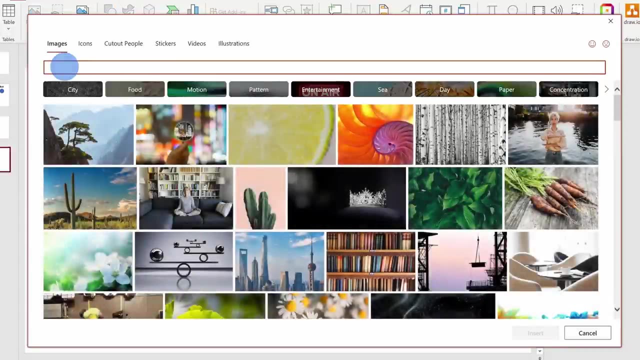 Once you add your new slide, let's go up to the ribbon and click on insert, And I'm going to click on pictures and I'll go to stock images. If you don't have access to stock images, maybe you have an older version of PowerPoint. 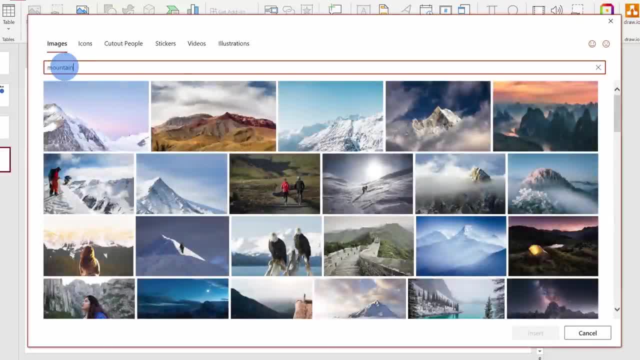 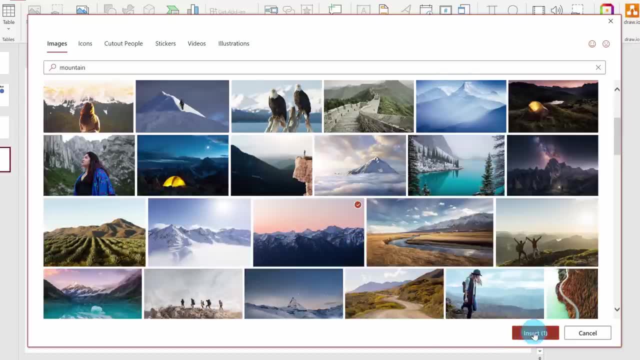 you can also find a picture of a mountain. Here I'll type in mountain and here it pulls up a ton of different photos And I'm going to use this photo of a mountain and then insert it into my slide. So I have a photo of a mountain. 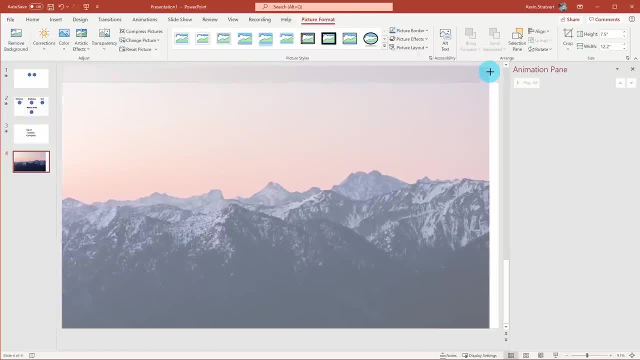 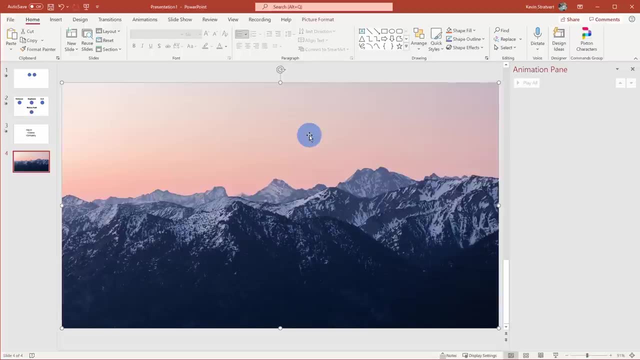 I also want to adjust it so it uses up the full dimensions of the slide Here. I'll simply pull it up and then I'll crop off the top. Once I set the dimensions of my picture to match the slide, I'm going to click on this. 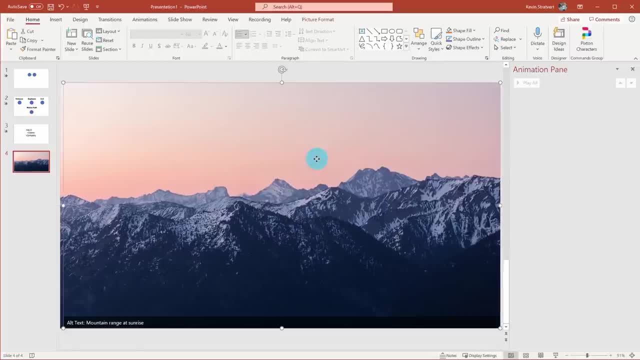 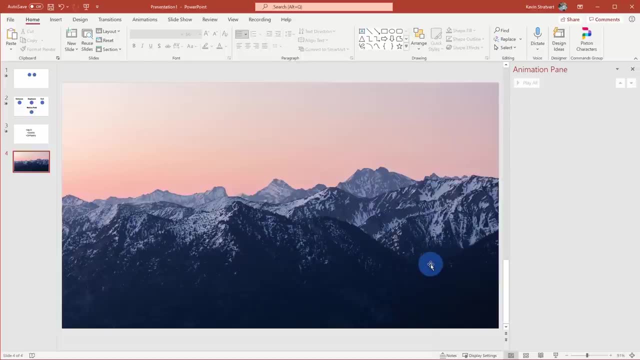 photo I'll copy and then I'll paste it. So now I have two copies of this photo and they align exactly. Next, I want to remove the background- The background- from the top layer photo. To do that I'll click on the photo and right here on the ribbon I have picture format. 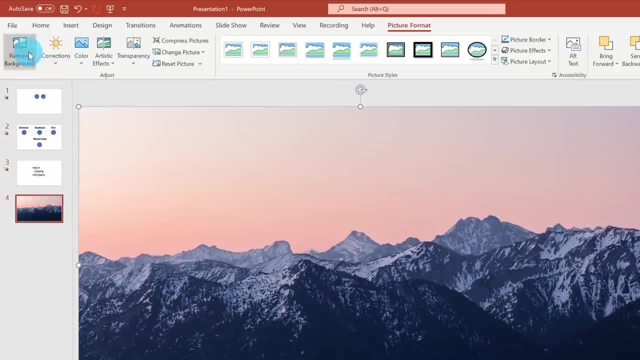 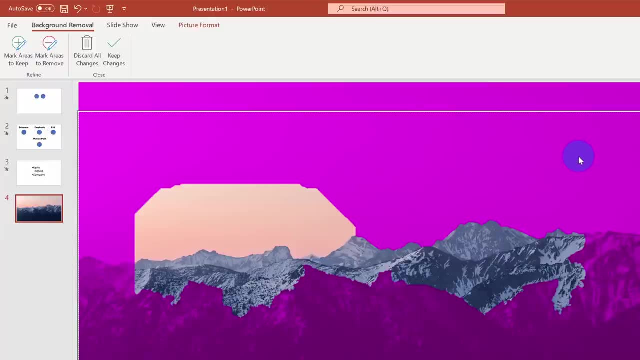 When I click on this all the way over on the left hand side, I can remove the background. I'll click on that Here now. I see my photo and all the magenta area will automatically be removed and the part that's not magenta will be kept. 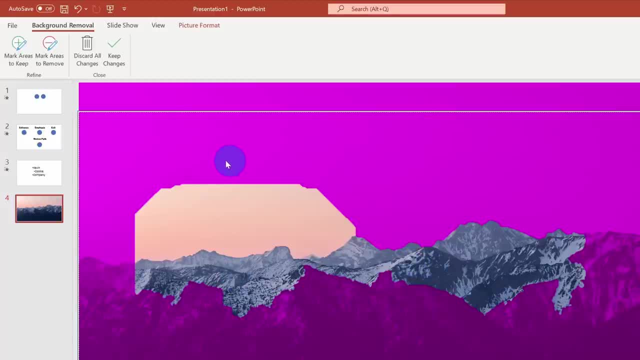 Now I want to keep the mountains on the bottom, but I want to remove the sky. So right here I'll click on this, mark areas to remove and then I'll highlight the sky. Now the entire sky is magenta, but I still have magenta down here in the mountains. 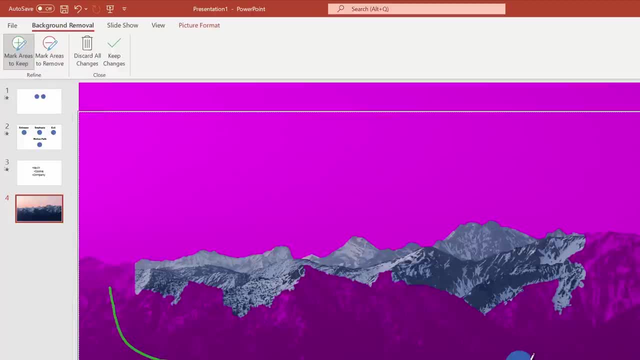 So I'll click on keep, I'll click on this, mark areas to keep and then I'll highlight the mountains over here. So I still have a few more areas to highlight and I'll go through and keep highlighting these mountains until it keeps this entire area. 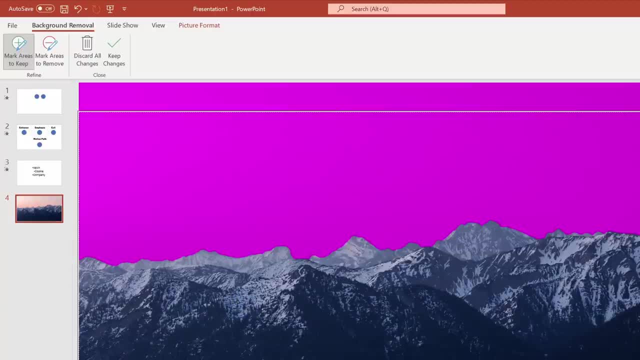 So now I have the sky that's going to be removed, and I have all of the mountains. This all looks pretty good, so I'll click on keep changes. As a little tip, if you ever need to remove the background from a photo, this is a very 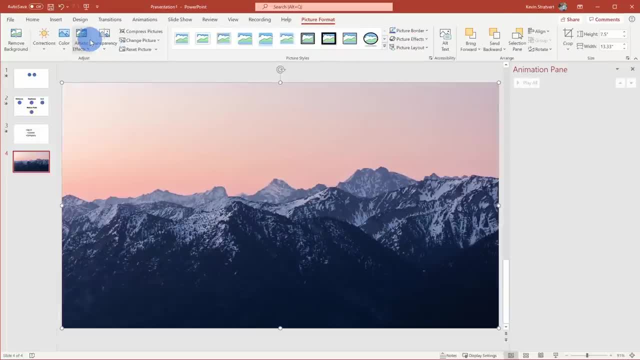 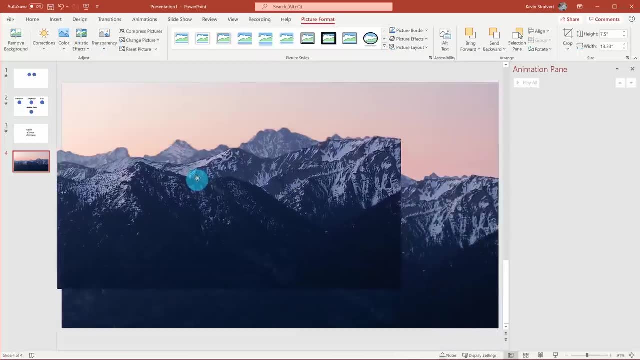 easy way to do that. Next, let's click on keep changes. Now we're back on the slide, but it looks identical to where we left off from. So what changed? Well, remember that I have two photos here. There is one photo with the sky which I've removed, and then my original photo that still 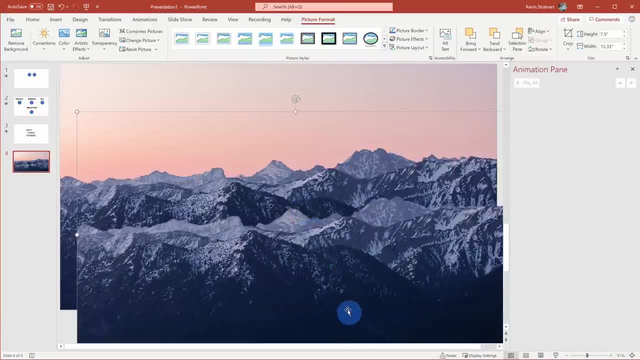 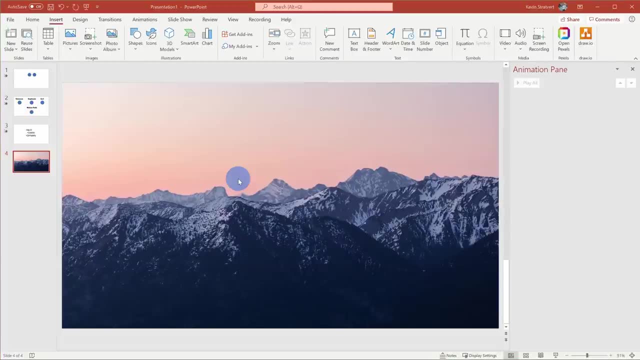 has the sky that's still there as the background. So we're going to use this to create layers and we'll use this as part of a pretty advanced and cool animation. Next, I want to insert a photo of the moon. So once again, let's go over to insert. click on pictures. 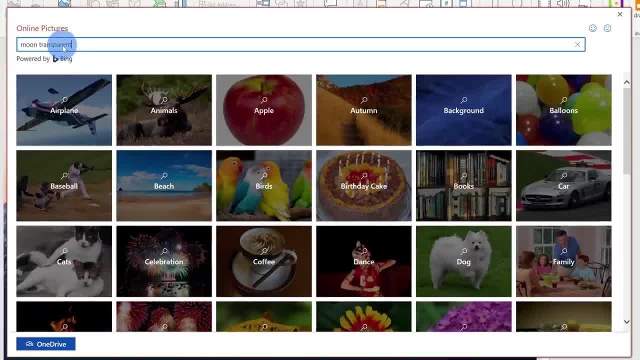 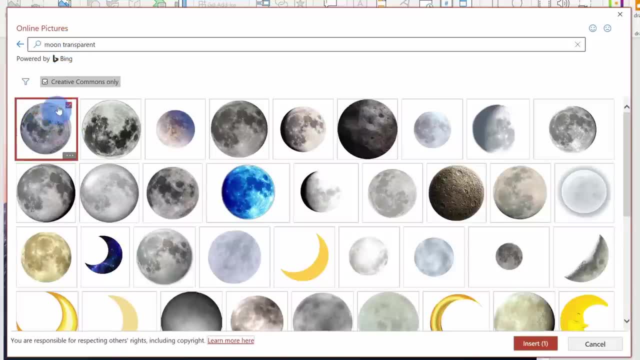 And then I'll go to online pictures. This opens up a prompt where I could search for pictures. I'll type in moon transparent By typing in transparent. this will ensure that there's no background there. Here I'll select this first image of the moon. 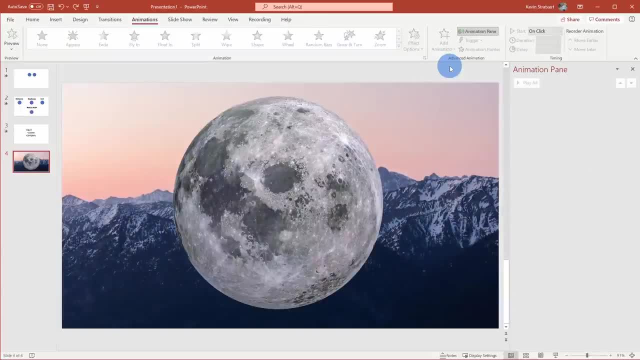 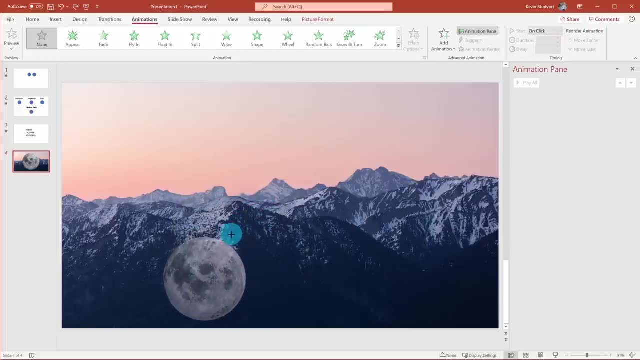 I think that looks pretty good. Then I'll click on insert. This is now inserted- a photo of the moon, and it's a little big right now, So I'll click on the moon and let's reduce the size so it looks a little bit more reasonable. 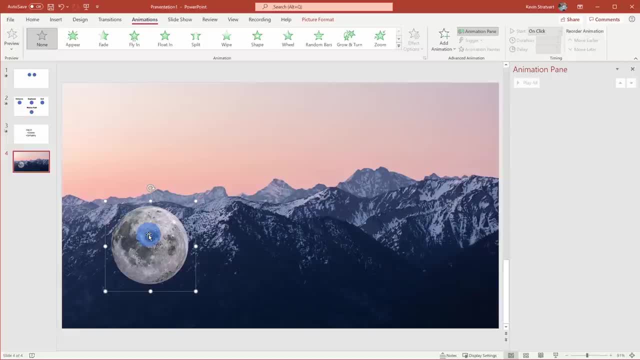 I'll place it over here, and right now it's in front of the mountain, and we'll leave it there for now, But coming up later We'll adjust the layers of this. Now I want to apply an animation to this moon, So I'm going to go up to my animations over here and let's click on this dropdown. 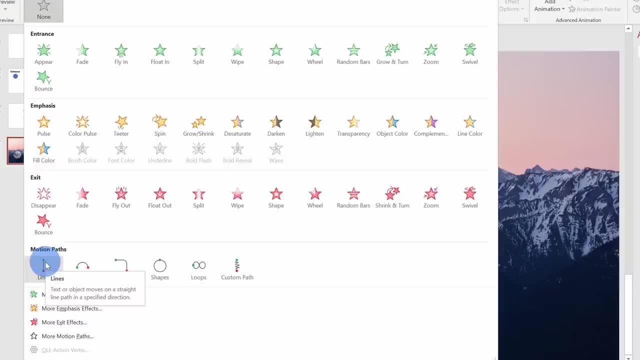 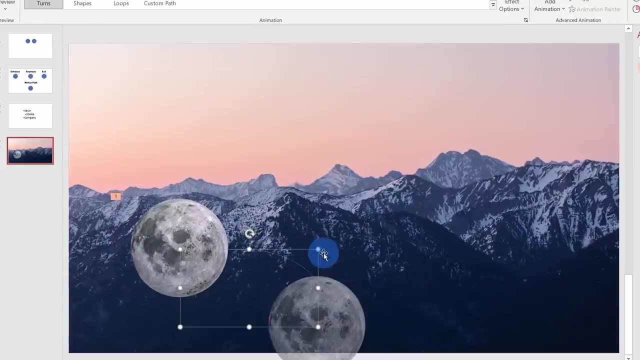 Right here there's a category for motion paths and I want it to lift up and then turn over the sky, So I'll go with this one that says turns. When I select that, you see that by default it goes to the right and then it turns down. 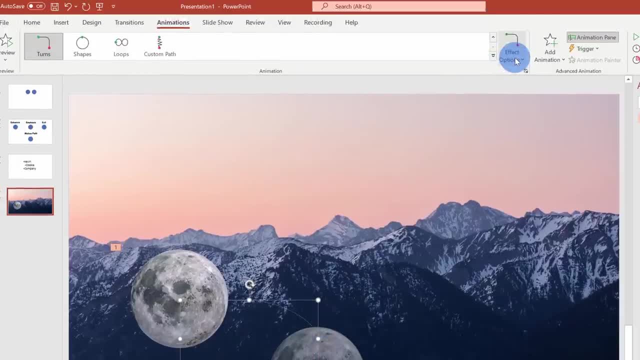 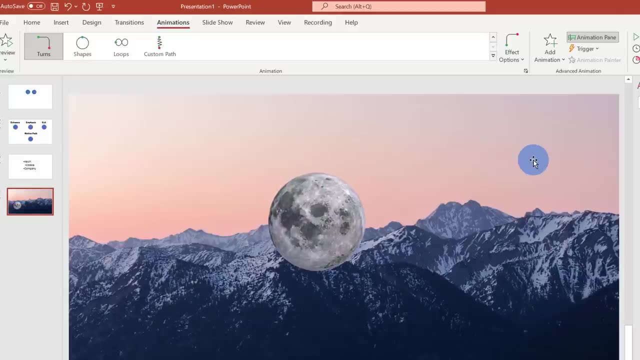 I want it to turn up. So let's go over here under effect options, just like we looked at earlier, And there's an option to go up and to the right. Select this option Now. from the preview you saw that the moon goes up and it moves to the right, but then 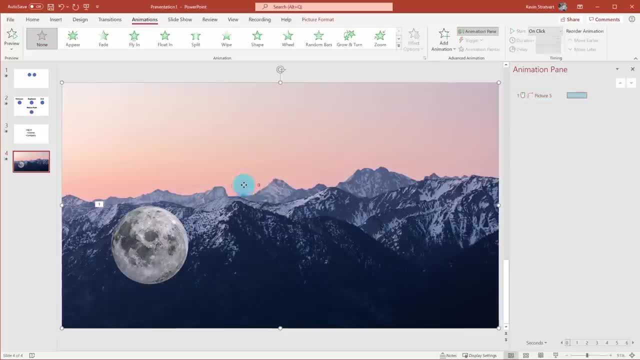 it stops right here, So it doesn't go up that far. Now I can click over here on the path and here I see the size of the path and I see the end position. I'm going to adjust this and let me expand this out. 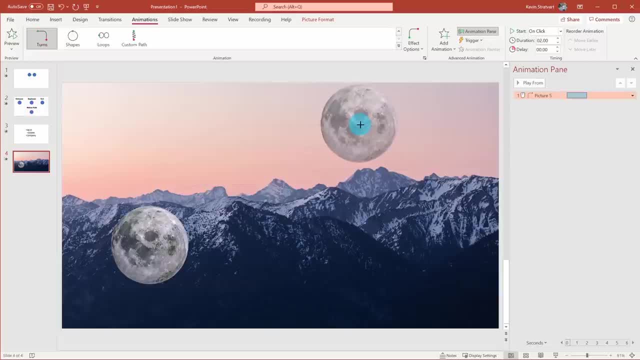 Here you'll see, as I'm expanding it out, the motion path is also expanding, So I want the moon to stop right about here in the sky. So here I see the full path and I'll click away If I click on preview. 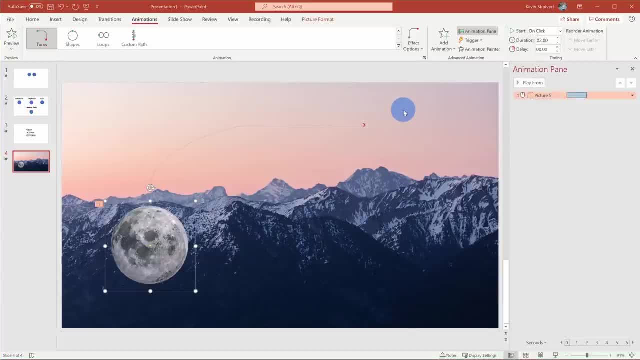 Now I can see the moon lift and then go over From the preview. the moon is lifting up and going over fairly fast, and I want it to go a little bit slower. Now, once again, we could adjust the duration Over here in the animation pane. I could select this and then I could drag it over. so it goes. 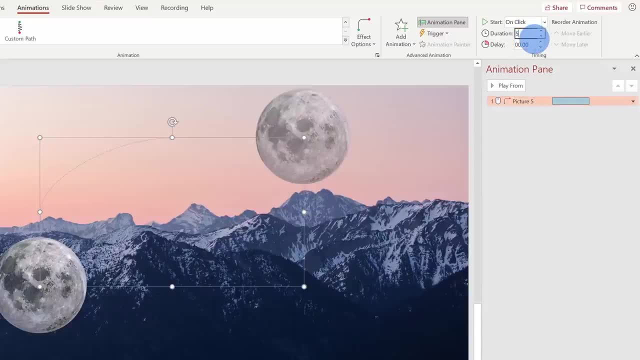 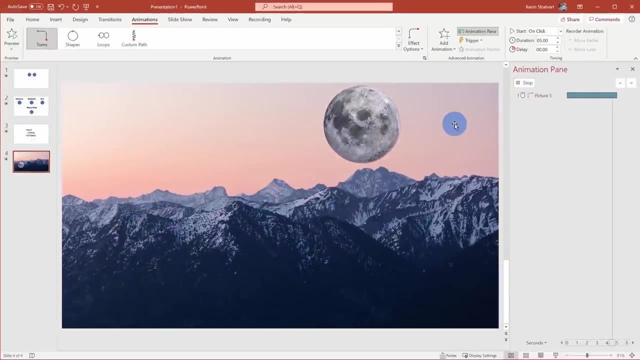 on a little bit longer. Alternatively, I could also click up here, and maybe I want it to go on for about five seconds. Now, if I click on this play icon, you'll notice the moon lifts up in the sky and it moves a little bit slower. 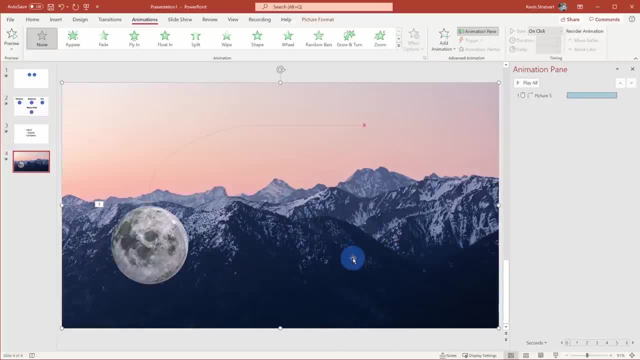 So I think that looks pretty good. Next, I want this mountain range right here, So the topmost layer. I want this to also bulge out or come out. I think that'll be a neat effect With the mountain selected. I'll go up here to my animations and over here let's say: 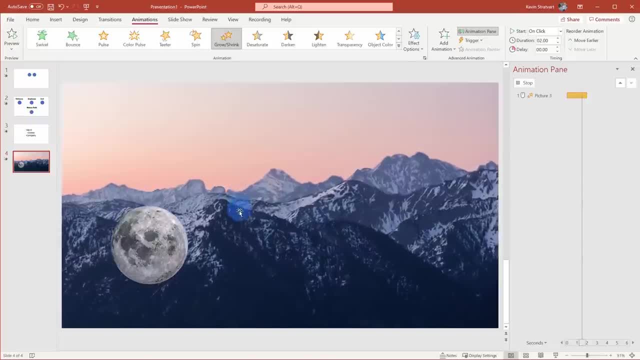 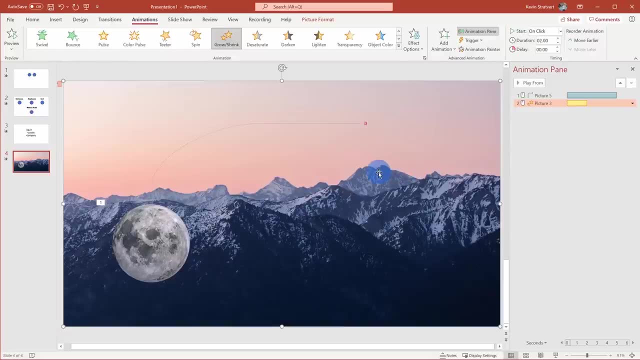 maybe we go with the grow and shrink, So I'll select this one and we see the mountain come out a little bit, and what's neat is you also have these other mountains slightly in the background, So it adds a little bit of depth. Now I have these two animations set, but I want to move the moon behind this mountain. 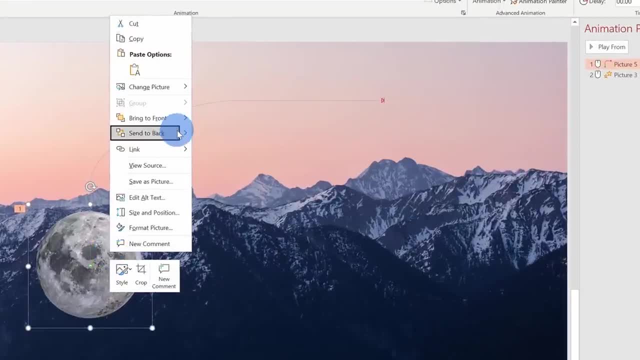 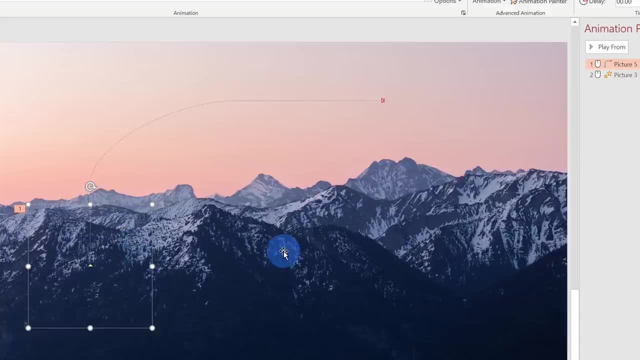 range in front. So here I'll select the moon, right click, and then I'll go to this option that says send to back. but I don't want to send it all the way back, So I'll simply send it backward. So right now it's sitting behind this first mountain and here I could pull it down and 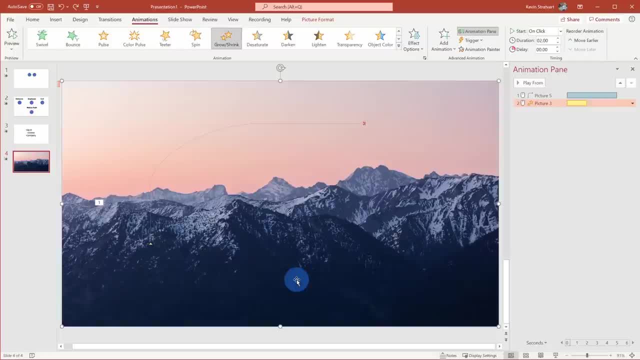 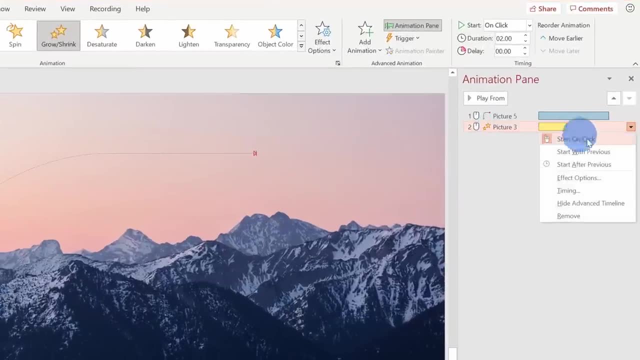 there, you see it sitting right there. I want both of these animations to occur at the same time. So over in the animation pane for the mountain range, I'm going to right click on this and I'll have it start with the previous one. 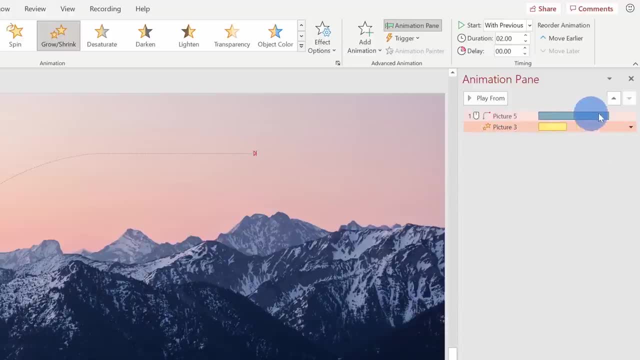 So here they'll both go on at the same time. Now you'll see that- the moon animation and the mountain animation. They don't last as long, so I want the duration to be the same. I'll select this and then I'll set it to five seconds. 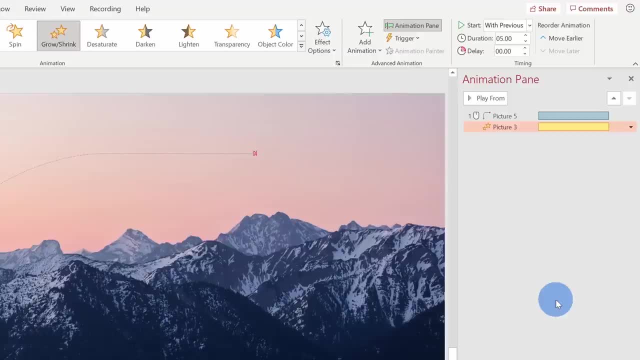 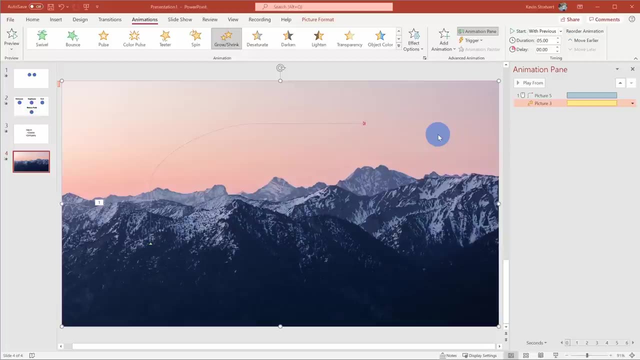 So this way, both animations occur over the same time period. This animation is starting to come together pretty nicely, but before we play the final animation, I do want to add a little bit more depth to this animation. I want the mountains that are in back to sit a little bit above these other mountains, just. 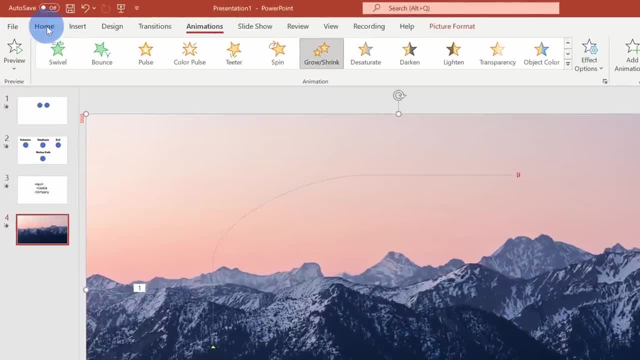 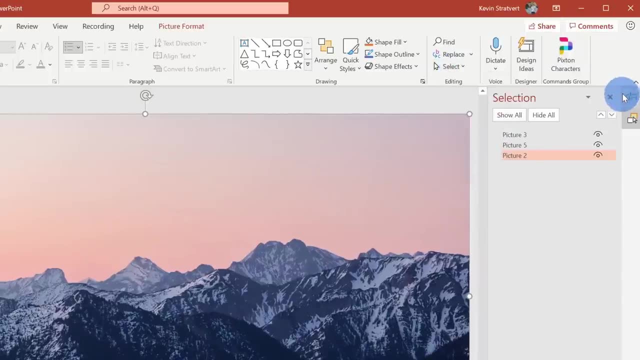 to add that depth. To do that up on the top ribbon, let's click on home and then go over and click on select. We're going to launch the selection pane. I'll click on that Here. you'll notice, on the right hand side I can toggle back and forth between the animation. 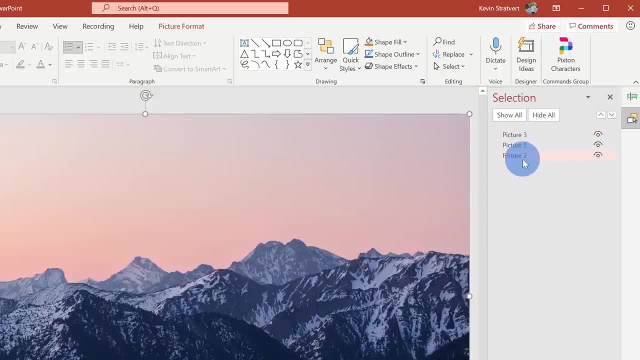 pane and the selection pane. Now my bottom, most layer is sitting right down here. It's picture two Here I can show and I can hide it. So this is my mountain with the sky. I'm going to select picture two by clicking on it in the selection pane. 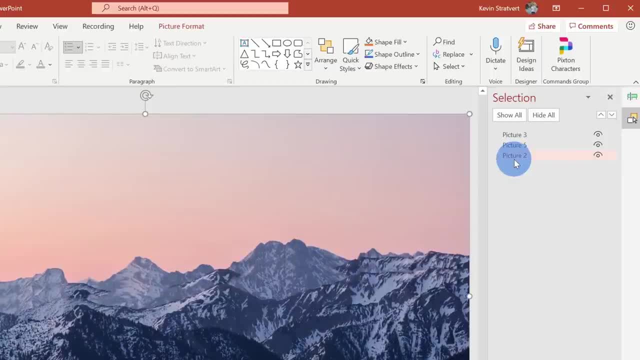 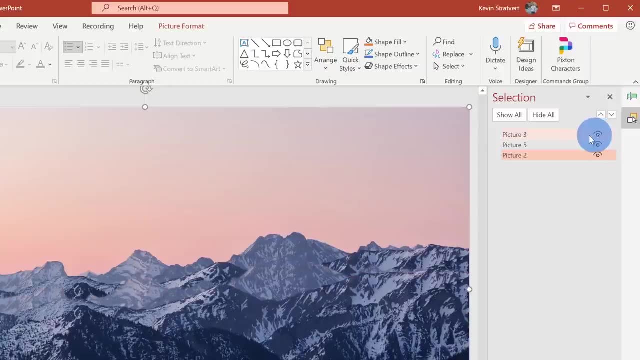 Then I'm going to hit my keyboard up arrow just to pull it a little bit higher, just so it's not sitting at the exact same point as the other mountain which is sitting on top, My previous mountain. So right now, picture three is the top most mountain. 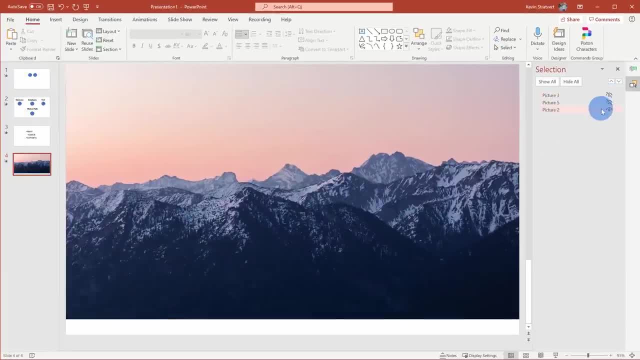 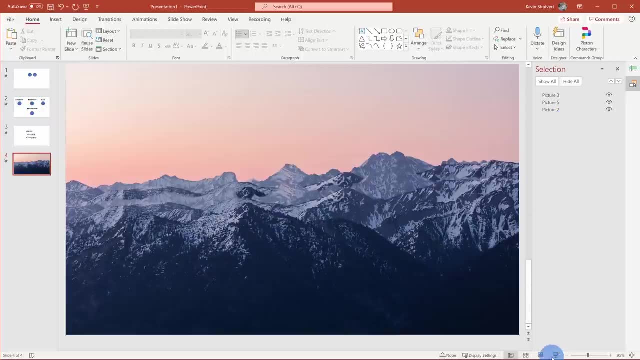 If I hide that, you see the moon, and then right down here I have my bottom, most layer. So these are my three layers, So that all looks pretty good right now. I'm now all set to play my animation, So let's click on presentation mode and here, if we click on play now, you'll see the mountain. 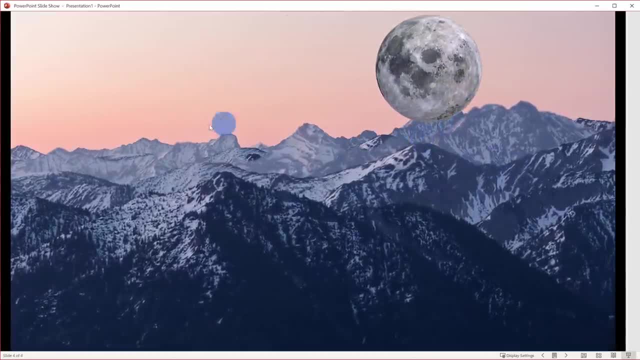 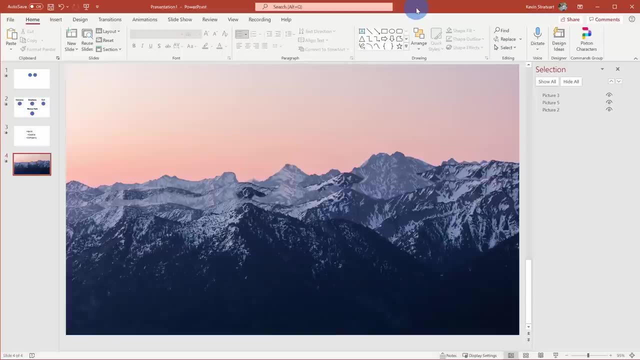 come out, You see the moon go up and you see a little bit of depth with this other image in back. So with PowerPoint animations you can pull off some pretty incredible effects. Now I don't have all of the fundamental tools to animate in PowerPoint, but PowerPoint offers. 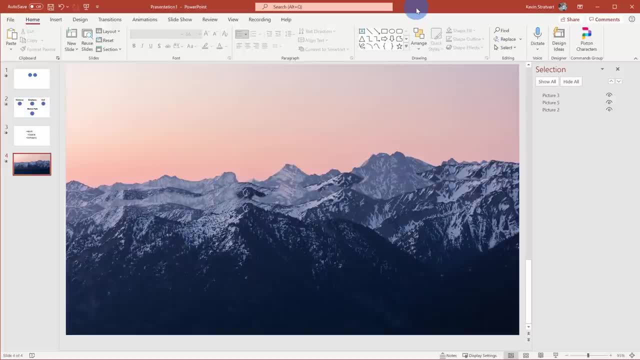 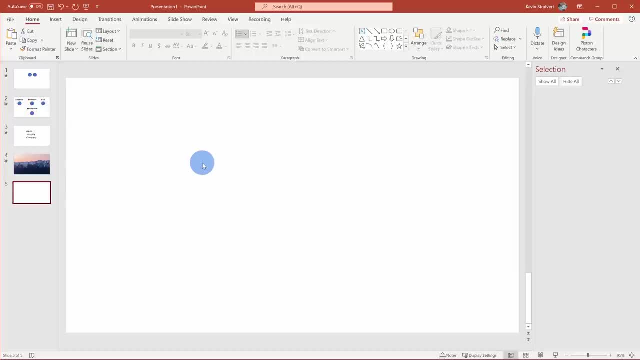 even more. It's such a rich program and there's so much functionality. Once again, over on the left hand side, let's insert another slide and I want to show you how you can use the morph transition to also add animations to your deck. 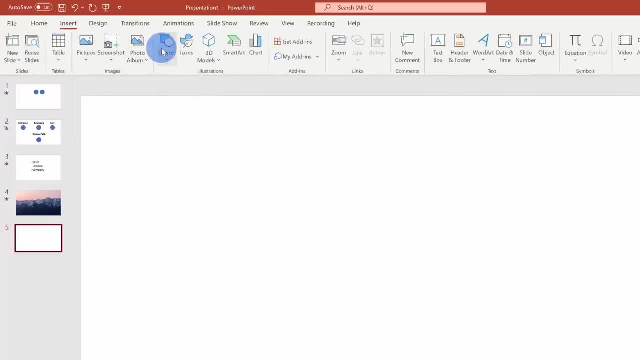 Let's go up to the top ribbon and click on insert. Once again, let's go over to shapes and this time let's insert a rectangle. I'm going to draw a rectangle right here in the top left hand corner. Let's go down and take slide five. 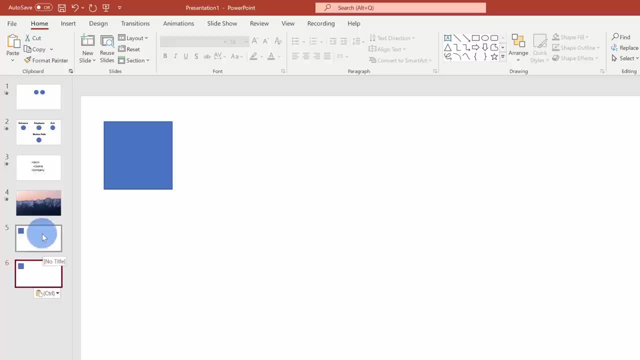 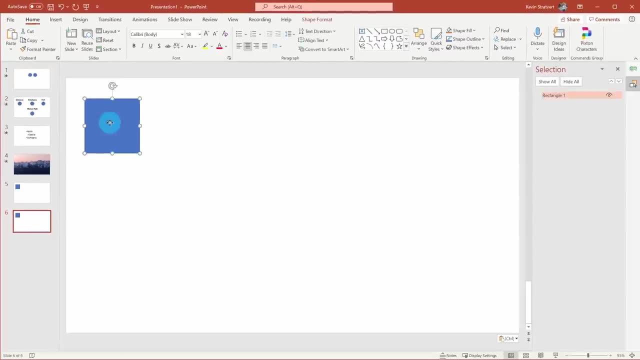 I'm going to copy it and paste it. So you should now have an identical slide. so you have two identical slides. On the second slide of the two identical ones, take the shape that you inserted and move it to a new position, and you can even try adjusting the size. 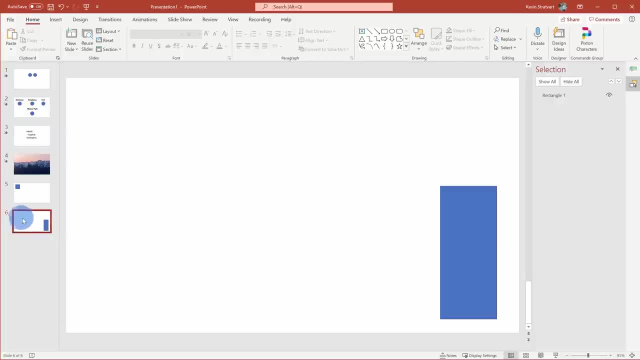 So here I'll make it a little bit bigger and maybe a little bit longer. Now, with the last or the second slide selected, let's go up to transitions and then click on morph, Right here you'll see it animate or morph from one shape to the other. 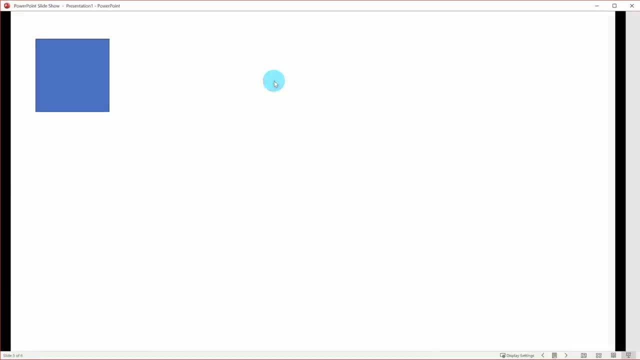 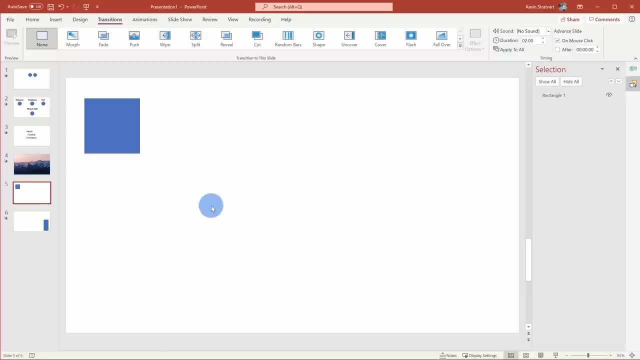 So here I'll click on the presentation mode and when I play it here, you'll see it go from that rectangle to another sized rectangle in another position. So this is one more way you can add animations to your slides. Now I also want to show you how you can pull off an advanced morph. 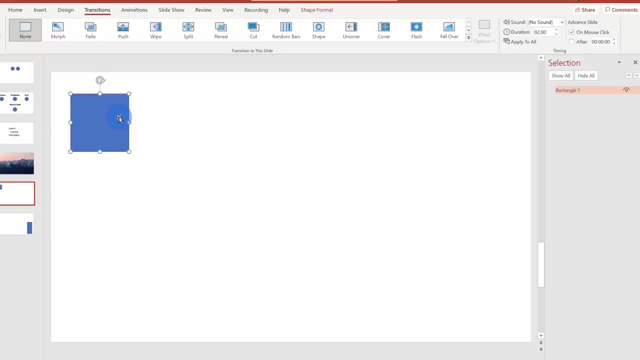 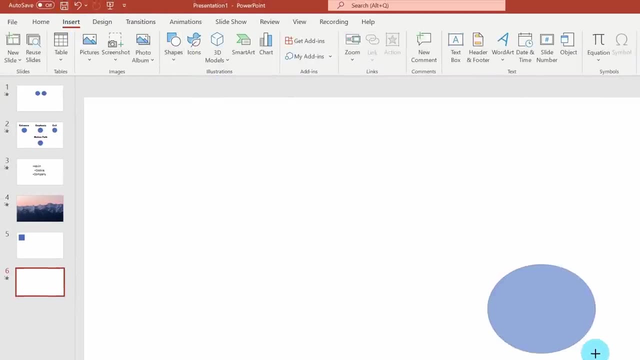 So say, you want to take this rectangle and you want to morph it into, let's say, an oval, Right here. I'll delete this shape for now and let's go up to insert. I'll go to shapes and let's insert in an oval. 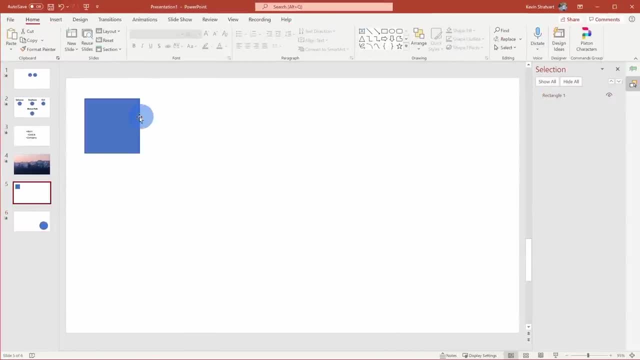 So here I'll just draw it in the bottom right hand corner. So I'm going to take this rectangle and I'm going to move it over here and I'm going to move it to this corner And I want this shape to morph into the other one. 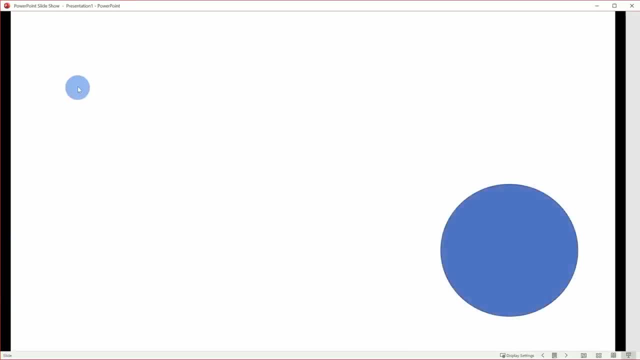 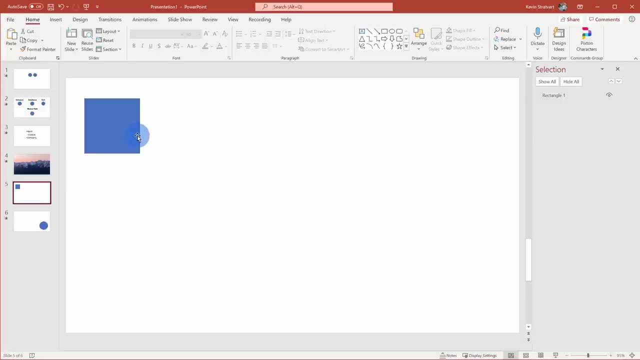 So I still have the morph transition. The trouble is, when I hit to the next slide, it simply fades out, and then this one fades in. I want this shape to morph into this shape, So we need to make sure that the names of these shapes are identical. 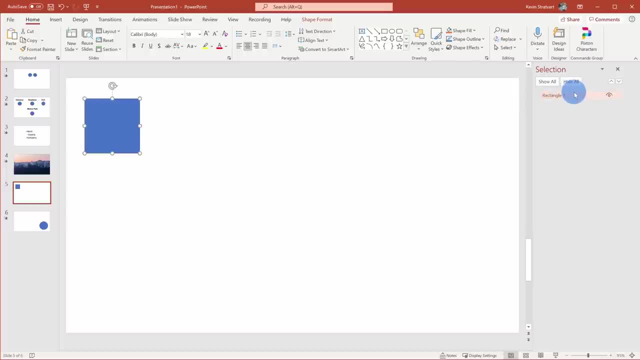 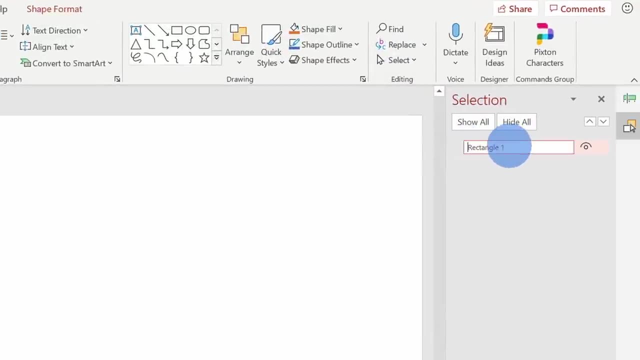 Here I'll click on this shape, and I still have my selection pane open. But if you don't have it open anymore, you can click on home and then click over on select and selection pane, And here this is referred to as rectangle one. 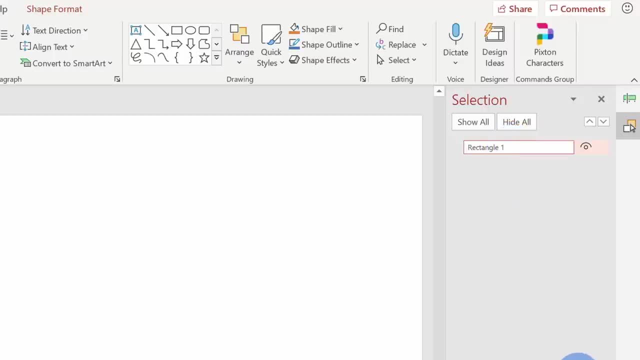 So I'll just leave that name for now. To pull off an advanced morph, we have to insert two exclamation marks at the beginning, So I'll put two in front of this, and let me actually just highlight this entire name. copy it, and then I'll go to the next slide. click on this shape, and here I'll double. 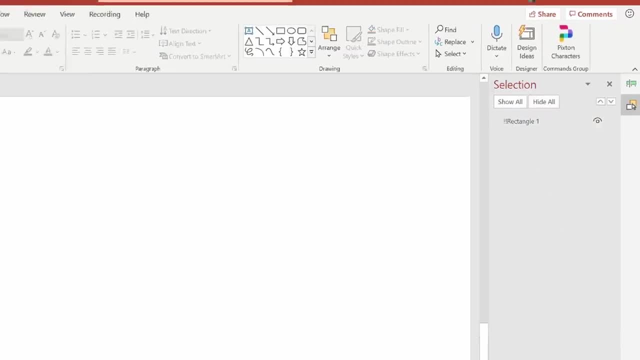 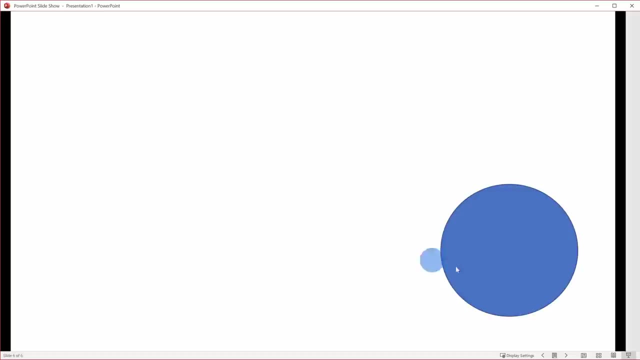 click in and I'll paste it in. So now they have the exact same name. So if I go back to slide five, I'll jump in the presentation mode. and now look at that animation. It morphs from one shape into the other. 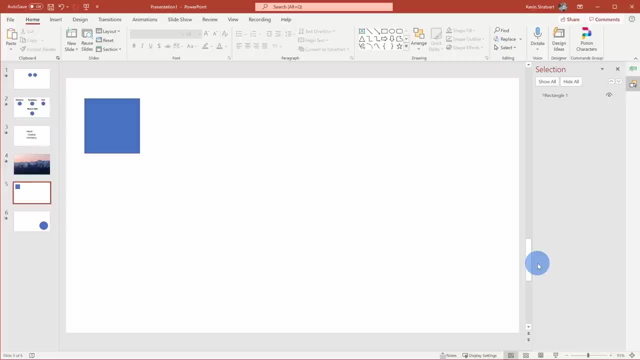 So this is another way that you can add some very impressive animations to your slide presentation. Lastly, I also want to show you how you can animate 3D objects in your presentation, And this is the last bit in terms of animations in PowerPoint. 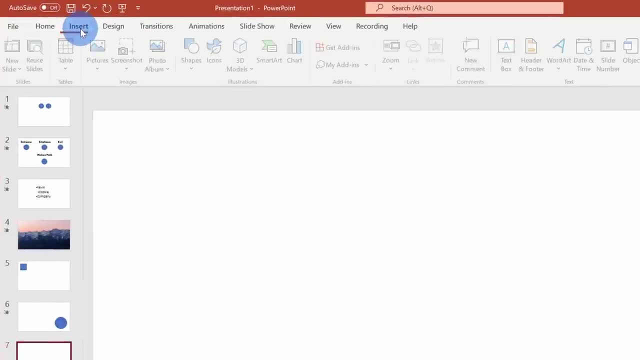 Once again. let's go over to the left and add another slide Up here. I'll click on insert and let's go over and click on 3D models. Now you could build your own 3D model and I recently did a tutorial of how you could. 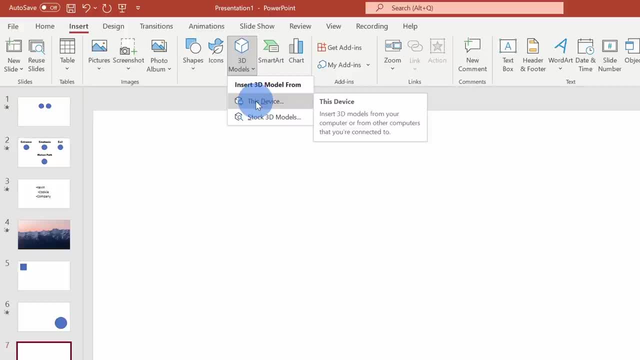 use Paint 3D. If you follow that, you can build your own models and you can then bring them into Microsoft PowerPoint. I'll put a link in the description of this one. For now, just to keep things simple, I'll go with one of the stock 3D models. 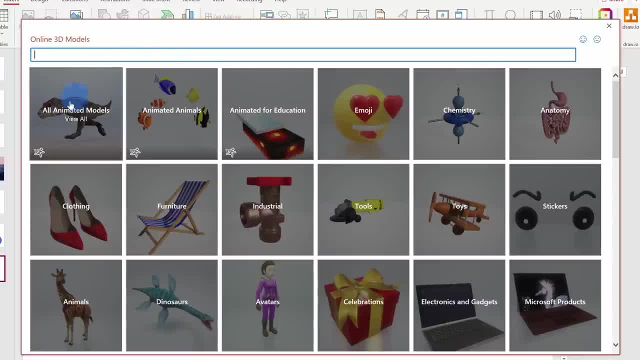 This opens up online 3D models, and right here at the top you'll see that there are all of these animated models. So here I can view all the animated models, or you could just look at animals or education. Let's click on all animated models to see what's available. 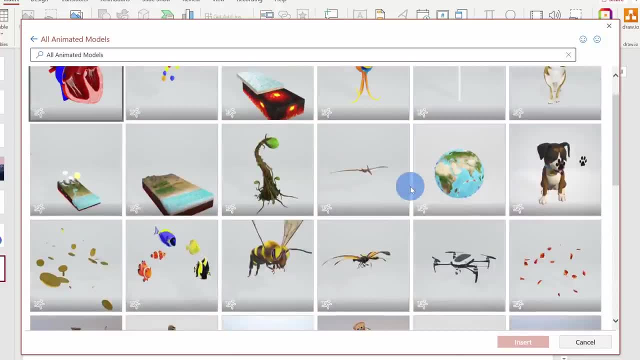 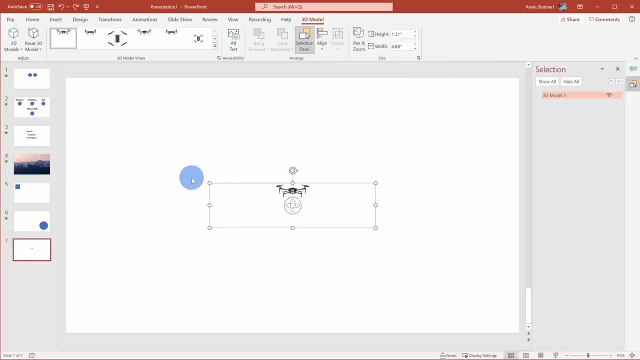 So look at this: There are a whole bunch of different models that we can choose from, And why don't I go in and I'll select this drone right here and then insert it? I've now inserted the drone And onto my slide and it's a little bit small right now. 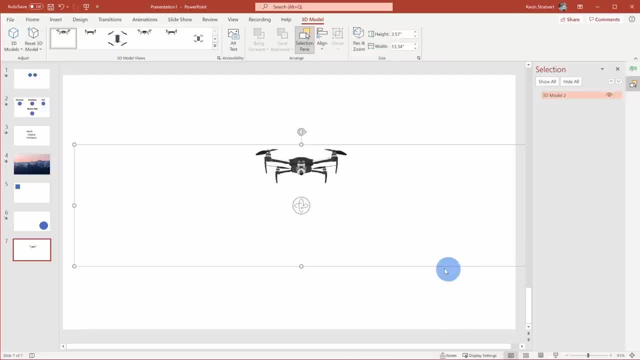 So I'll expand it just so we could see it a little bit better. So there's my drone in the center of the slide Now. right now it's on 3D model on the ribbon, but here I can go over to animations and if 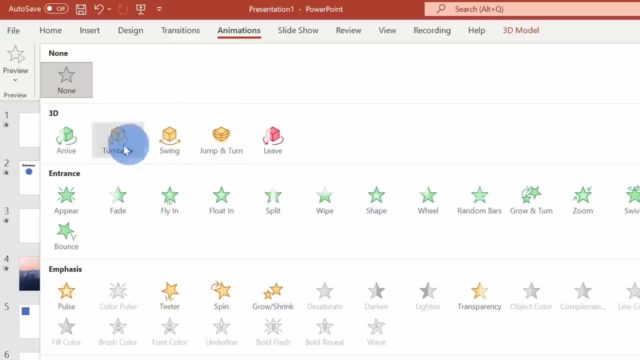 I expand all the different animations here. you'll see that there are some specific animations for 3D objects, So I could have it arrive, I could have it leave, and there are also some other animations that I could apply. Let me go with this jump and turn and let's test this one out. 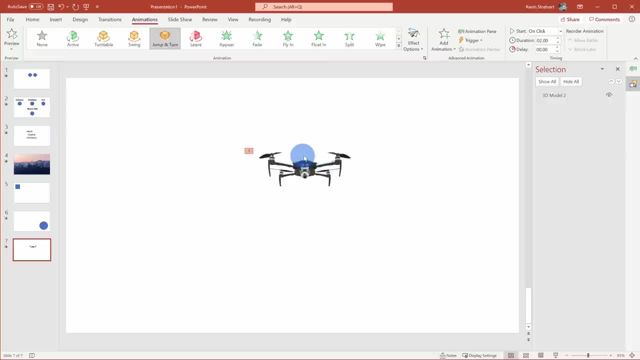 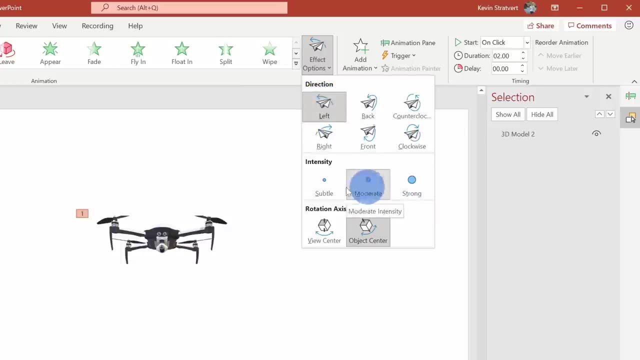 So check that out. I'm now animating a 3D object here. Also over on the right hand side. I have some effect options, So here I could decide what direction I want it to go in, Also the intensity and the rotation access. 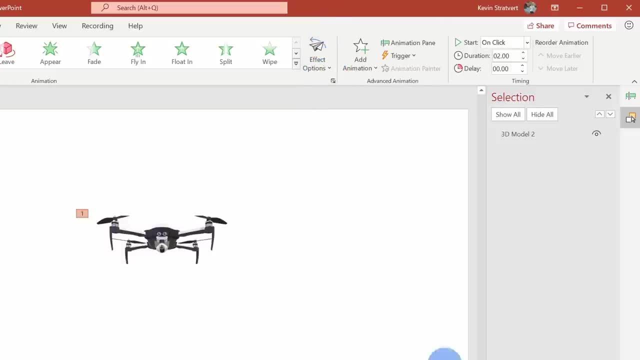 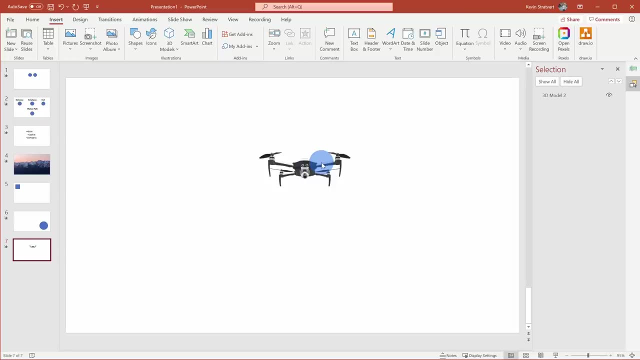 So I have a lot of similar effect options to what I had for the other animations. If I throw it into presentation mode here, if I click on it now, you'll see this cool animation to this 3D object. Next, I want to show you how you can also use a morph with a 3D object to add an additional. 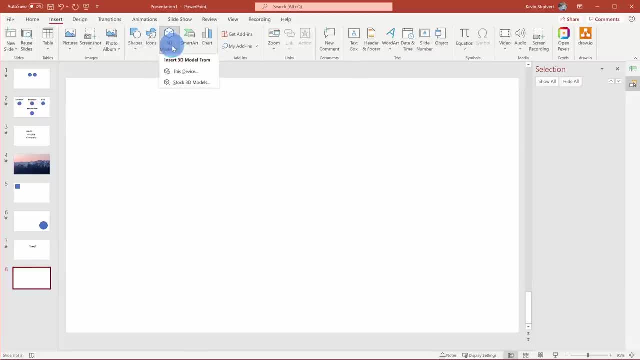 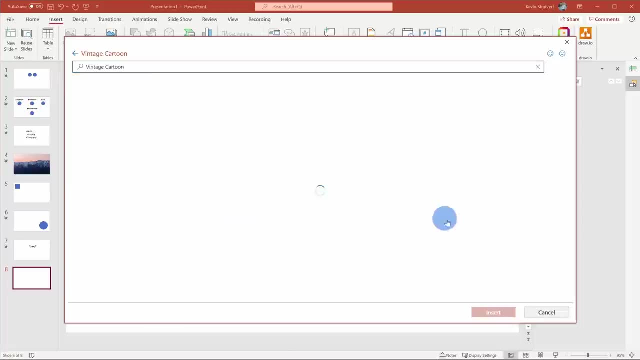 animation. I'll add another slide in my presentation. Let's go back up to 3D models and I'll go to the stock 3D model option Right here. let's select vintage cartoon. Within vintage cartoon, I'll select the car and then click on insert. 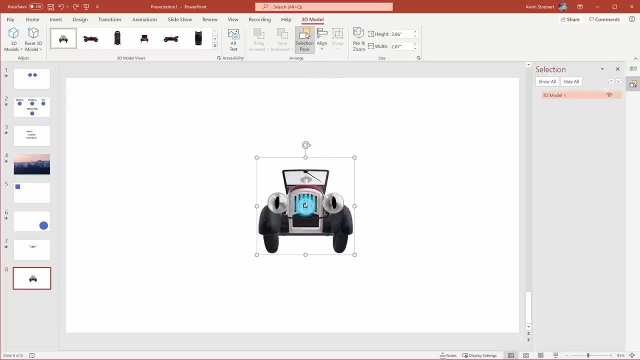 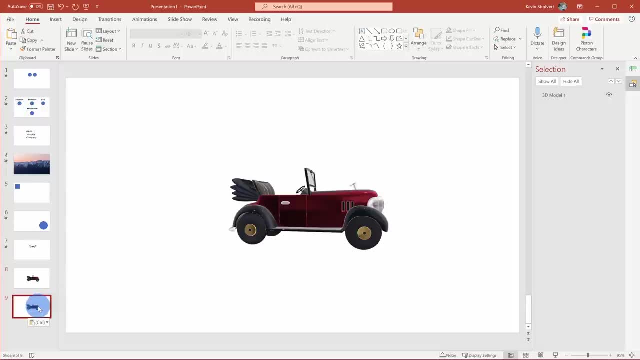 This is now inserted- the car onto my slide- and I'll adjust it a little bit so we have a side view of the car. Next, I'm going to take this slide, I'll copy it and paste it again, And this time let's use the morph transition again. 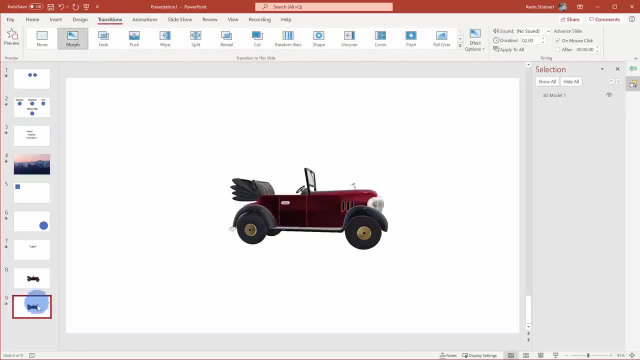 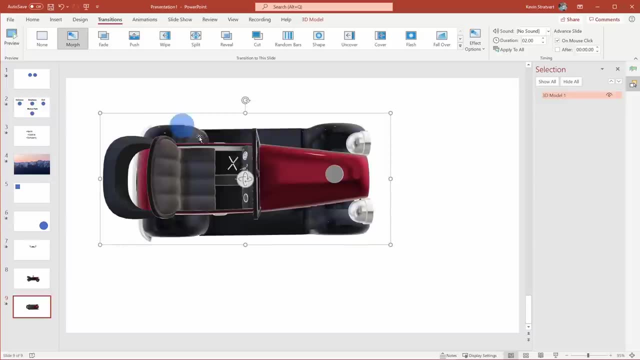 Right here Let's go to transitions and then let's click on morph And over here with the car I'm going to adjust the position. So maybe now we want to switch to a top down view and I'll also expand the car. just a.